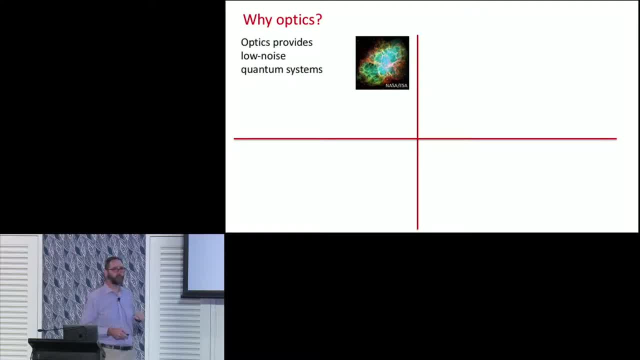 noise systems. Okay, so the light from the Crab Nebula, six and a half thousand light years away, is still very polarised when it reaches us here at Earth. Okay, so if we're able to, you know, have light and prepare it in a really clean state, then it's going. 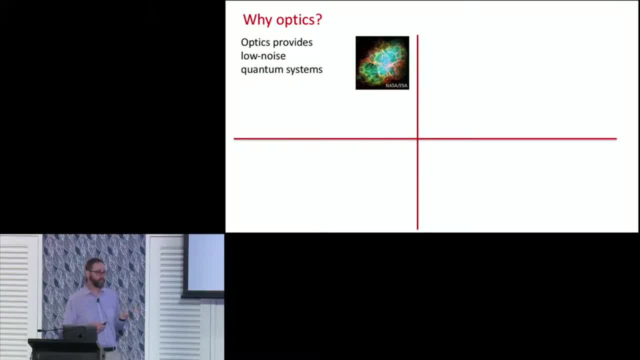 to. it doesn't interact particularly strongly in non-resonant systems, and so we can keep things very clean. Also, we're able to detect light at quantum noise- limited levels. okay, Detection is exceptionally good, and so we have a clean and flexible system. We also 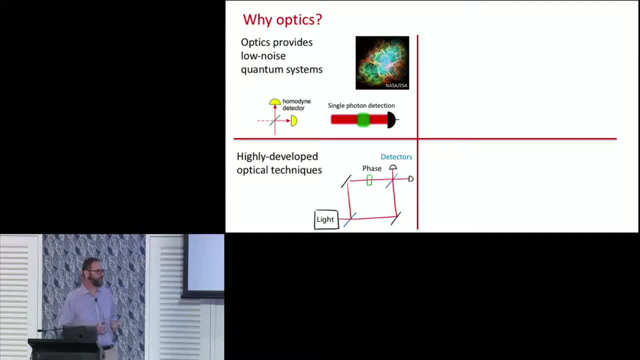 have highly developed optical techniques. We've been doing interferometry as a science community for over 150 years, similarly polarisation control, and so these kinds of classical optics techniques can be used to detect light at a very high level, and so we're able to do. 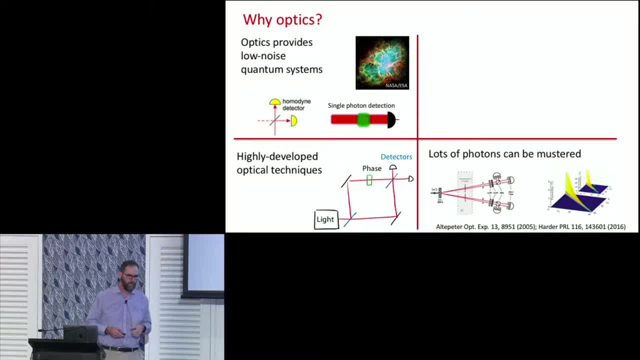 these kinds of stuff. Again, some of the information we've been using for, you know, evaluation is not going to be translated to the quantum realm as well. Also, we can muster lots of photons. okay, If photons or other optical quantum states are going to be our. 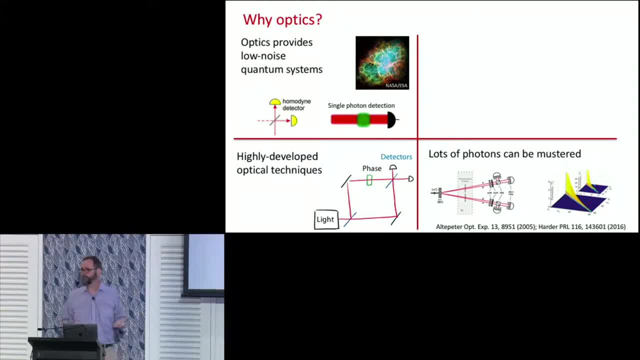 quantum systems, we actually have access to enormous numbers of them. okay, So we already have experiments where millions of photon pairs are generated, a second where they're generated in many tens at a time, including in my lab, And so the question then becomes: 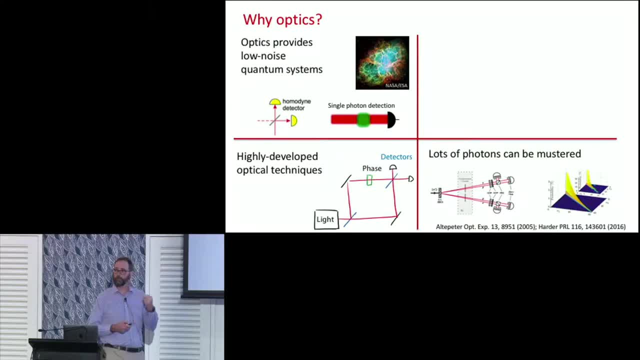 them, but how do we control them? okay, but in terms of the number of raw systems, not. not a problem. and another really attractive reason for considering optics is, of course, in the classical regime it's already a platform for networking. we already know that our world is connected up by optical fibers and we 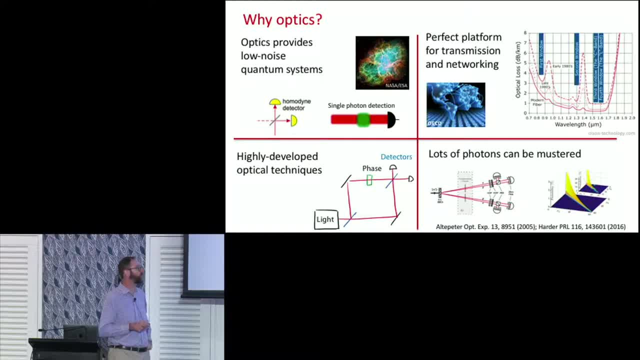 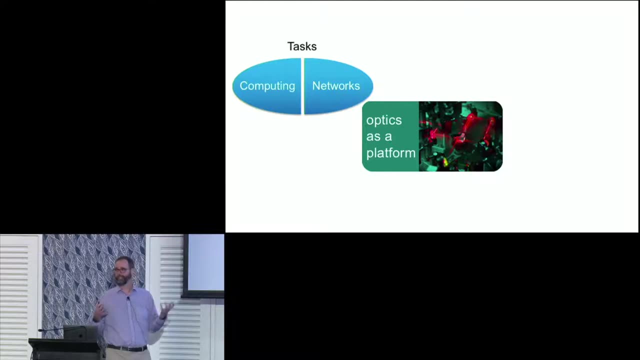 work at in this, the telecom regime through optical fibers, because losses are low, we can send signals long distances and we can communicate very, very quickly. so these are some of the reasons why we might consider optics as a quantum information platform and, of course, I've already alluded to the fact 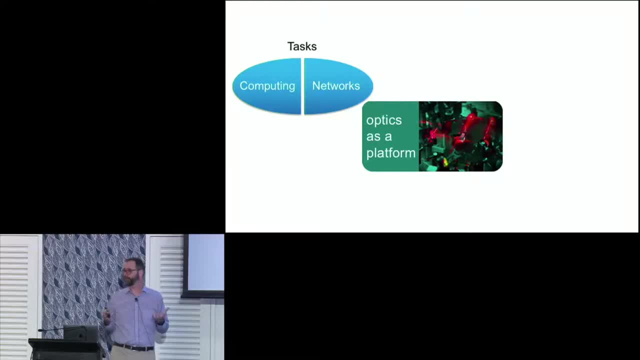 that perhaps, unlike some of the other platforms that we might talk about, there's more than just one or two tasks for using optics. so computing, quantum computing is one, but quantum networks is another one. okay, and we heard in how Wiseman's tutorial the other things like making precision measurements or doing 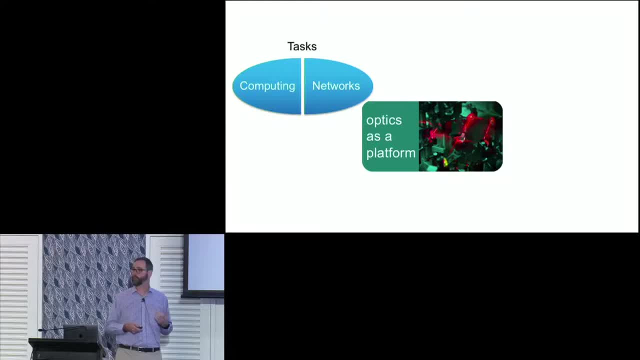 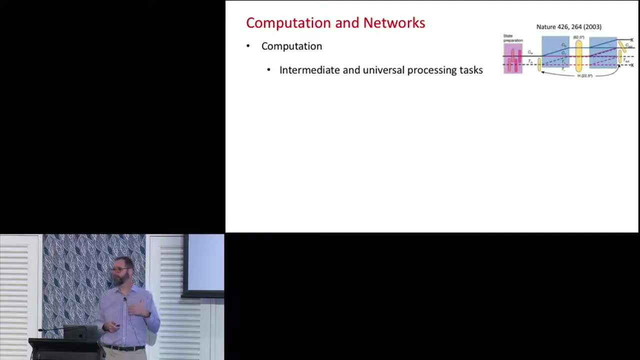 other quantum and quantum networks is another one. okay, and we heard in how Wiseman's tutorial- the other things like making precision measurements or doing other quantum and enhanced processes are in the mix as well, but I won't talk about those things today. so our computation: we're thinking about using optics for intermediate and for 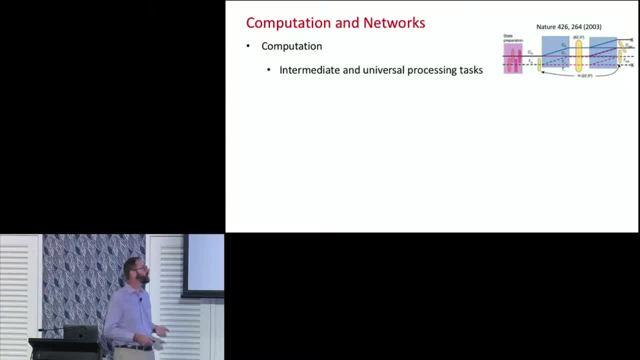 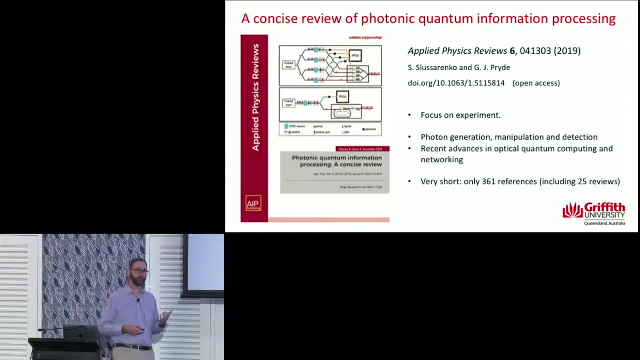 universal processing tasks are the first optical CNOT gate are demonstrated here, was demonstrated in our Center, and I'll say a little bit more about computation later on. but I'll do want to point you to a resource that you might be interested in if you're thinking about photonic or quantum computing with photos. 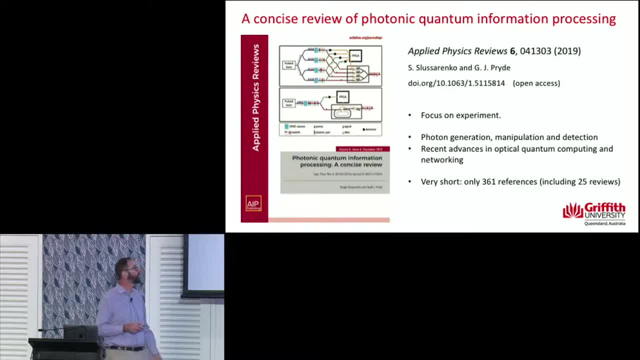 It's this review paper, pardon me, co-authored by Sergei and myself. What's really nice about this paper is that it's relatively short. okay, It's got a heck of a lot of references, and it references reviews that. look at all the 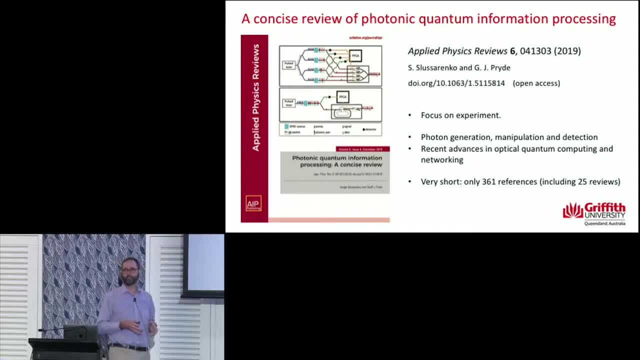 different sub-areas, but it's a pretty entry-level document. So if you have a new PhD student or you're just not particularly aware with it, why don't you start here, and then you can dive into as much of this sort of more detailed literature. 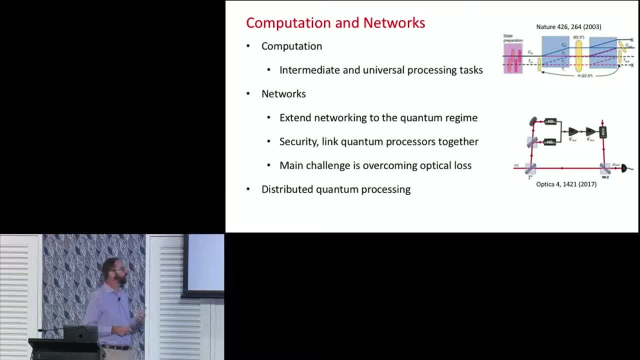 as you'd like. The other thing that I'm going to talk about- well, I'm not going to talk about very much in this talk, but I want to talk about it now- is the idea of using optics for networks, The idea of extending networking to the quantum regime, for security reasons, for linking processes. 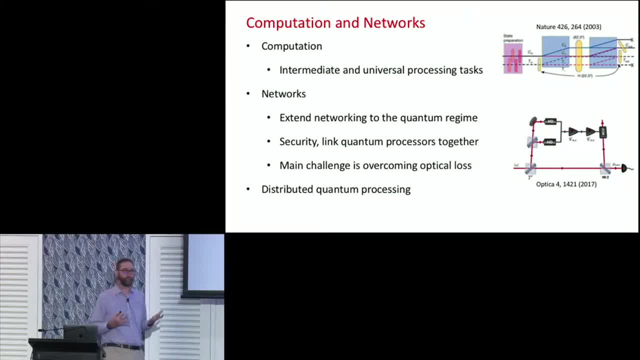 together, and what I want to tell you is that the main challenge is optical loss, and in other parts of this conference you'll hear about center-developed and center-implemented techniques for dealing with loss in optical encodings. okay, And so if we put the networking and the computation together, we can imagine some sort of distributed 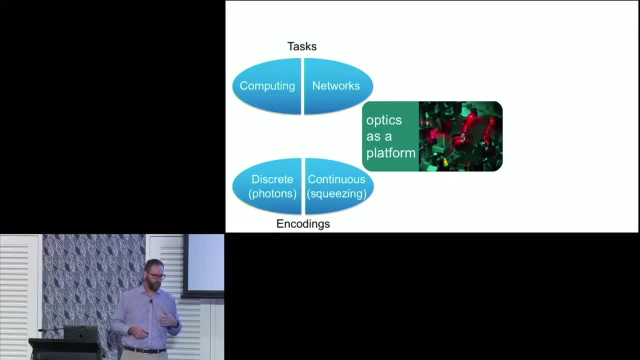 quantum processing, All right. so if we're going to think about doing these quantum information tasks with optics, we need to think about how we're going to encode our quantum information into optical systems, And today I'll talk about discrete encodings, or using single photons, and continuous encodings. 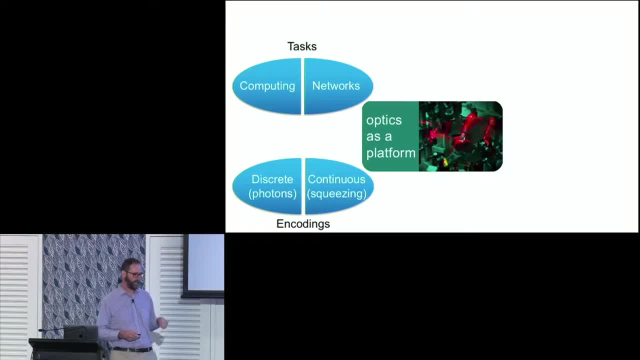 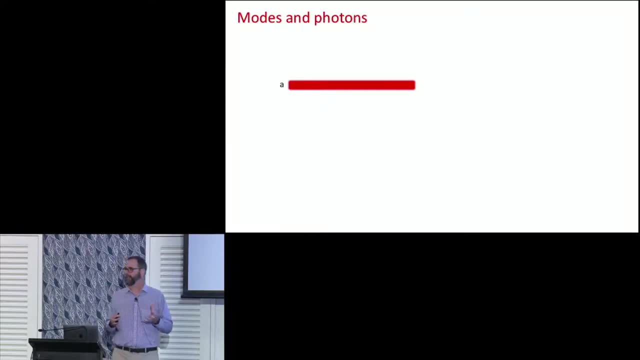 which is really more than just squeezing, but that's a little bit of an entry point into the field. And so to talk about this, we want to really start with the fact that, in optics, the most natural thing to talk about isn't so much the photon as the fundamental particle. it's. 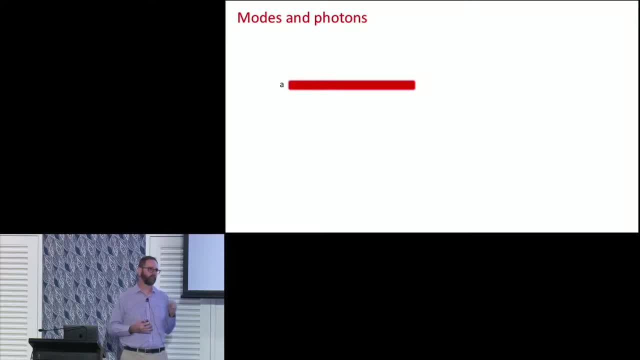 really the idea of an optical mode. This is something like a beam of light, okay, And it's not just defined by its spatial beam, like this laser pointer, but also by things like its frequency, by its timing envelope, by things like its transverse spatial mode. 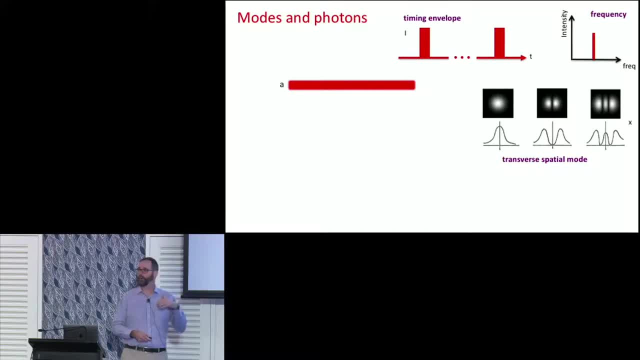 What shape is the cross-section of that beam? Is it Gaussian, Is it some more complicated Ermit-Gaussian mode, for example, And something like its polarization? okay, So if we have a particularly well-defined property in each of these, and perhaps some 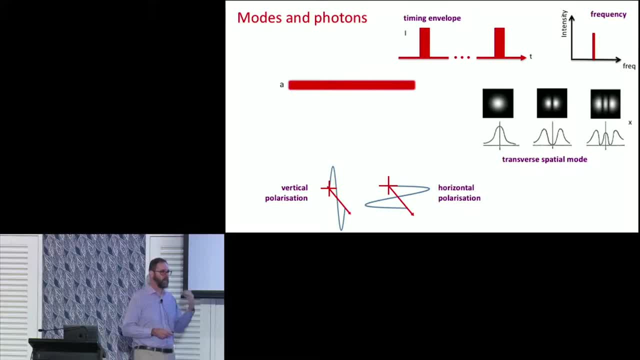 other degrees of freedom. then we can talk about an optical mode, And this is something that, in quantum mechanics, we model as a harmonic oscillator when we quantize light. Okay, so the most obvious thing is to take this optical mode that we've defined and to 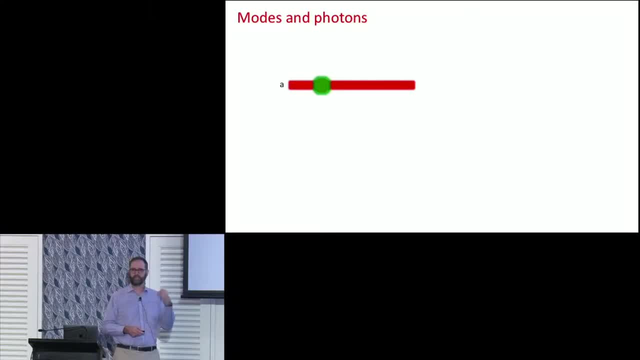 plop a photon into it, a single photon, okay, But this by itself isn't a qubit. We need a two-level system, And so, as Tim told us, a very natural way to do this is to superpose a photon across. 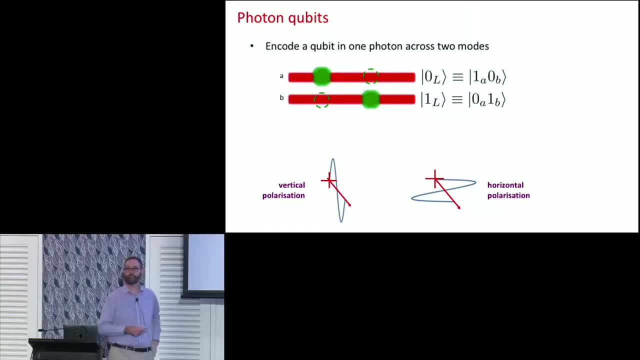 two different optical modes. okay, Perhaps there are two different spatial modes, as I've drawn here, or, more commonly, two different polarization modes, But it will depend a little bit on what materials platform we're going to end up using in conjunction with our optics. 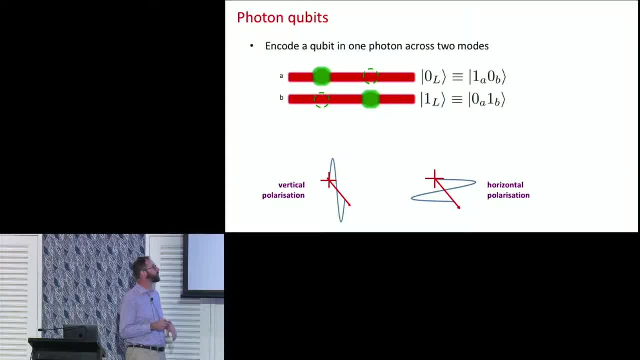 Okay, one of the photons in the top mode. we can call this a logical zero state. We label as one photon in mode A and zero in mode B. Vice versa, Vice versa for the other logical state. And of course we can make superpositions between one photon in one mode and one photon. 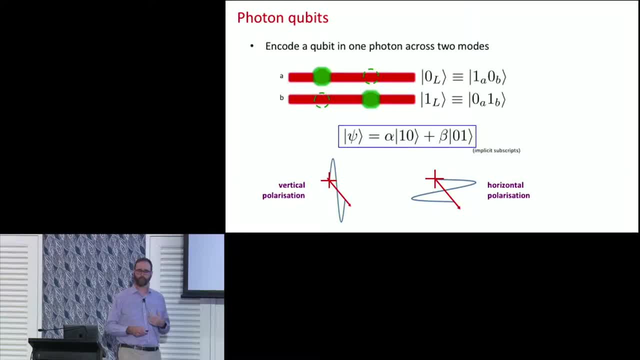 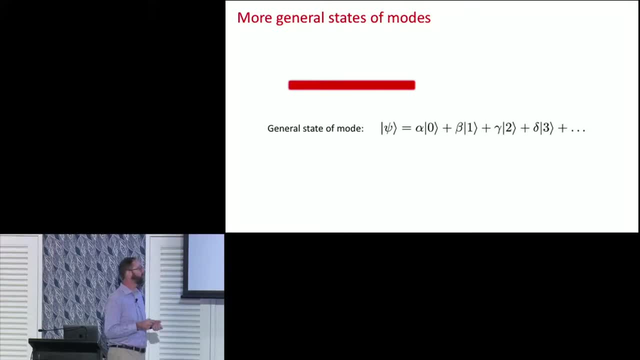 in the other mode And then we're off and going with photon qubits. But of course a single photon isn't the only thing we can put into an optical mode, And in general a single optical mode might have a pure state that looks something like: 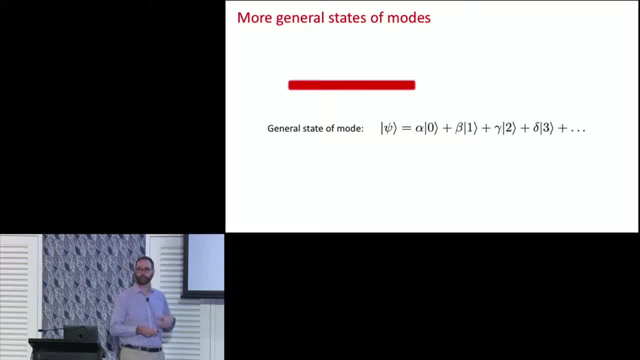 this a coherent superposition of the vacuum: one, two, three and higher order photon terms. In fact, the most common optical quantum state you might say is the coherent state. It's a quantum version of a nice monochromatic wave. 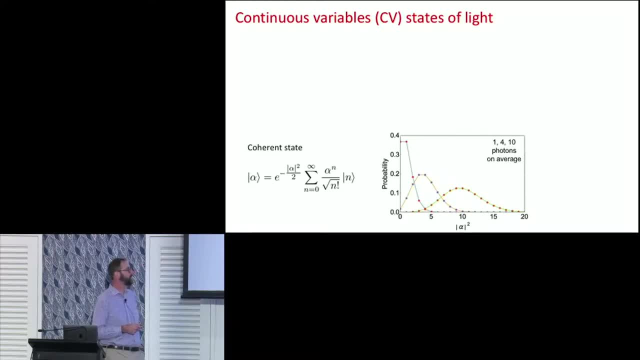 And we think of this in a photon number basis, as being expanded, something like this. okay, And so you have these different photon number distributions for different average photon numbers given by mod alpha squared. Okay, But So if we want to think about how we actually deal with this, how we think about it, how, 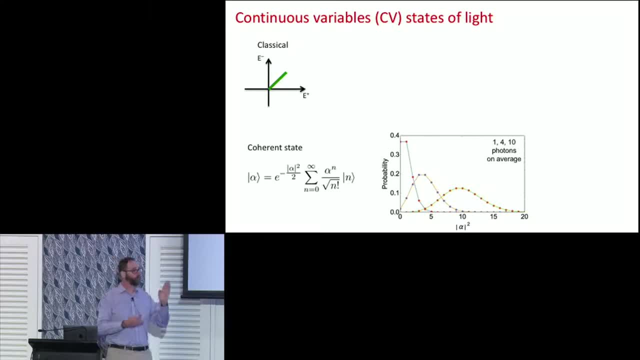 we measure it, then we can start with our classical notion of the quadratures of light. So, as I say, a monochromatic wave. We can think of it as having a sine omega t and a cos omega t component. We can write this down in a phaser diagram of our two quadratures, one proportional to 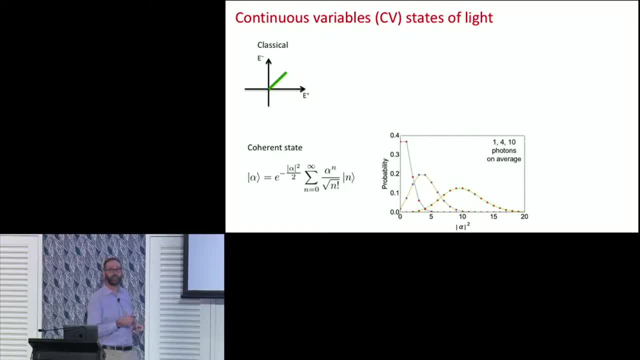 sine or cos and the phase given by the angle of this phaser. And in quantum light we come along and we just add Heisenberg's uncertainty principle to this. Okay, So we have uncertainty, this ball on a stick diagram here, which is associated with the 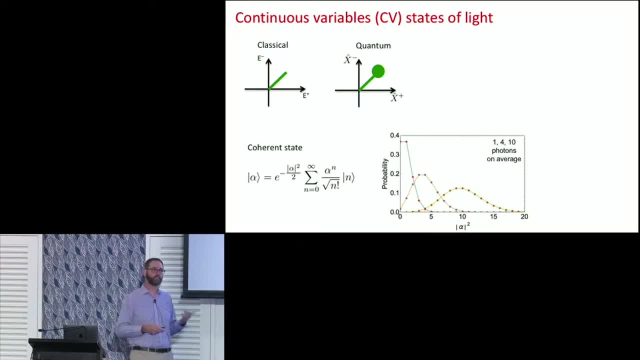 fact that these two quadratures, x plus and x minus, these quantum quadratures are really like the position and momentum of the harmonic oscillator: They don't commute and therefore there's an uncertainty relationship between them. And the key thing about that is because in the uncertainty relation we can trade off. 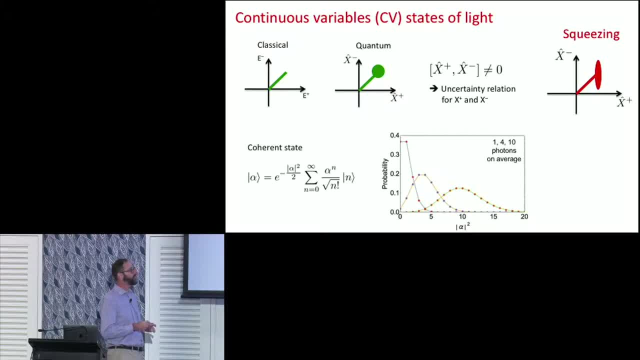 the uncertainty in p and x. Similarly, here we can trade off these uncertainties and we can squeeze one of them, or reduce the uncertainty at the expense of p and x- Okay, At the expense of the other one. And it turns out that this is a powerful resource for optical quantum information science. 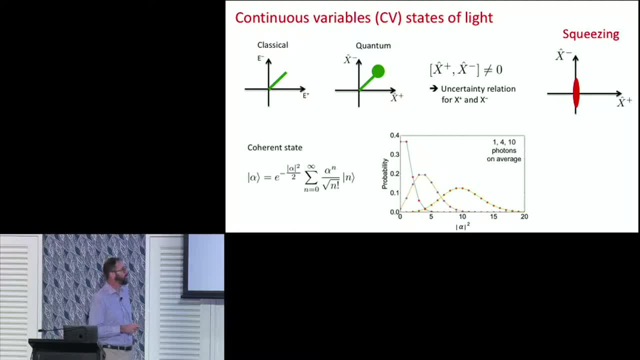 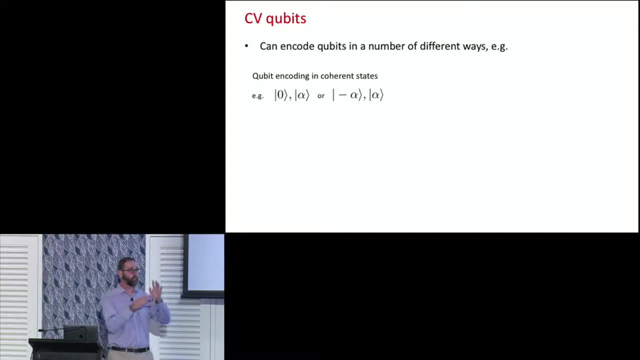 Okay, I also want to point out that in many experiments it's the vacuum itself, the zero photon state, which is squeezed, and so that's commonly what you'll hear about. Okay, So if we have these continuous variable states- continuous because those quadrature measurements- 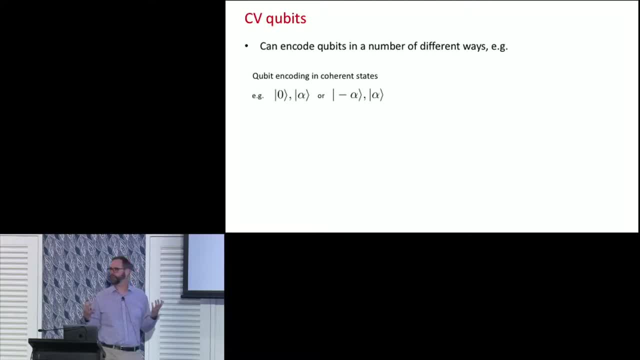 can give us any continuous value, Okay, And we can use that to turn that into some sort of you know qubit. So we might do something like using superpositions of coherent states. We might do something like using Gottesman-Kataev-Preskill states. 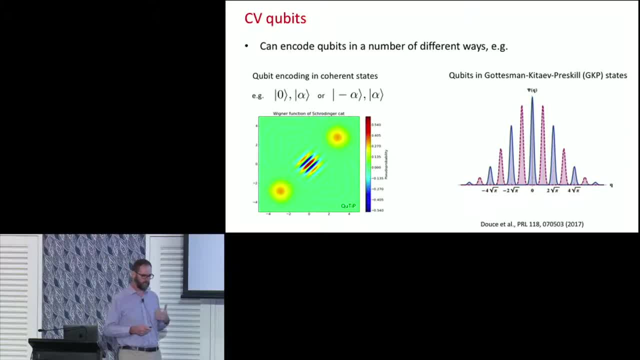 And there are other encodings as well and I think you'll probably hear something about those later in this conference. I don't want to go into the technical details of all of these, but simply to say that if we think about this quadrature phase space, there are different ways of defining orthogonal 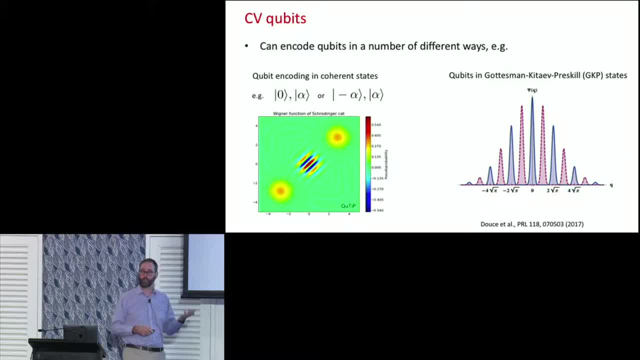 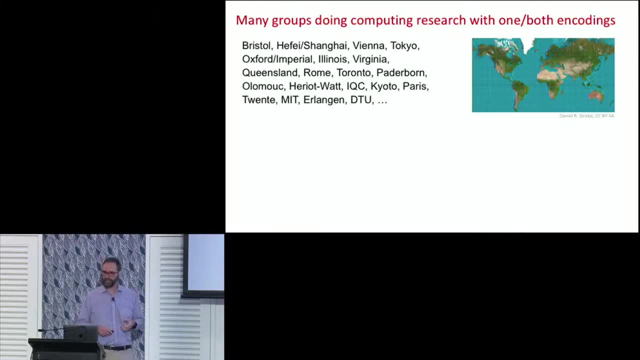 states within a space, Within a space in which you can use as basis states for computing and, of course, you can make superpositions of them All right. So there are many, many groups around the world working in all of this different space. 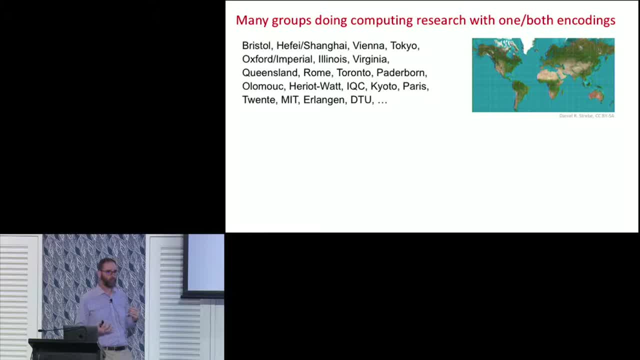 working with the discrete variable encoding, the continuous variable encoding, and working on some of the different kinds of problems that we're about to speak of at the moment. Here's a list, in no particular order, and it's not even a complete list, because this 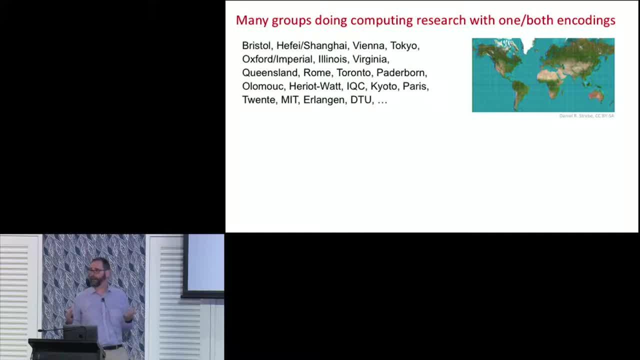 just captures a number of the major players. Okay, And here, by the way, are our partners within the center and who you'll hear about in other parts of this and other talks In this space- there's also a couple of major companies pursuing these approaches. okay. 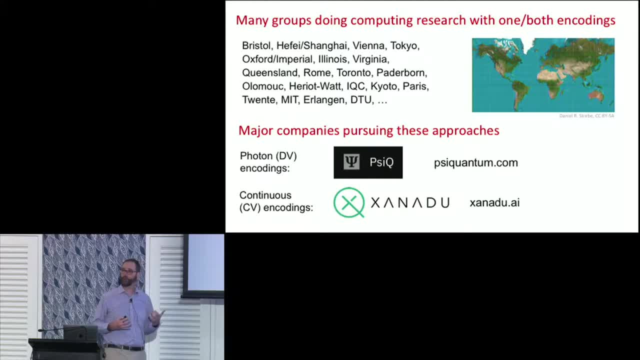 And there are two in particular that are notable In the photon encoding space. there's PsyQuantum, based in California, CEOed by Jeremy O'Brien, a former CQC2 team member, and also Xanadu, based in Canada, looking at continuous variables. 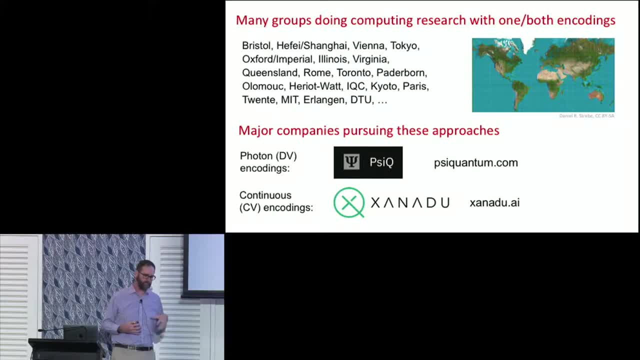 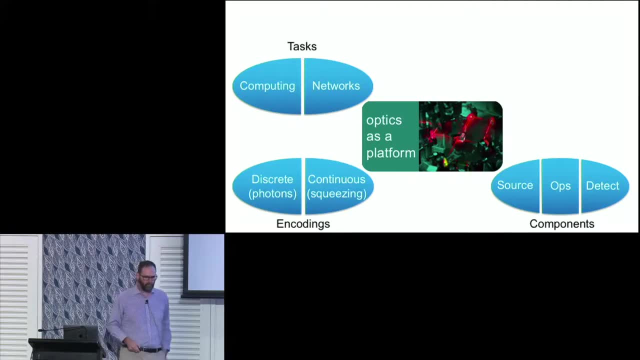 approaches. There's Christian Weebrook, who's also out of a center background as well. So these are the two big players in this space, And I want to talk a little bit about components. okay, So we have this idea that we can encode quantum information into light, and the question is: 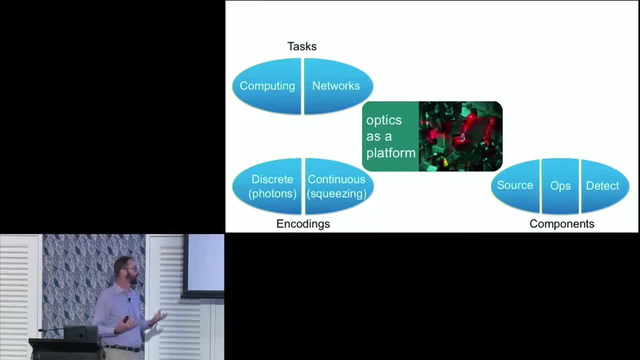 how do we do that? What is the hardware that we need in order to make this happen? And it really comes down to implementing sources of quantum light, detection of quantum light and, in the middle, some operations That one performs on it. 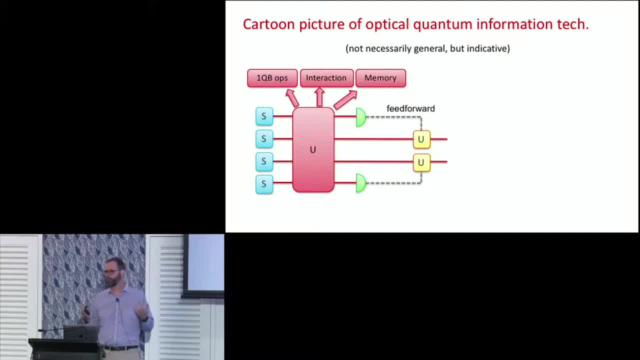 Okay, so here's a cartoon picture of optical quantum information science. It's a cartoon because it's really not representing any circuit in particular and it's not even particularly general, but it gives us a little bit of a flavor of what we might do with optical 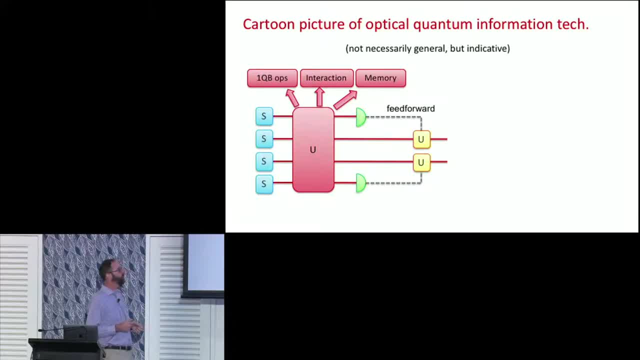 quantum states. Well, first of all, we have these S's sources of states. We need to generate our light and we need to encode information into it. Okay, then we need to do some processing on it, which is some single qubit operations. 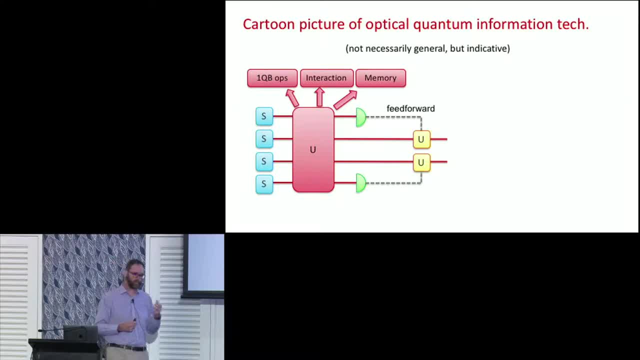 some interactions between different qubits, maybe some memory to store the light, although that's maybe not necessarily needed, as we'll talk about in a moment. And then often optical computing progresses by detecting some of these photons, reading them out and then using that information to feed forward onto the states of the remaining. 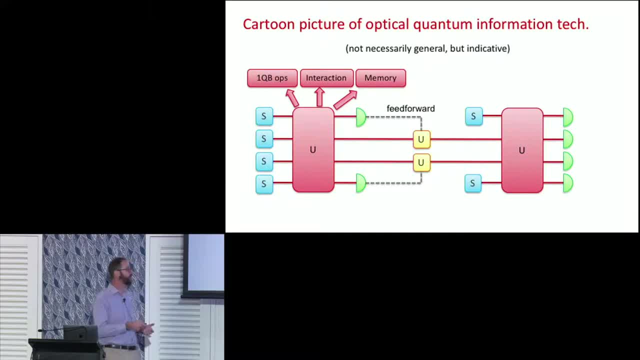 photons, And then one can introduce some new photons or some new quantum states and continue this until finally, at the end one reads out: Okay, so you can see that then we need to talk about sources, processing and detection as part of this model. 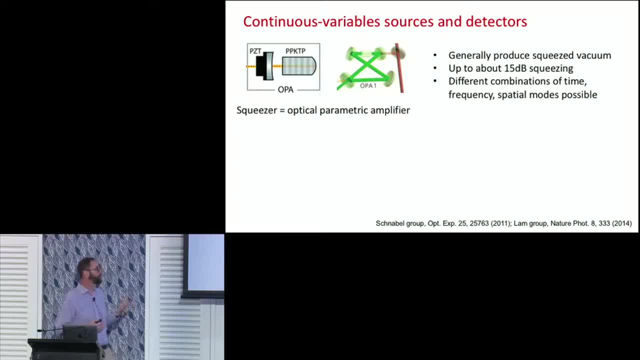 So in the continuous variable picture again, there are different ways of doing things, but often it comes down to the sources of quantum light being squeezes, which are optical parametric amplifiers working in a particular regime. Okay, so this might be something like a nonlinear crystal which is pumped by a laser in some 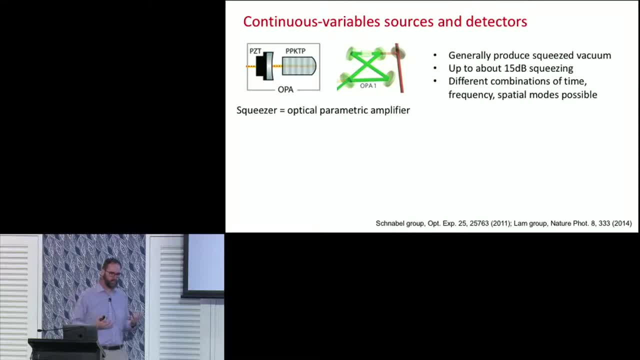 sort of cavity structure and in this regime they produce squeezed vacuum, is typically what happens, and we can see up about 15 dB of noise suppression in one quadrature. Okay, and so then, with this, depending on how you set up the optics and the properties, 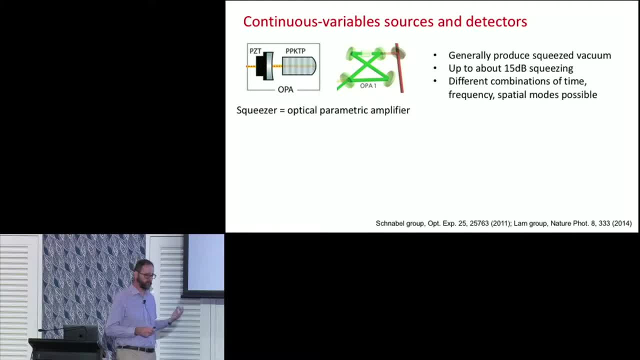 of this squeezer. you can then use different modes of light. You can think about temporal modes, frequency modes, spatial modes- See squeezing in all of these different polarization modes, Squeezing in polariztion modes, in all of these different degrees of freedom. 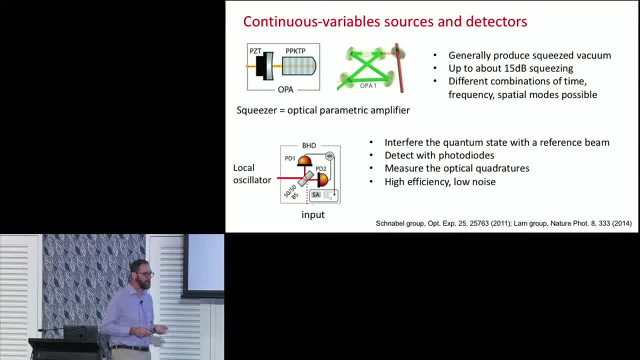 Pick whichever one is most suitable for your applications. The low noise detection that I mentioned earlier is typically done by balanced homodyne detection, And so the idea is to take the quantum state of interest and to mix it on a beam splitter or to interfere it. 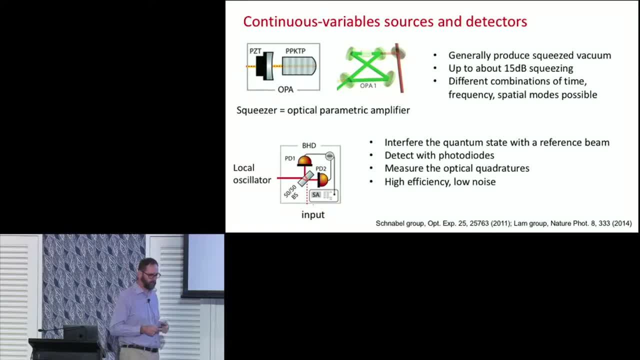 on a beam splitter with a local oscillator, which is typically a coherent state over which you have precise control, And then these are detected on high efficiency photodiodes. The different signal here gives us some common mode noise rejection, and we're able to make these quadrature. 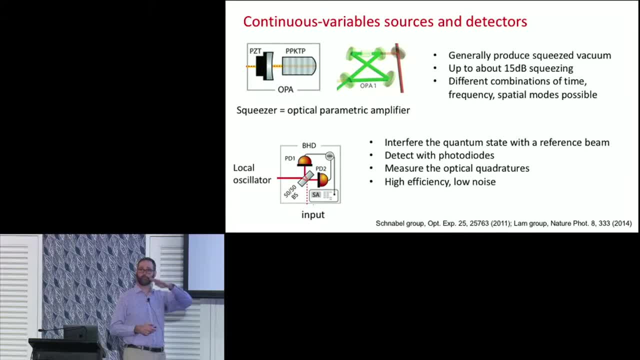 measurements that I spoke about earlier And measuring in different projections in that quadrature space is achieved by tuning the phase of the local oscillator, And so high efficiency, low noise measurements. So these are very robust techniques that work incredibly well. I haven't mentioned entanglement. 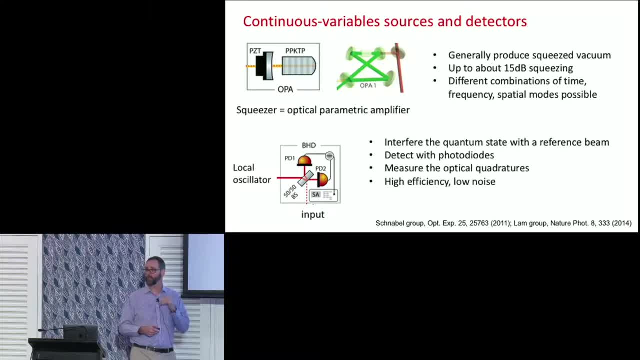 I'm here, But I want to tell you that there's a beautiful thing about continuous variables and squeezing, which is that if you take two squeezed states and you put them onto a beam splitter, you can make an entangled state, And it's a very simple, deterministic process. 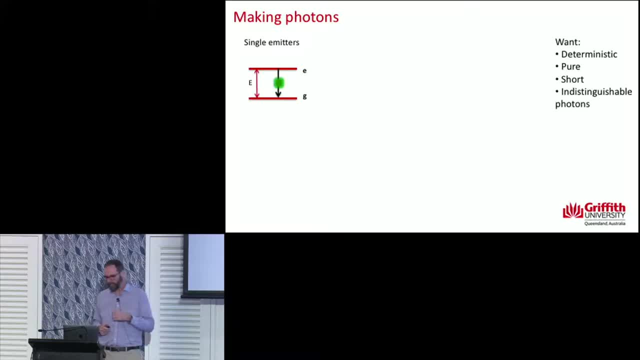 It's a really, really beautiful technique. So if we're thinking about a photonic encoding, then obviously making photons is the name of the game, And the obvious way to think about that is to take a system that has a single excitation in it. 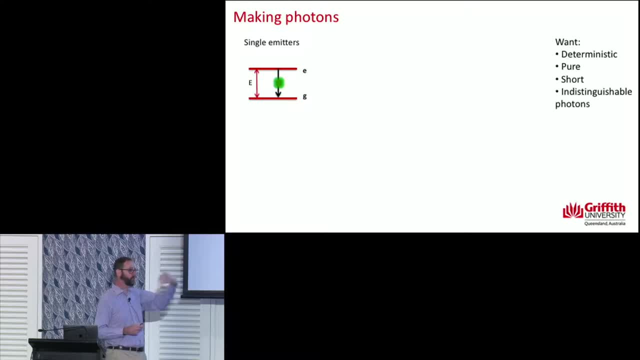 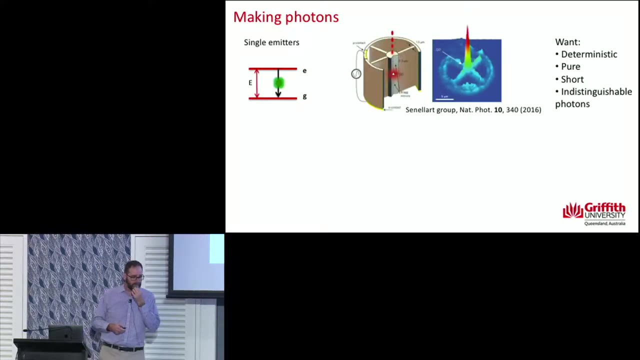 to let that excitation collapse and for the energy to come out in the form of a photon. So perhaps we have, like we learn in first year university, some sort of atom that's in an excited state and it emits a photon, something like that. 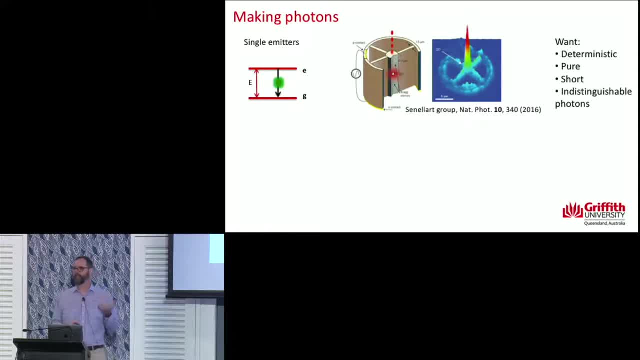 In order to be able to control and to capture that photon. it turns out that some sort of artificial atom like an NV center or like a quantum dot, as the example from the group here turns out to be a good way to do it. 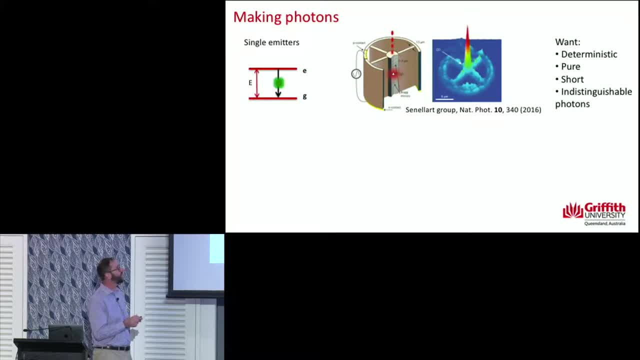 Why is that? Well, in here we have a quantum dot which is in a micropillar structure here, which means that the photon can be collected and emitted in a preferred direction. So it makes it unlike an isolated single atom, which 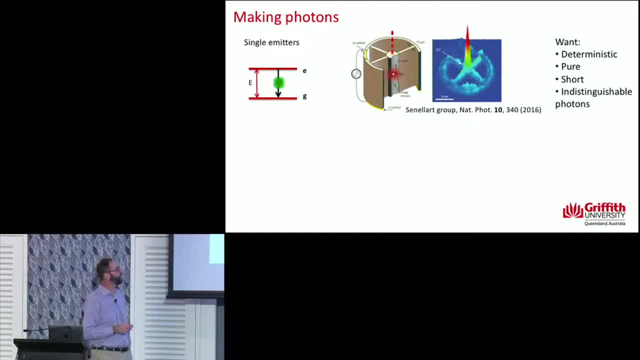 radiates in all directions. Here we can have some directional emission, And so the papers from this and from other teams are really starting to show some amazing results. in this case, These kinds of technologies give us a good step towards what we want, which is sort of deterministic, so on-demand photons. 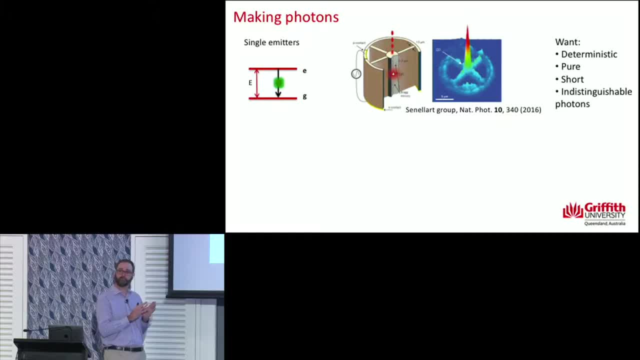 pure photons, usually temporarily short so that we can access them on a fast cycle, and photons that are indistinguishable, so that if I take two photons from the same device or from two separate devices, they can be interfered with very high fidelity. 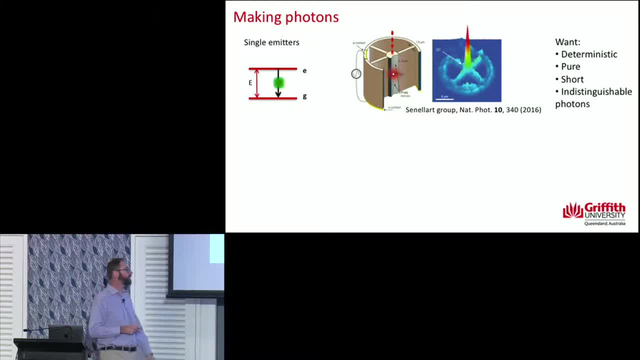 And quantum dots. These are one of the contenders for meeting these kinds of goals. Another contender, which seems like at first an unnatural one but is actually an exceptionally good contender, is the idea of spontaneous parametric down conversion. So in this process there's a nonlinear crystal. 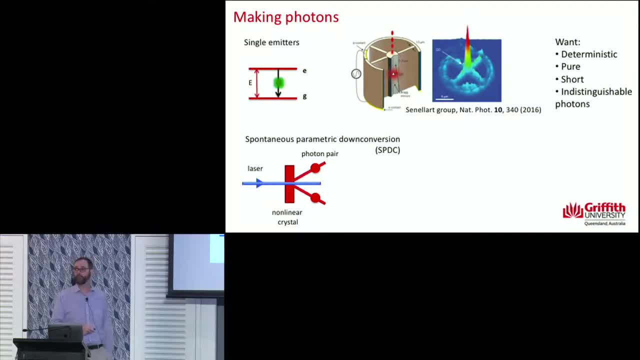 which is this sort of solid vertical box that is pumped by a bright laser And sometimes randomly, pairs of photons are emitted, So one of the pump photons is destroyed And, conserving energy and momentum, a photon pair is generated. OK, these are generated randomly. 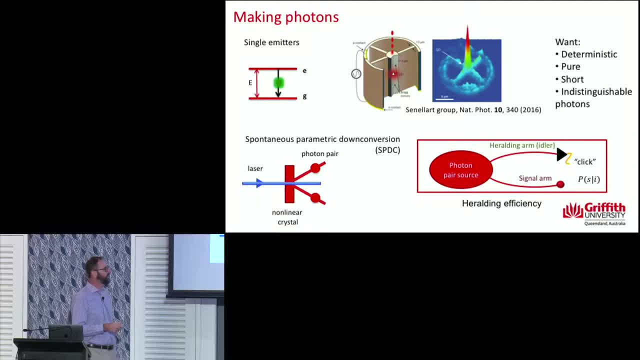 And so that doesn't seem so useful, But because they're generated in pairs. if we measure one of those photons, then with extremely high efficiency. in principle unit efficiency, but in practice a number given by the so-called heralding efficiency, depending on various experimental constraints. 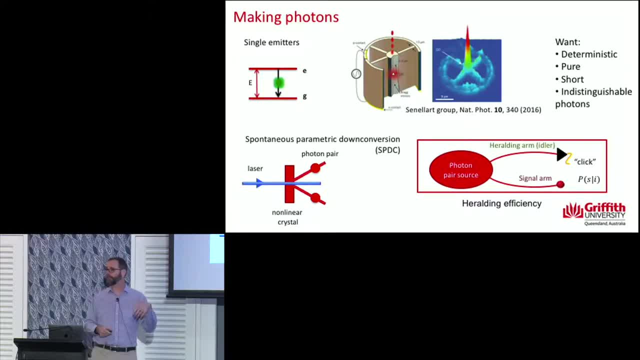 with very high efficiency, we can have one photon in the other arm, And with a suitable kind of detection, we can guarantee that we have one and only one photon here. OK, and so while this source is not inherently deterministic, it does produce, if they're properly engineered. 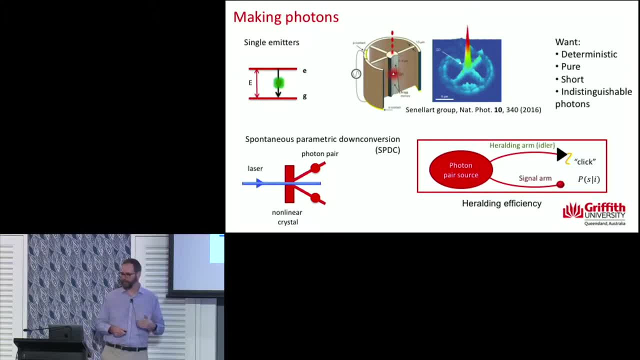 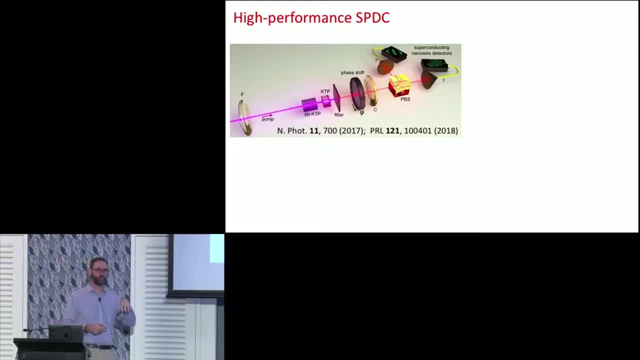 very pure, very indistinguishable and in every other way very nice photons. So for the rest of the talk, I'm going to talk about quantum dots and down conversion, But keep in mind that there are alternative technologies as well, But perhaps they're the two front runners at the moment. 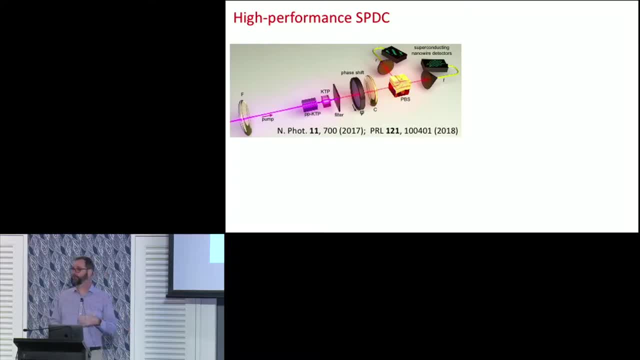 OK, so in the center we're very good at doing high-performance spontaneous parametric down conversion. Here's an example of a setup that does that Basically. here's the pump laser and the down conversion crystal, And then here are the two photons, one of which 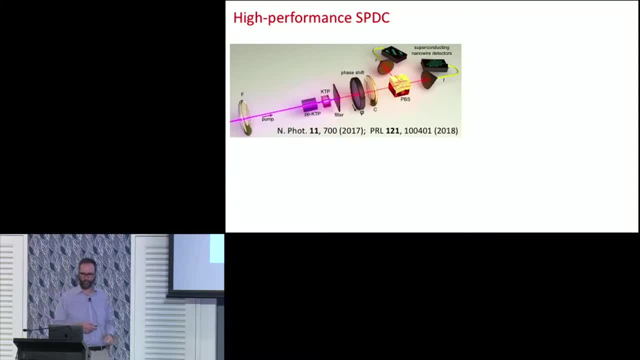 is detected or here the other one's detected as well. But in principle it can go off to experiments and you can do what you want. You can have very high visibility- typically 99% or better- And also you can have very high visibility. 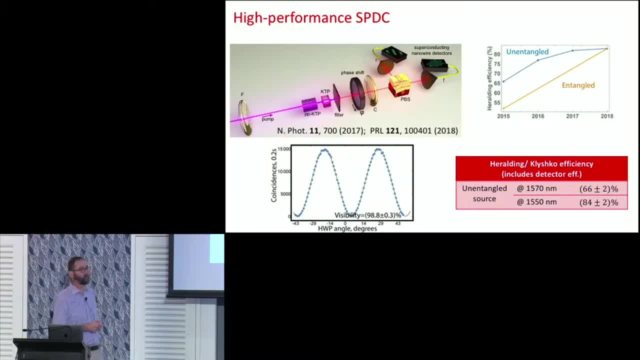 And also very high heralding efficiency. So for an unentangled sources, and also these sources can generate entangled pairs, although not in a heralded way, And again with very high efficiency. OK, so numbers sort of including the ultimate detection. 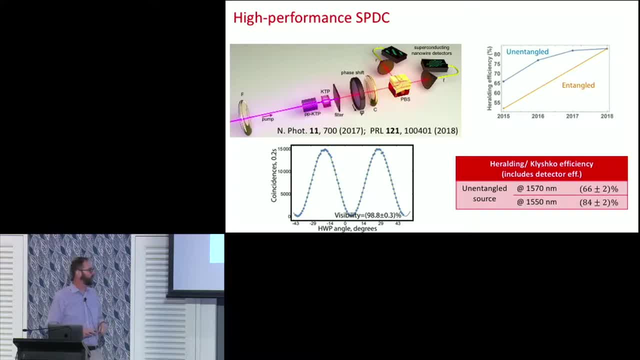 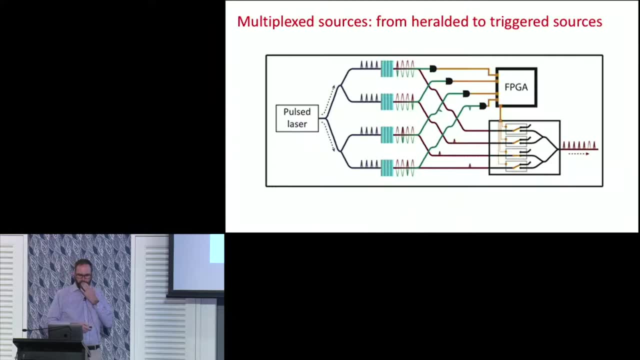 efficiency. so factoring nothing out at all, sort of getting to the 85-plus percent kind of range. All right, so down conversion is a promising technique for giving us nice pure photons, But even so we have to herald those photons. 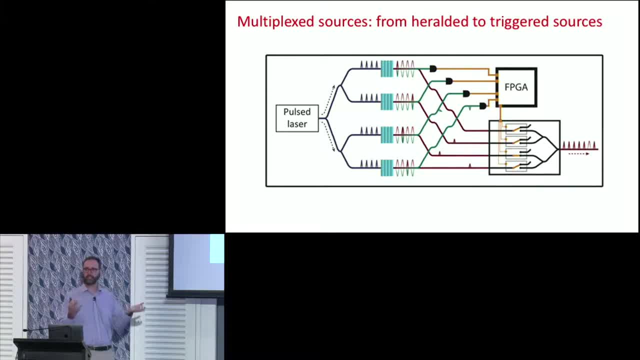 And those heralding events happen at random times. How can we take that sort of technology and turn it into a source that's periodic or that's perhaps triggered, so that when you press a button, so to speak, a photon comes out And the idea here is to use what's? 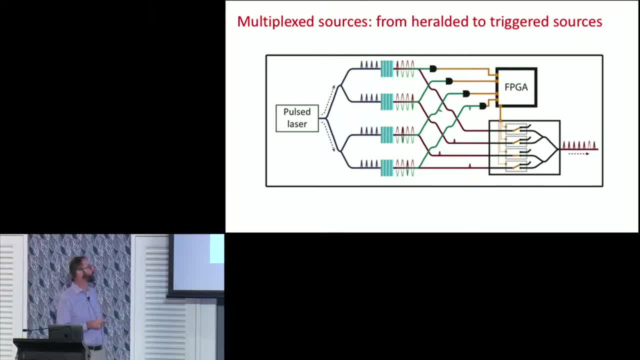 often known as multiplexing. OK, And it's quite a simple idea. The idea is that one takes many such sources- four are shown in this particular diagram- and each of these sources will fire randomly in time. OK, But one of the photons from each of them goes to a detector. 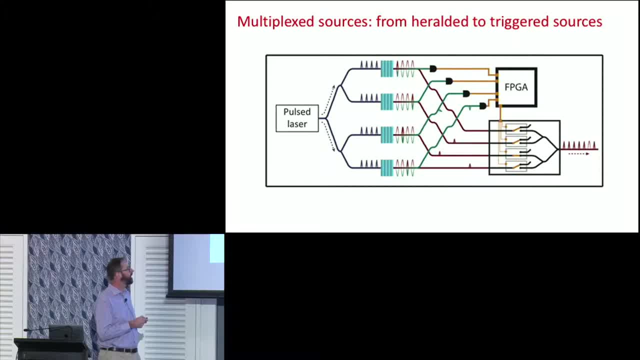 and we see which one fires. And then whichever one fires, we switch the corresponding mode. So perhaps it's the top one. Here's the remaining photon. We switch that into the output. OK, And with sufficiently many sources, then one can have a very high probability. 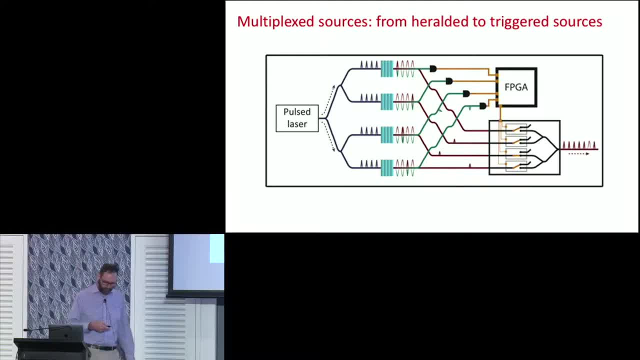 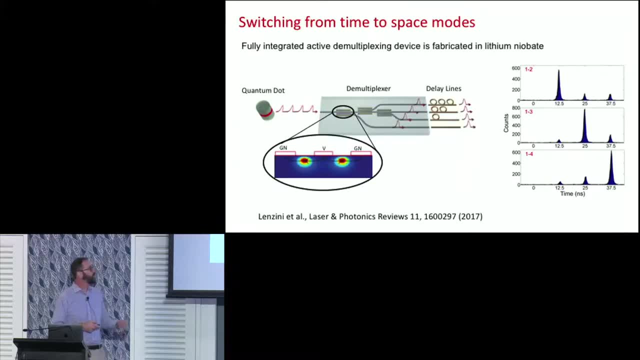 of being able to complete this protocol and have near deterministic single photon sources. I should just say that the reverse is also possible: to use a similar kind of technology to go from one particular pulse train here into different spatial modes. And so here's an example of center work. 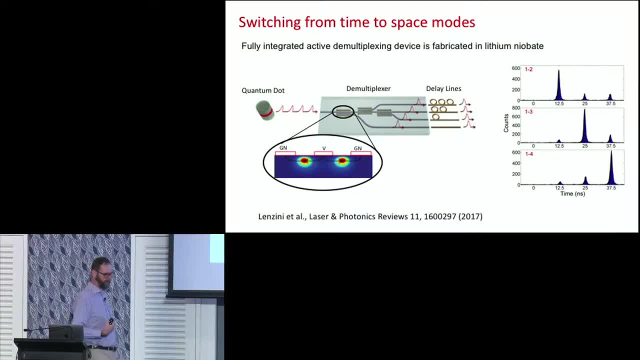 that's doing exactly that. So this is from the group of Miyako Labino, collaborating with our colleagues at University of Queensland, And the idea here is to have a lithium niobate waveguide device with fast switches here that switch basically the light between these different output modes. OK, 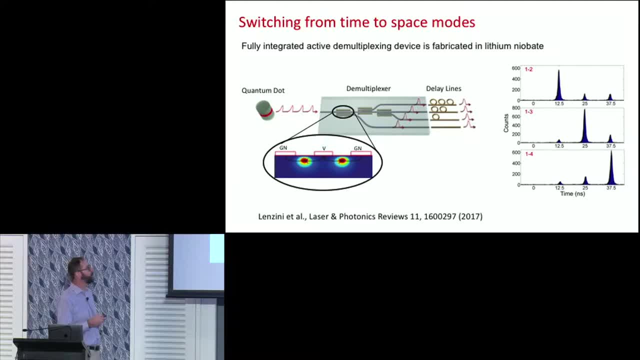 So the quantum dot here in this case emits this pulse train of photons, And the idea is, that's all very nice if we want them in temporal modes, but perhaps we want to switch them out into different spatial modes, And so that's possible by basically using 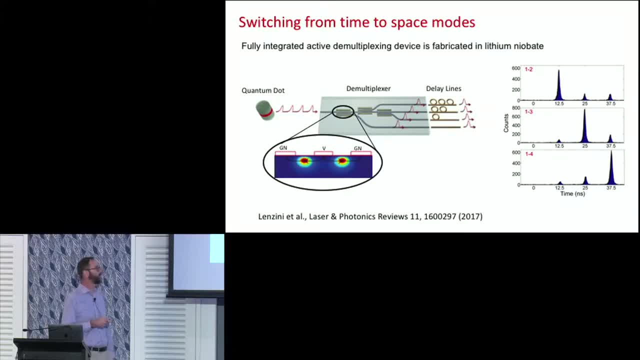 this lithium niobate device, which I'll say more about a little later in the talk, in order to do that, And you can see that you can get switching between channel 1 and 2, channel 1 and 3, and so on. OK, 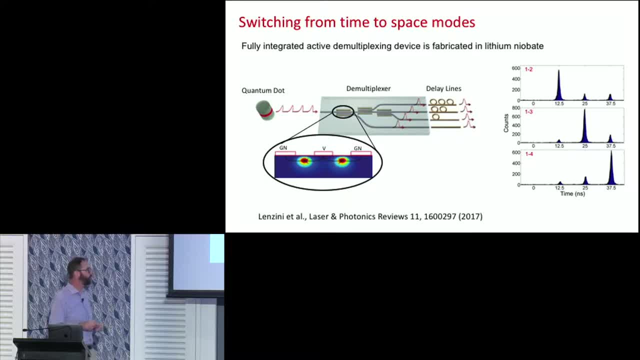 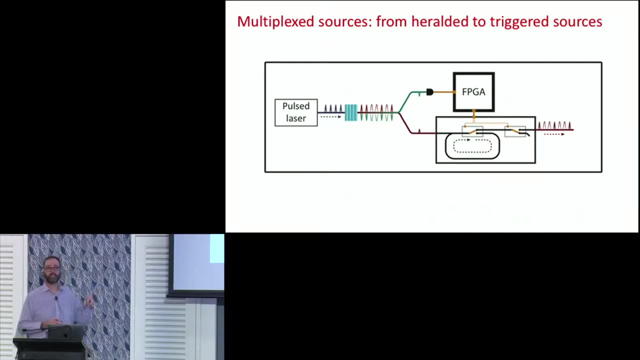 And the key thing is that this is all done in a compact, integrated platform and can be done at very high speeds. OK, so switching between time and space are possible for a bunch of different applications. I should just also point out that one of the apparent inconveniences of the first multiplexing scheme 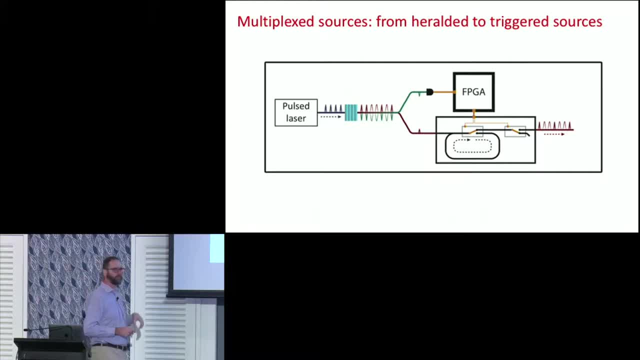 I showed you is that one has to have many sources in parallel, But you can temporarily multiplex instead. So instead you just have one source here. The photons here are sort of spat out at various random times Wherever one of these pulse pairs is full. 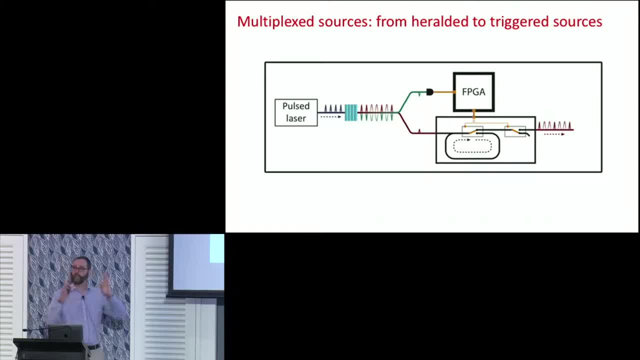 then we're imagining a pair being generated. If we define a block of these pulses as being one clock size, then within the clock cycle it's very likely that one of these, one of these, one of these pulses will be filled and we can store the pulses in a loop and 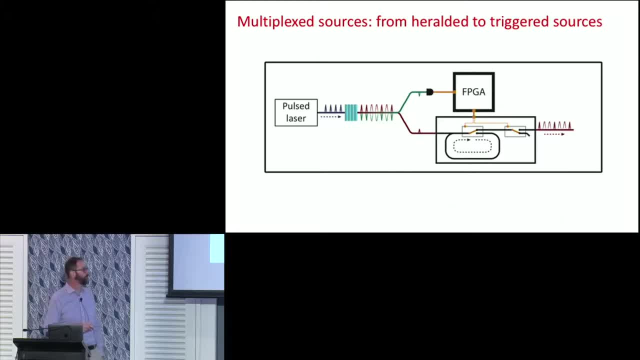 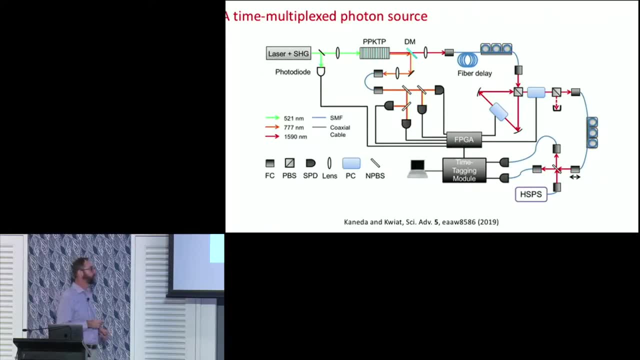 then switch out the one where it was stored in a periodic fashion, as shown here, and this isn't only hypothetical- this group, Paul Kwiat's group at the University of Illinois, who have done exactly this. the experiment looks rather complicated, but we can focus in on the key part here in the middle. this, this. 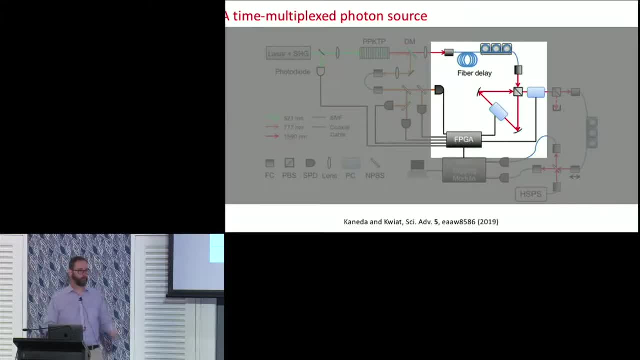 loop. here this triangular loop is, is the the storage loop for the photons. here's the detector that heralds the presence of it. a photon is switched into this loop and then, at the end of the end of the clock cycle, it can be switched out with high efficiency and high fidelity. okay, so here's an example of a graph. 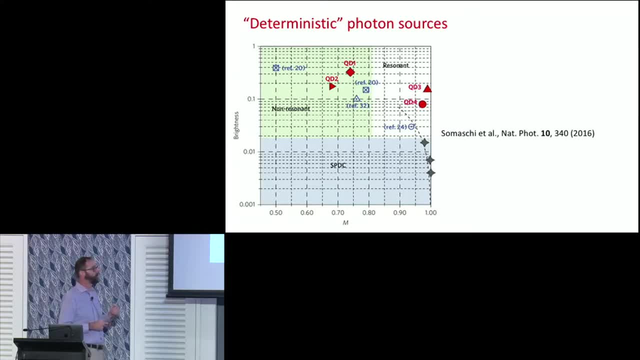 taken from a quantum diagram of a graph. taken from a quantum diagram of a graph. taken from a quantum diagram of a graph. taken from a quantum dot paper from the Sennelaar group. which dot paper from the Sennelaar group. which dot paper from the Sennelaar group, which is comparing different kinds of sources. 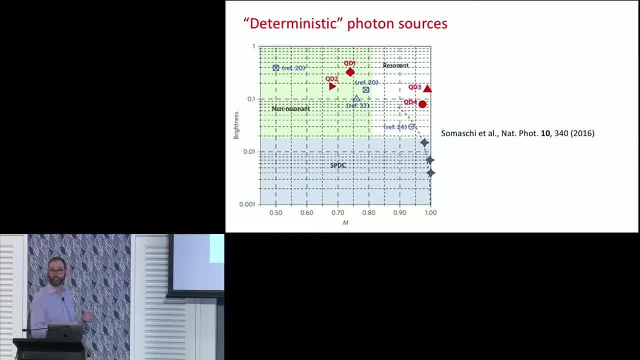 is comparing different kinds of sources. is comparing different kinds of sources across the horizontal axis, roughly across the horizontal axis. roughly across the horizontal axis, roughly speaking, is the quality of the source. speaking is the quality of the source. speaking is the quality of the source. won't go into detail about exactly what. 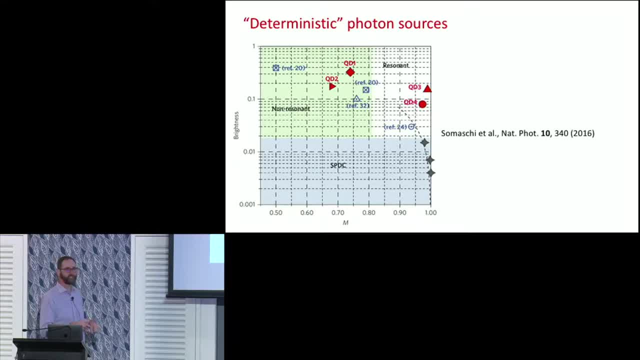 won't go into detail about exactly what. won't go into detail about exactly what this M parameter quantifies, but it's this M parameter quantifies, but it's this M parameter quantifies, but it's: it's approximately how interferable the. it's approximately how interferable the. 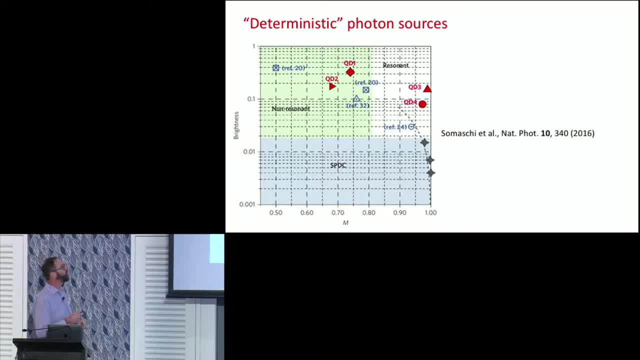 it's approximately how interferable the photons are. so one is ideal. here's: the photons are so. one is ideal: here's: the photons are so. one is ideal. here's the brightness, brightness. one in this brightness, brightness, one in this brightness. brightness, one in this context means every time you ask for a. 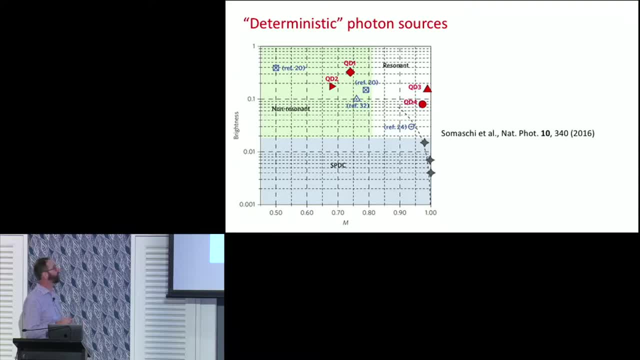 context means every time you ask for a context means every time you ask for a photon, you, you can collect and use photon. you, you can collect and use photon. you, you can collect and use exactly one photon, obviously one can go. exactly one photon, obviously one can go. 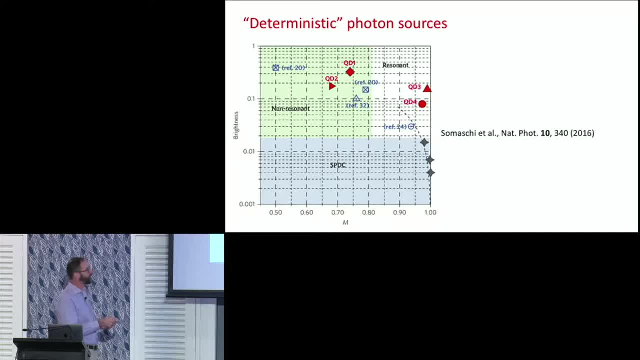 exactly one photon. obviously one can go down from there, so down. conversion gives down from there, so down conversion gives down from there, so down conversion gives you very, very clean photons. these are you very, very clean photons. these are you very, very clean photons. these are these sort of gray markers over here on. 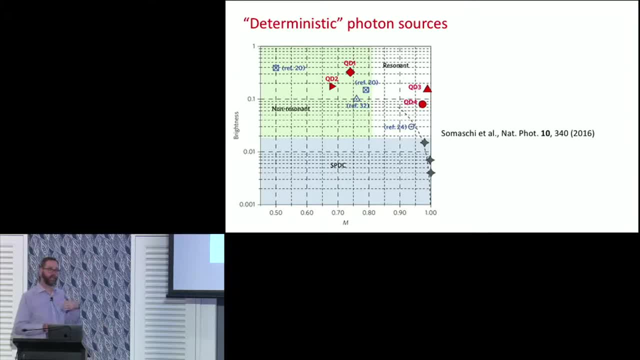 these sort of gray markers over here on these sort of gray markers over here on the right-hand side of the graph. but you, the right-hand side of the graph, but you the right-hand side of the graph, but you can see that without any additional, can see that without any additional. 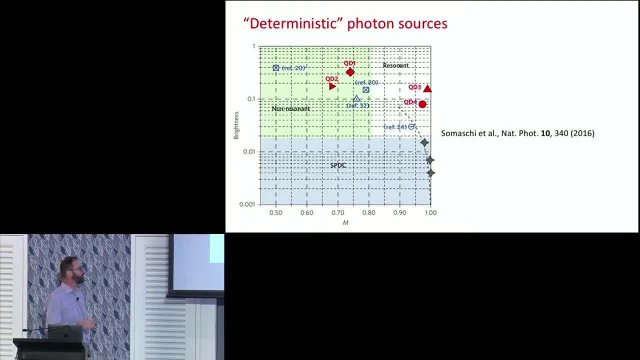 can see that, without any additional techniques, the rates can be low. because techniques the rates can be low. because techniques, the rates can be low because the probability of getting an emission, the probability of getting an emission, the probability of getting an emission is low. it's a random process, okay. 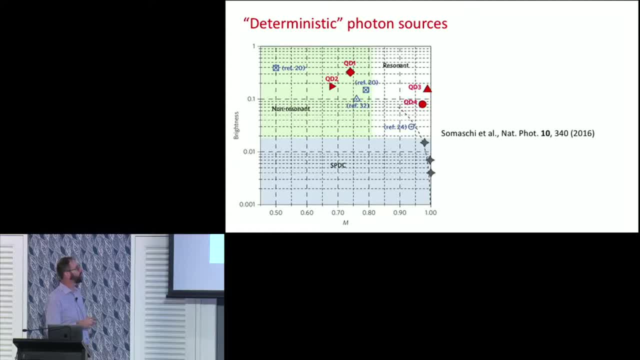 is low, it's a random process. okay is low, it's a random process, okay. quantum dots given here, different groups. quantum dots given here, different groups. quantum dots given here, different groups, including the red ones by the Sennelaar. including the red ones by the Sennelaar. 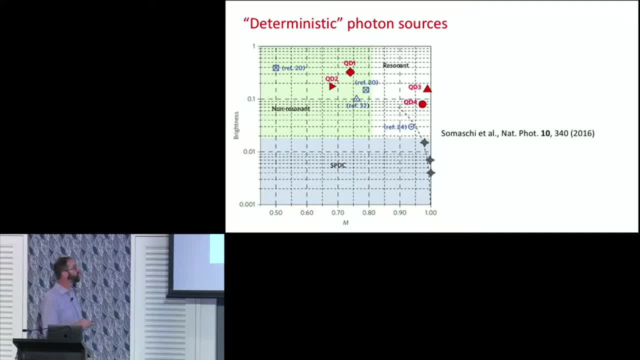 including the red ones by the Sennelaar. group give you higher performance, but group give you higher performance, but group give you higher performance, but still we're talking about 20-30 percent. still we're talking about 20-30 percent. still we're talking about 20-30 percent. brightness okay, and some of them high. 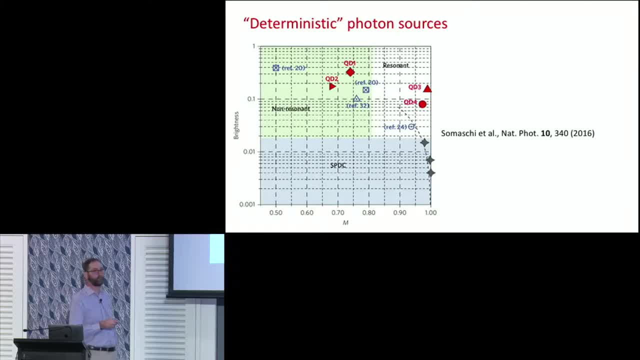 brightness okay, and some of them high brightness okay, and some of them high, high, high interference probability and high, high high interference probability and high, high high interference probability and some of them not so much. if you take some of them, not so much if you take some of them, not so much if you take separate dots. dots photons interfered. 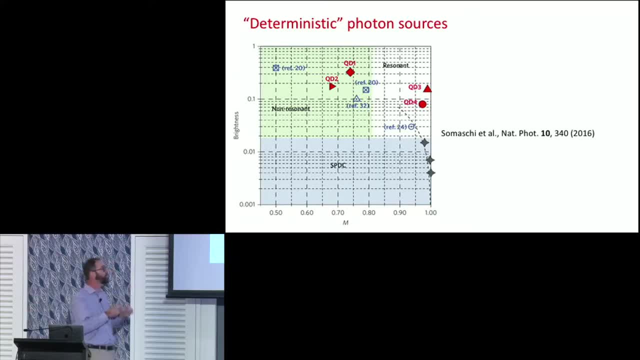 separate dots, dots photons interfered separate dots, dots photons interfered from two completely separate devices, from two completely separate devices, from two completely separate devices that have different materials properties, that have different materials properties, that have different materials properties. then, even though they're in principle, then even though they're in principle, 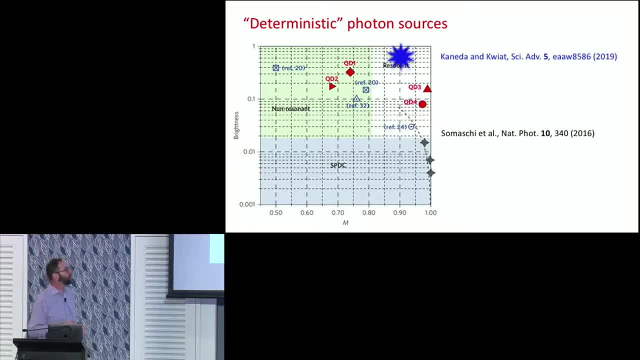 then, even though they're in principle identical, then these numbers tend to identical, then these numbers tend to identical, then these numbers tend to decrease. so the clear result: I just decrease. so the clear result: I just decrease. so the clear result I just showed you is is up here. this is what 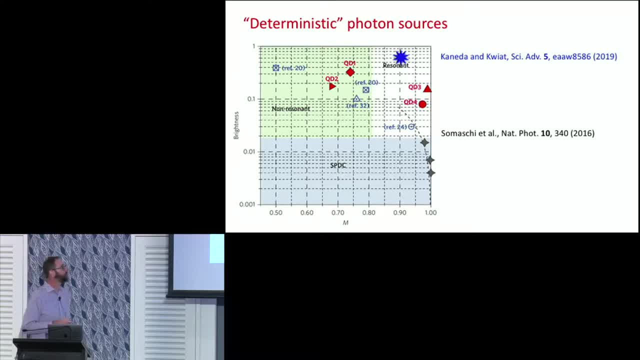 showed you is is up here. this is what showed you is is up here. this is what you can do by heralding down conversion. you can do by heralding down conversion. you can do by heralding down conversion. and this was the, I guess, the first time. 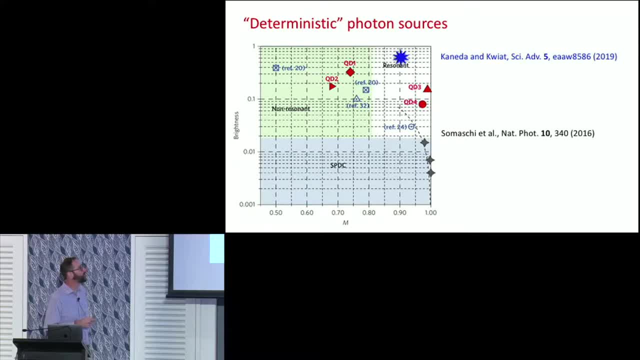 and this was the I guess the first time, and this was the I guess the first time it's been done in a very serious way. so it's been done in a very serious way, so it's been done in a very serious way, so you can see pretty high efficiency and 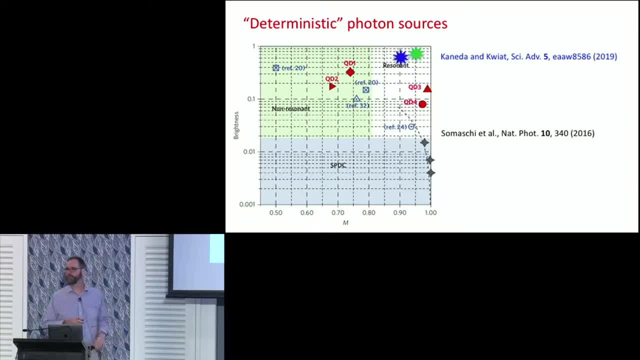 you can see pretty high efficiency. and you can see pretty high efficiency and the visibility is not too bad. with some. the visibility is not too bad with some. the visibility is not too bad with some simple improvements. one could simple improvements, one could simple improvements. one could immediately get to the green dot and I 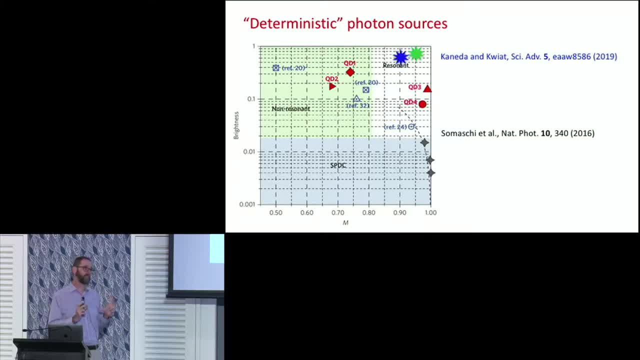 immediately get to the green dot and I would just say that the kinds of down would just say that the kinds of down would just say that the kinds of down conversion source, the high quality conversion source, the high quality conversion source, the high quality sources that we make are very much. 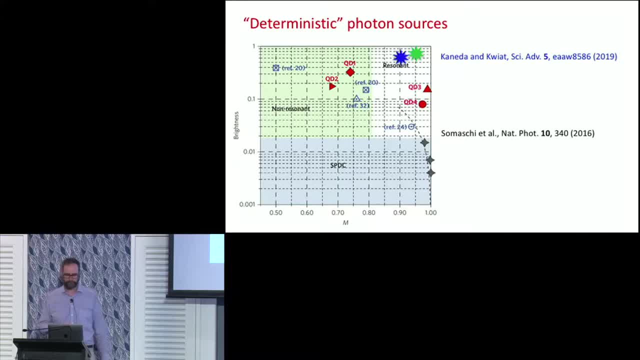 sources that we make are very much sources that we make are very much integral, integratable into this kind of integral, integratable into this kind of integral, integratable into this kind of technology. and how small a corner would technology and how small a corner would technology and how small a corner would be truly interesting for LOQ see how. 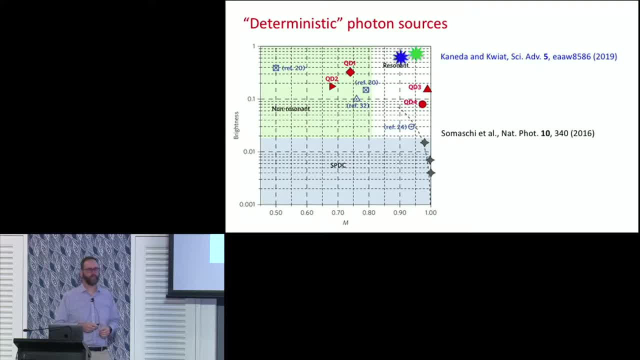 be truly interesting for LOQ. see how. be truly interesting for LOQ. see how long is a piece of string. yeah, it's long is a piece of string. yeah, it's long is a piece of string. yeah, it's, it's a. it's a tricky question. it depends. it's a. it's a tricky question. it depends. it's a. it's a tricky question. it depends on what encodings you want to use. maybe on what encodings you want to use. maybe on what encodings you want to use. maybe I'll say more about it at the end, if 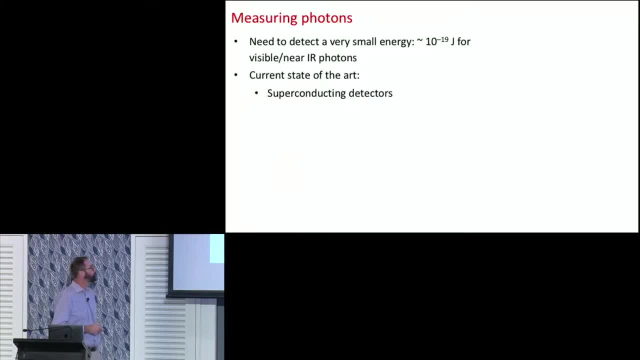 I'll say more about it at the end. if I'll say more about it at the end, if that's, if that's okay, yep, okay. so that's, if that's okay, yep, okay. so that's, if that's okay, yep, okay. so that's making photons, so we need to. 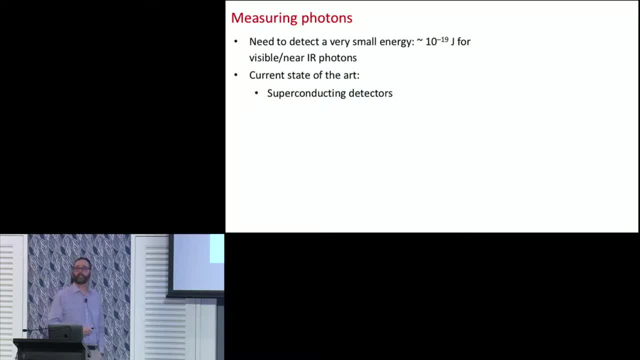 that's making photons, so we need to. that's making photons, so we need to measure them as well. and the idea here: measure them as well, and the idea here: measure them as well. and the idea here is that we're looking to, you know, is that we're looking to, you know. 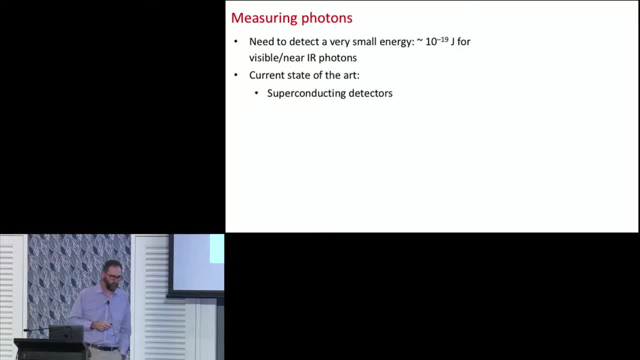 is that we're looking to. you know, detect a very small amount of energy. of detect a very small amount of energy. of detect a very small amount of energy of order 10 to minus 19 Joules. okay for the order: 10 to minus 19 Joules. okay for the. order 10 to minus 19 Joules. okay for the kinds of photons that we're interested, kinds of photons that we're interested, kinds of photons that we're interested in and there's much to be said about in and there's much to be said about. 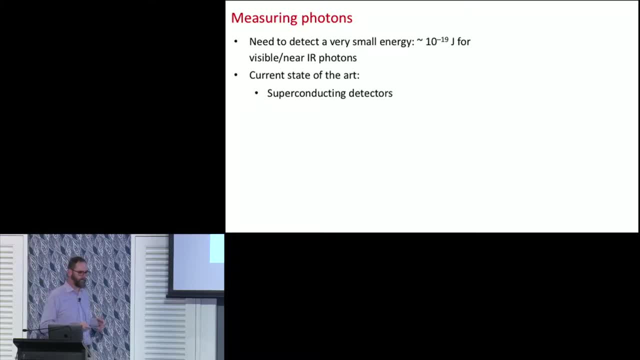 in, and there's much to be said about detectors, but let's just go to the state detectors. but let's just go to the state detectors, but let's just go to the state of the art which is superconducting, of the art which is superconducting. 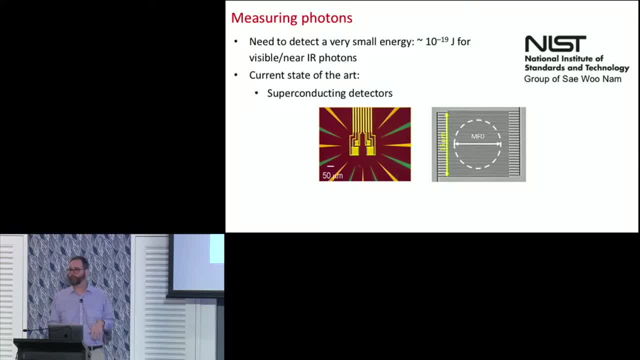 of the art which is superconducting detectors, and one of the leaders in this detectors and one of the leaders in this detectors and one of the leaders in this field is the group of say woonam at NIST field is the group of say woonam at NIST. 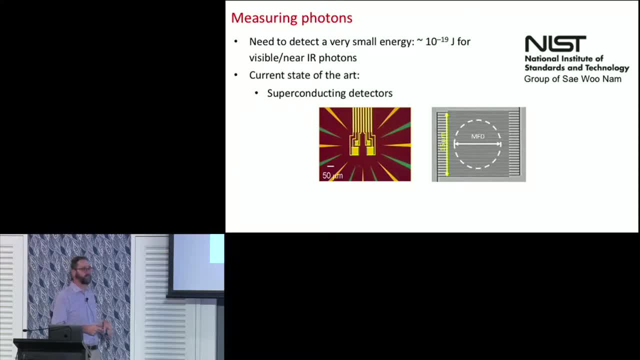 field is the group of say woonam at NIST. who makes these transition edge? who makes these transition edge? who makes these transition edge superconducting? and these nanowire superconducting and these nanowire superconducting and these nanowire superconducting detectors in tungsten. 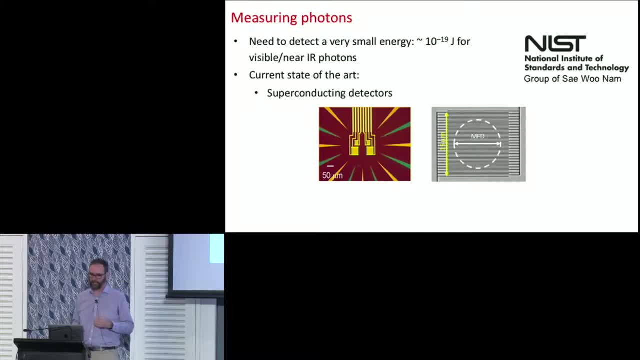 superconducting detectors in tungsten. superconducting detectors in tungsten. psilocyde: there are other groups making psilocyde. there are other groups making psilocyde. there are other groups making competing platforms or doing making competing platforms or doing making. 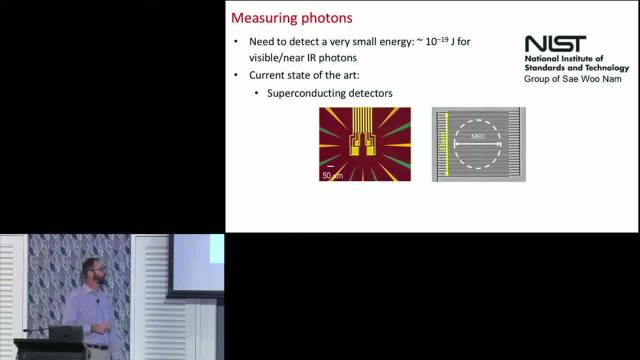 competing platforms or doing making similar things. there are companies that similar things. there are companies that similar things. there are companies that produce these, although I believe that at produce these, although I believe that at produce these, although I believe that at the moment say we makes the highest. 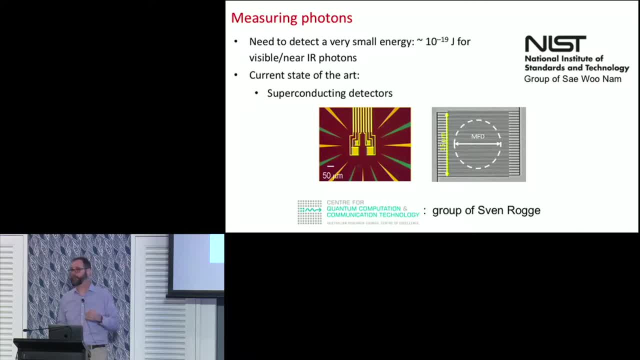 the moment say we makes the highest, the moment say we makes the highest quality ones. nevertheless there's an quality ones. nevertheless there's an quality ones. nevertheless there's an effort here with our own Sven wrong group effort, here with our own Sven wrong group effort, here with our own Sven wrong group, to make very similar nanowire devices. 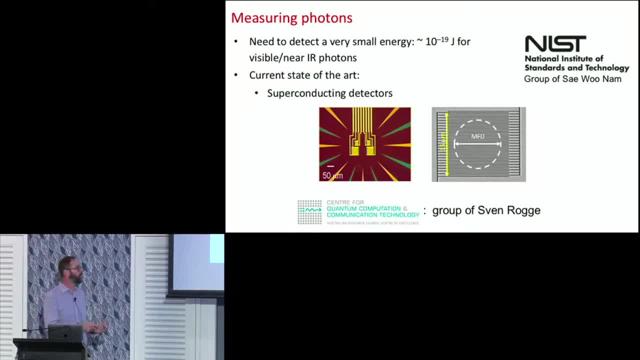 to make very similar nanowire devices. to make very similar nanowire devices not only just the sort of simple basic, not only just the sort of simple basic, not only just the sort of simple basic device here that one then shines an device here that one then shines an. 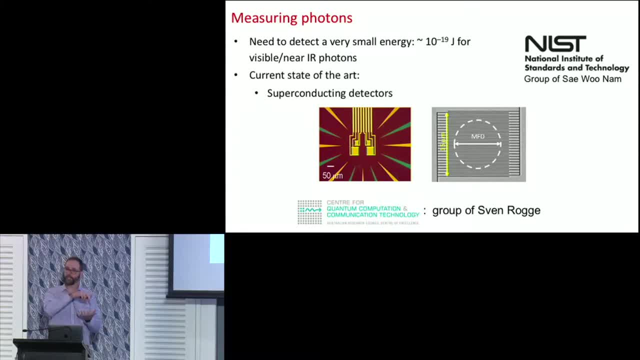 device here, that one then shines an optical fiber. that's what, this white optical fiber, that's what this white optical fiber, that's what this white circle. here is the, the output mode of an circle. here is the- the output mode of an circle. here is the, the output mode of an optical fiber, not only just the basic. 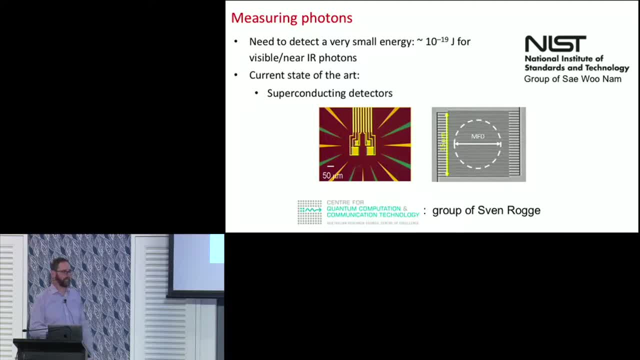 optical fiber, not only just the basic optical fiber, not only just the basic device which you position under an device, which you position under an device, which you position under an optical fiber, but also patterning it on optical fiber. but also patterning it on optical fiber, but also patterning it on top of other different waveguide. 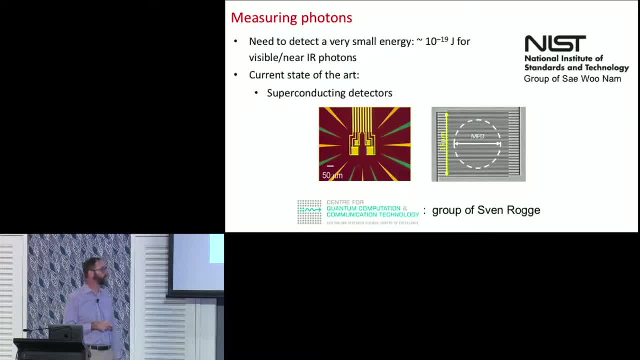 top of other different waveguide, top of other different waveguide structures, and customizable in all sorts structures and customizable in all sorts structures and customizable in all sorts of different ways. all right, so you'll of different ways. all right, so you'll of different ways, all right. so you'll notice that I haven't really said. 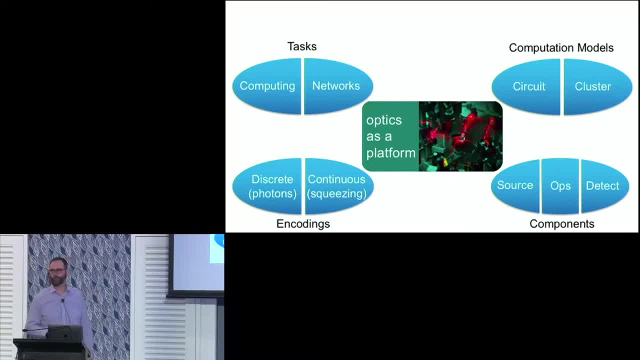 notice that I haven't really said. notice that I haven't really said anything about operations, despite anything about operations, despite anything about operations, despite promising to talk about sources, promising to talk about sources, promising to talk about sources, operations and detectors, and in order to operations and detectors and in order to 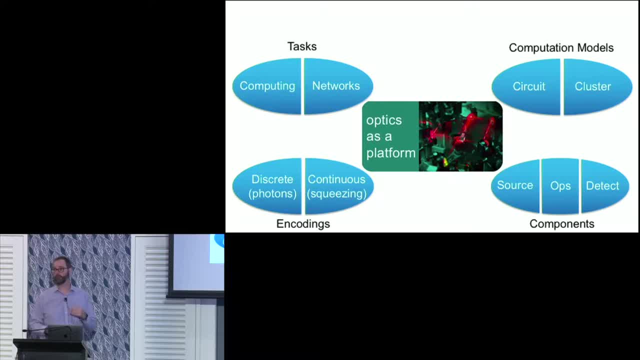 operations and detectors. and in order to do that, I want to say a little bit about do that. I want to say a little bit about do that. I want to say a little bit about computation models. okay, because the way computation models okay, because the way computation models okay because the way the operations are done in optics. 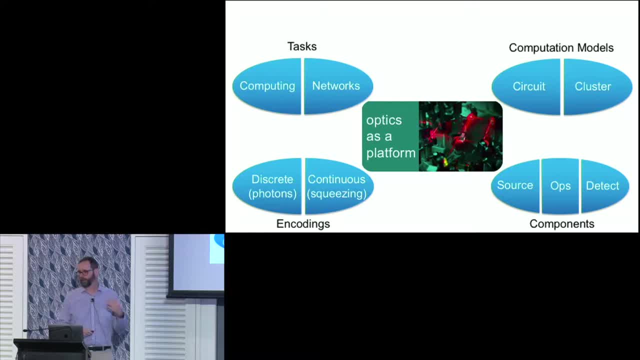 the operations are done in optics. the operations are done in optics depends a little bit on whether you're depends a little bit on whether you're depends a little bit on whether you're thinking about a circuit model or a thinking about a circuit model, or a thinking about a circuit model or a cluster model of quantum computation. 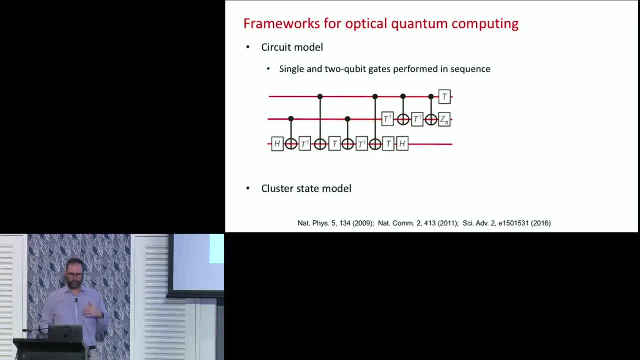 cluster model of quantum computation. cluster model of quantum computation. alright, so the circuit model: we well alright. so the circuit model: we well alright. so the circuit model. we well know. you take some some circuit that you know. you take some some circuit that you know. you take some some circuit that you want to make and you decompose it. 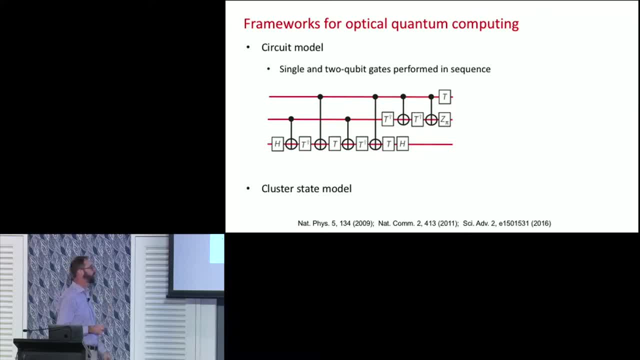 want to make and you decompose it. want to make and you decompose it typically into single qubit and two typically into single qubit and two typically into single qubit and two qubit operations. this is the circuit for qubit operations. this is the circuit for. 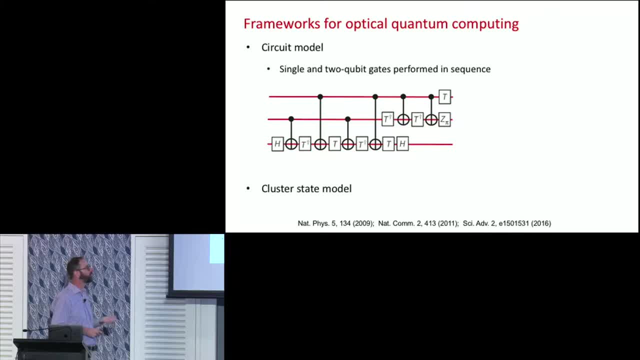 qubit operations. this is the circuit for realizing a Toffoli a three qubit. realizing a Toffoli a three qubit. realizing a Toffoli a three qubit. Toffoli gate, for example: okay, composed. Toffoli gate, for example: okay, composed. 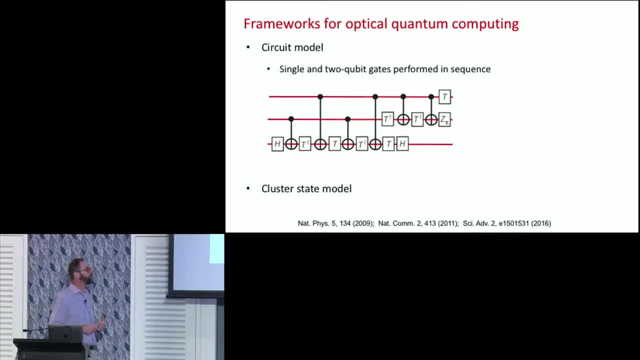 Toffoli gate, for example, okay, composed of single and two qubit operations. okay, of single and two qubit operations. okay, of single and two qubit operations. okay, and you can see that obviously there's, and you can see that obviously there's, and you can see that obviously there's, there's quite a lot of operations to be. 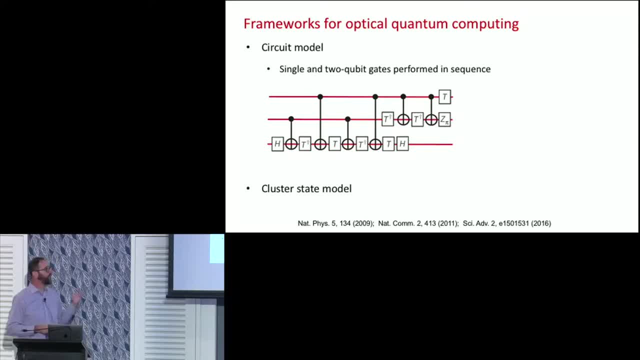 there's quite a lot of operations to be. there's quite a lot of operations to be done here, including a lot of two qubit done here, including a lot of two qubit done here, including a lot of two qubit gates in order to make any decent size. 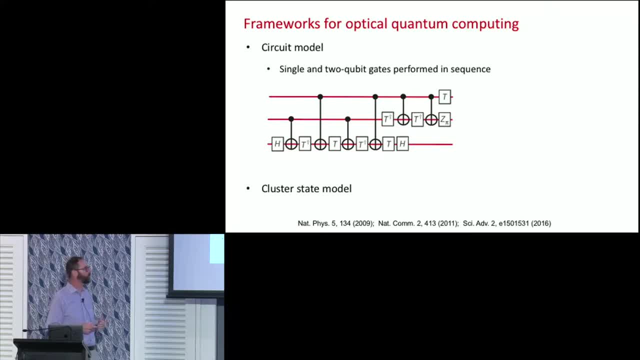 gates in order to make any decent size gates in order to make any decent size circuit. and we saw in Lloyd's talk about circuit and we saw in Lloyd's talk about circuit and we saw in Lloyd's talk about a universal quantum computation that a universal quantum computation, that 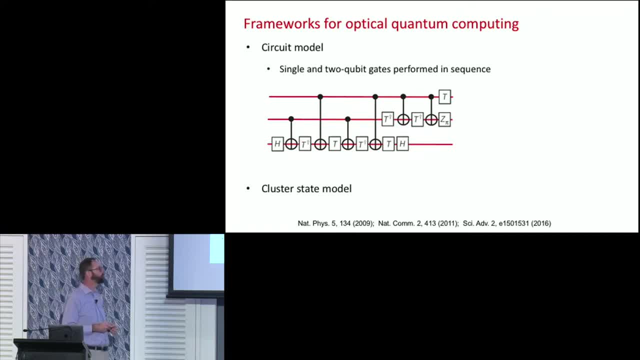 a universal quantum computation, that there are going to be enormous numbers. there are going to be enormous numbers. there are going to be enormous numbers of gates that need to be realized, so in of gates that need to be realized, so in of gates that need to be realized, so in terms of realizing these gates, optics. 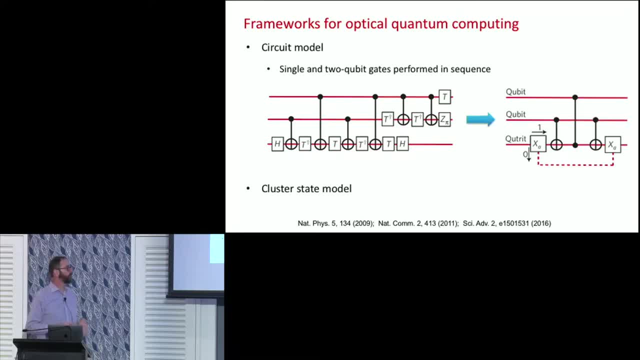 terms of realizing these gates optics. terms of realizing these gates optics has some advantages and some has some advantages and some has some advantages and some disadvantages. okay, one of the advantages disadvantages: okay, one of the advantages disadvantages- okay, one of the advantages is that it's very easy to move in and 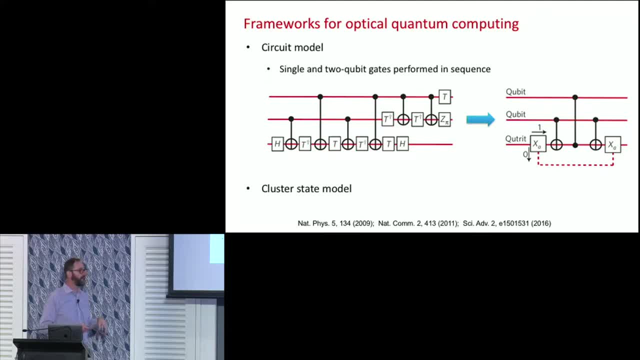 is that it's very easy to move in and is that it's very easy to move in and out of the computational subspace in a, out of the computational subspace in a, out of the computational subspace in a very clean way and to do that in a way. 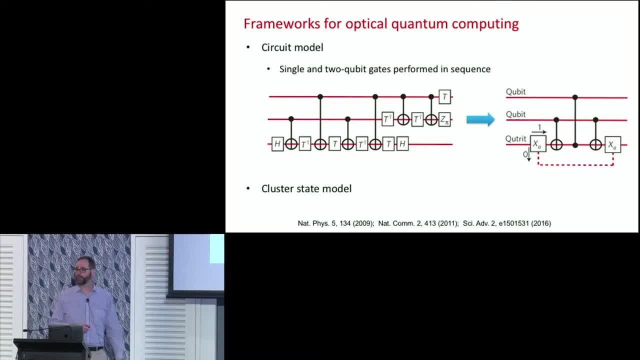 very clean way, and to do that in a way, very clean way, and to do that in a way that allows you to really simplify the, that allows you to really simplify the, that allows you to really simplify the way that you can perform some of these way that you can perform some of these. 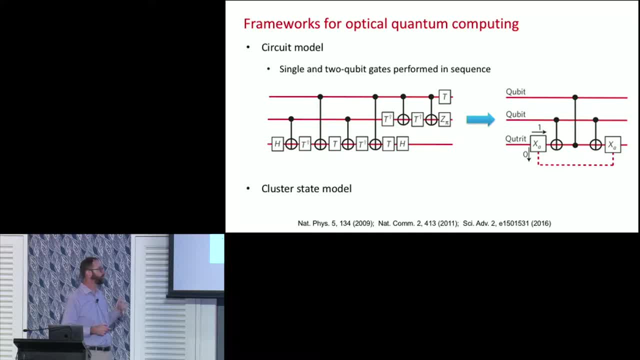 way that you can perform some of these gates. okay, so, some work from Tim Ralph gates. okay, so, some work from Tim Ralph gates. okay, so, some work from Tim Ralph and a number of other collaborators and a number of other collaborators and a number of other collaborators- group at Bristol and others. Andrew. 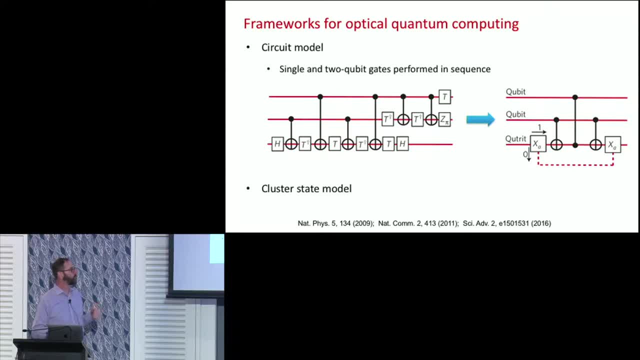 group at Bristol and others. Andrew group at Bristol and others. Andrew White's group has led to. you know White's group has led to. you know White's group has led to. you know techniques for doing exactly this kind techniques for doing exactly this kind techniques for doing exactly this kind of thing, but at the same time as we'll of thing, but at the same time as we'll of thing, but at the same time as we'll see in a moment one of the challenges, see in a moment. one of the challenges, see in a moment, one of the challenges of optics is that doing the two qubit. 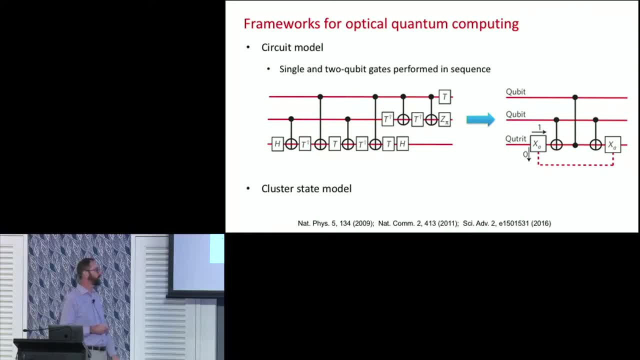 of optics. is that doing the two qubit of optics? is that doing the two qubit gates is hard, although doing one qubit gates is hard, although doing one qubit gates is hard, although doing one qubit gates is easy and they can be done with. 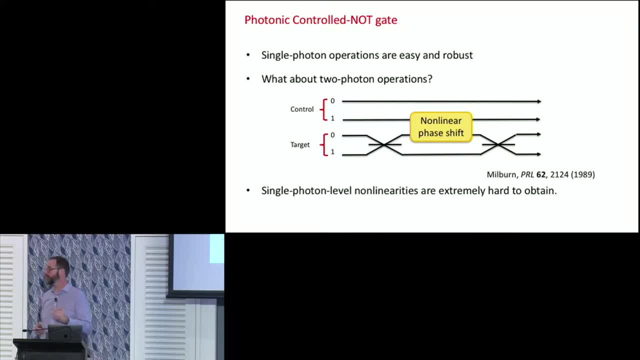 gates is easy and they can be done with. gates is easy and they can be done with high fidelity. okay, so to do a two qubit high fidelity. okay, so to do a two qubit high fidelity. okay, so to do a two qubit gate, for example, a control, not gate. we 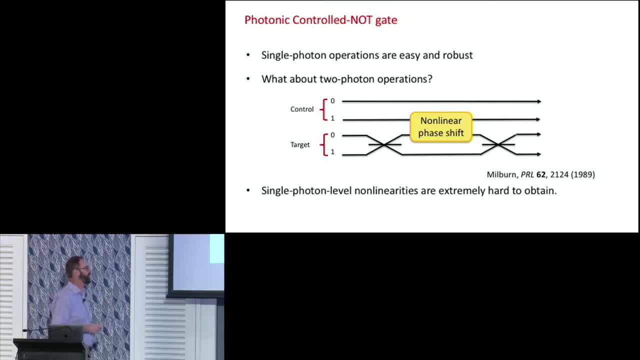 gate, for example, a control, not gate. we gate, for example, a control, not gate. we need to make two photons talk to each. need to make two photons talk to each. need to make two photons talk to each other. two photons interact and I said other two photons interact and I said: 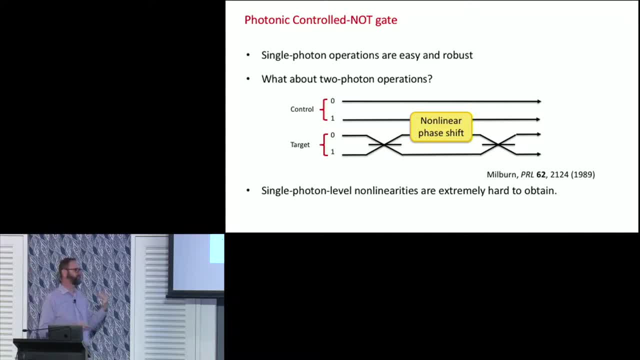 other two photons interact and I said that photons are very low-nose system, that photons are very low-nose system, that photons are very low-nose system because they don't really like to, because they don't really like to, because they don't really like to interact with non-resonant systems and 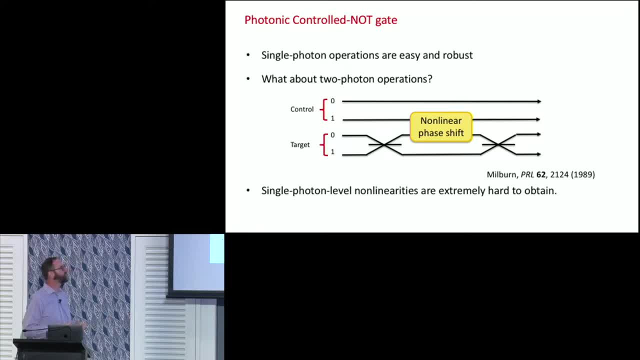 interact with non-resonant systems and interact with non-resonant systems and they certainly don't like to act with, they certainly don't like to act with, they certainly don't like to act with other photons. okay so, single photon. other photons: okay, so, single photon. 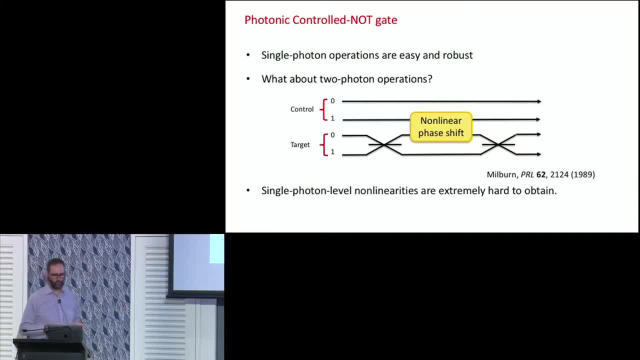 other photons. okay. so single photon operations are easy and robust, not so. operations are easy and robust, not so. operations are easy and robust, not so easy for two photon operations. the basic easy for two photon operations. the basic easy for two photon operations. the basic idea introduced by Jared Milburn is to 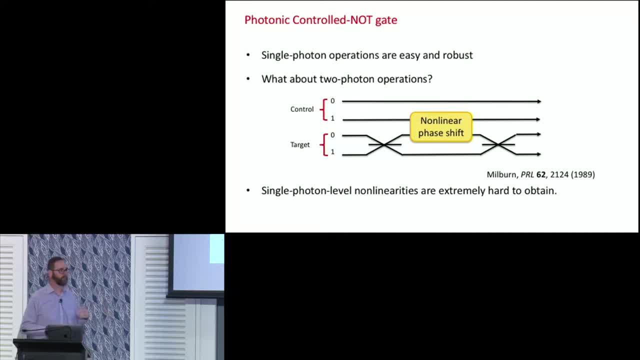 idea introduced by Jared Milburn is to. idea introduced by Jared Milburn is to use some sort of nonlinear phase shift. use some sort of nonlinear phase shift. use some sort of nonlinear phase shift in some nonlinear material. okay, so occur. in some nonlinear material. okay, so occur. 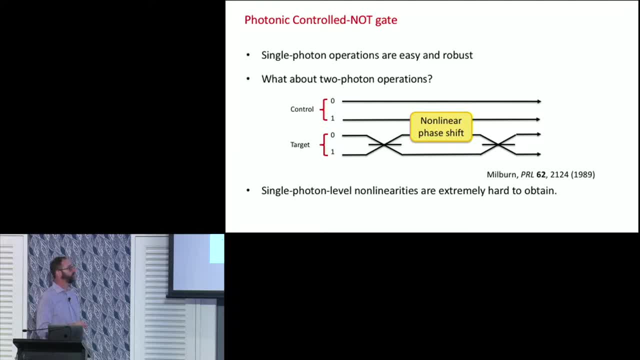 in some nonlinear material. okay, so occur chi-3 nonlinearity, and the idea is: is chi-3 nonlinearity? and the idea is: is chi-3 nonlinearity? and the idea is: is that if both the photons end up in this, that if both the photons end up in this? 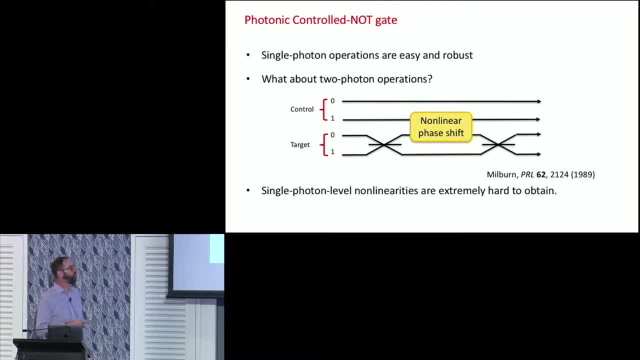 that if both the photons end up in this, in this nonlinear device, so here's, here's in this nonlinear device, so here's, here's in this nonlinear device. so here's, here's a control photon, as we said. it's either a control photon, as we said, it's either. 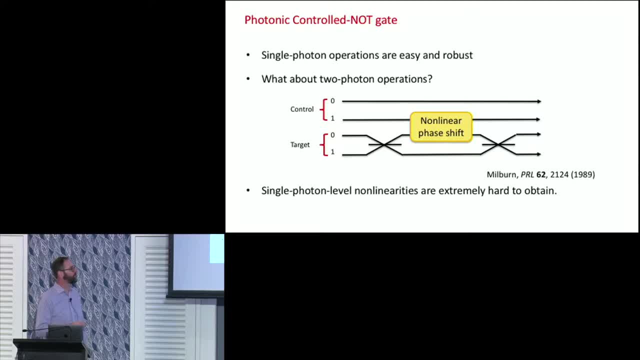 a control photon. as we said, it's either in the top mode or in this mode. is the in the top mode or in this mode? is the in the top mode or in this mode? is the target photon? it it's either in one of target photon it it's either in one of. 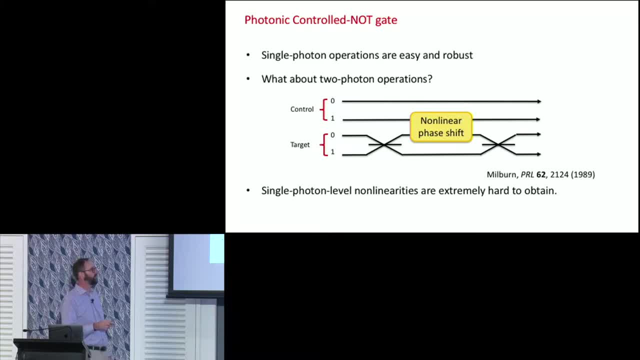 target photon, it, it's either in one of these two modes or, of course, a these two modes or, of course, a these two modes or, of course, a superposition, if the photons both end up superposition. if the photons both end up inside the phase shift, then there's a. 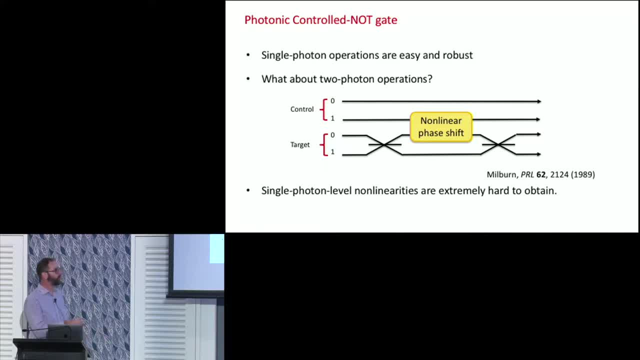 inside the phase shift, then there's a inside the phase shift, then there's a PI phase shift. mutual phase shift between PI phase shift. mutual phase shift between PI phase shift. mutual phase shift between them. the interferometer reads that out them. the interferometer reads that out. 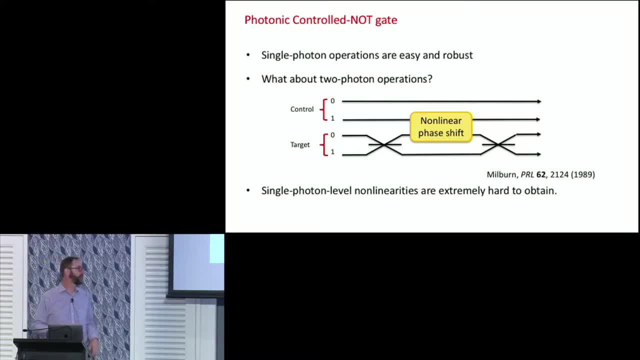 them. the interferometer reads that out and flips the phase of the target qubit and flips the phase of the target qubit and flips the phase of the target qubit at the output. that's how this kind of at the output. that's how this kind of. 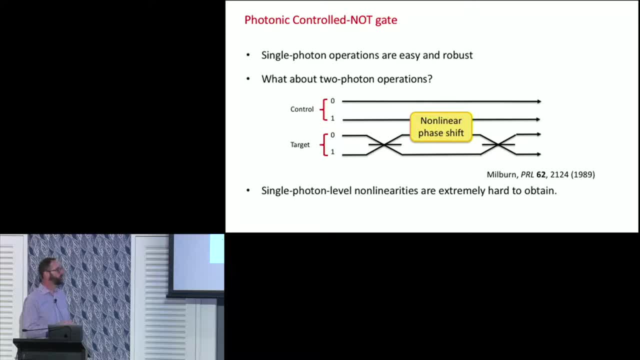 at the output. that's how this kind of CNOT gate would work. okay, but these CNOT gate would work okay, but these CNOT gate would work okay, but these single photon level nonlinearities are single photon level nonlinearities are single photon level. nonlinearities are extremely hard to obtain. that's not to. 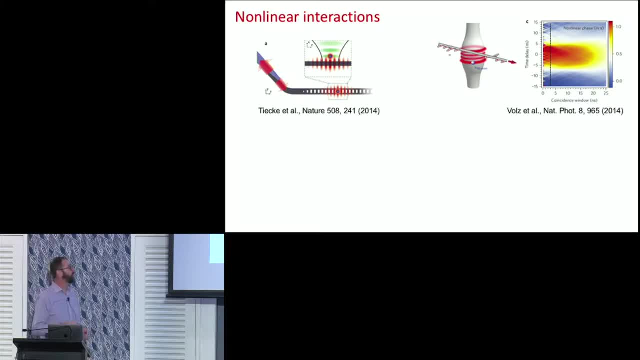 extremely hard to obtain. that's not to extremely hard to obtain. that's not to say that people are not working on this. say that people are not working on this, say that people are not working on this topic and indeed very strong kernel topic and indeed very strong kernel. 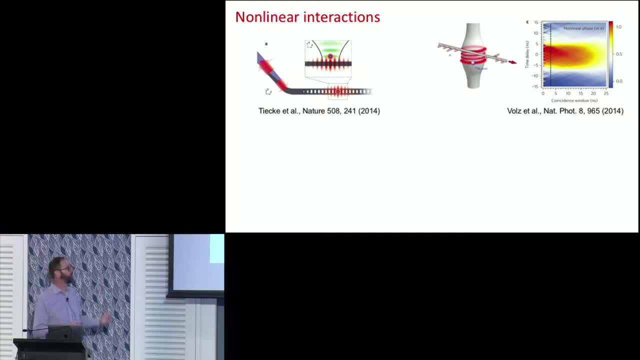 topic and indeed very strong kernel linearities are being achieved in. linearities are being achieved in. linearities are being achieved in resonance systems coupled with with resonance systems coupled with with resonance systems coupled with with cavities. here's a couple of examples. cavities: here's a couple of examples. 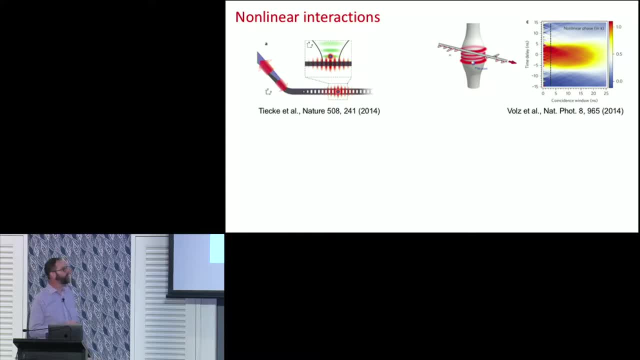 cavities. here's a couple of examples. there's a lot of work going on around. there's a lot of work going on around. there's a lot of work going on around the world on it, but these sort of single the world on it, but these sort of single. 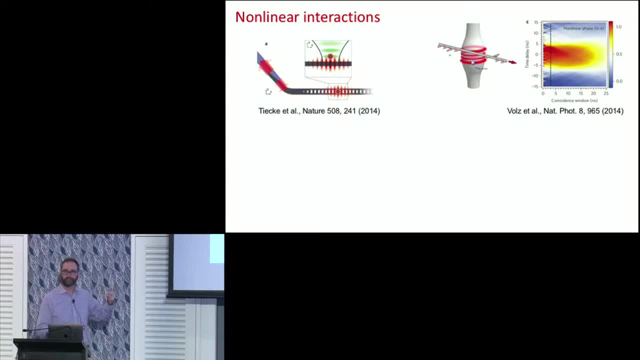 the world on it. but these sort of single system, single single atom or single system single single atom or single system single single atom or single resonant system kind of devices, really resonant system kind of devices, really resonant system, kind of devices really have some outstanding challenges in. 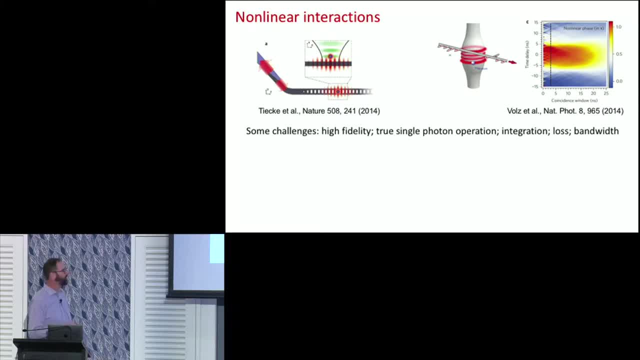 have some outstanding challenges. in have some outstanding challenges in order to become, in order to become you. order to become, in order to become you, order to become, in order to become: you know robust, long-term technology. one know robust, long-term technology. one know robust, long-term technology. one needs to see higher fidelity operation. 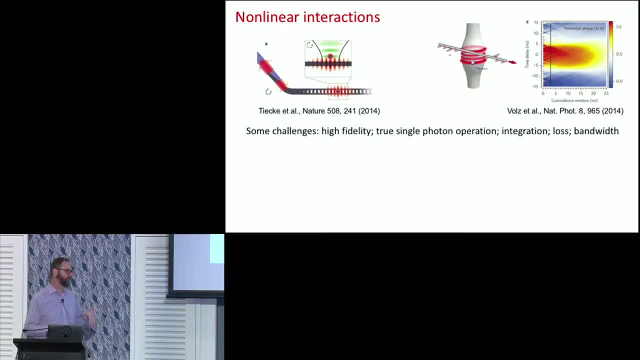 needs to see higher fidelity operation, needs to see higher fidelity operation, true single photon operation, and then true single photon operation, and then true single photon operation, and then there are questions about integration. there are questions about integration, there are questions about integration loss and bandwidth, and so on. perhaps. 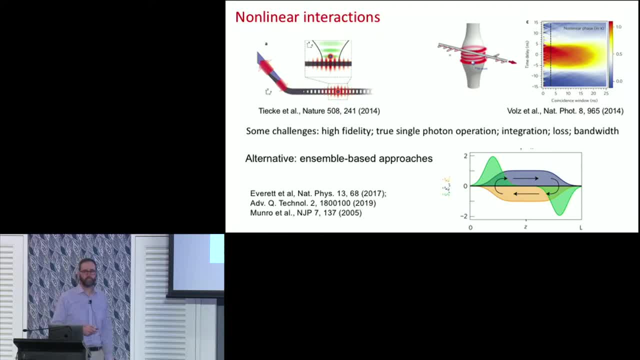 loss and bandwidth and so on. perhaps loss and bandwidth and so on, perhaps solvable, but, but it's not solvable, but, but it's not solvable, but, but it's not straightforward. an alternative is to use straightforward. an alternative is to use straightforward. an alternative is to use an ensemble based approach, and this is 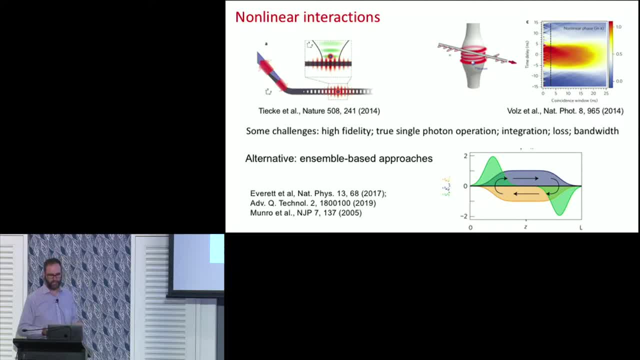 an ensemble based approach, and this is an ensemble based approach and this is something that Ben Buchla's group is, something that Ben Buchla's group is something that Ben Buchla's group is looking at here in CQC to T. the idea is looking at here in CQC to T. the idea is: 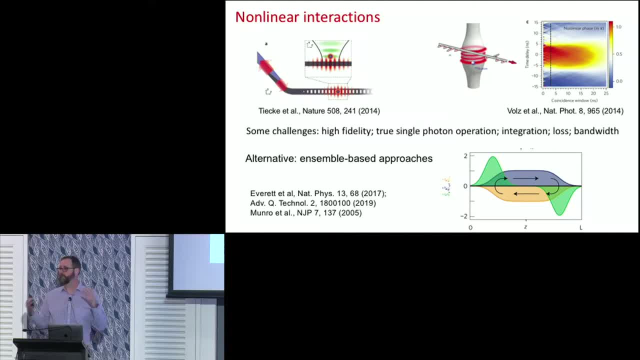 looking at here in CQC to T. the idea is to have some sort of spin wave, which is to have some sort of spin wave which is to have some sort of spin wave, which is what's depicted here in stored in some, what's depicted here in stored in some. 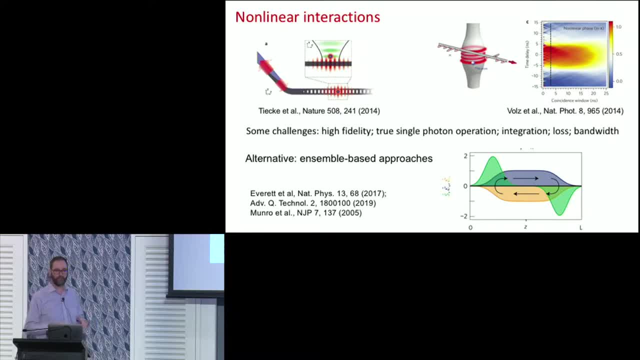 what's depicted here in stored in some atomic medium, some ensemble atomic atomic medium, some ensemble atomic atomic medium, some ensemble atomic medium, and then using the slow light or medium. and then using the slow light or medium, and then using the slow light or the stop light, the stationary light based. 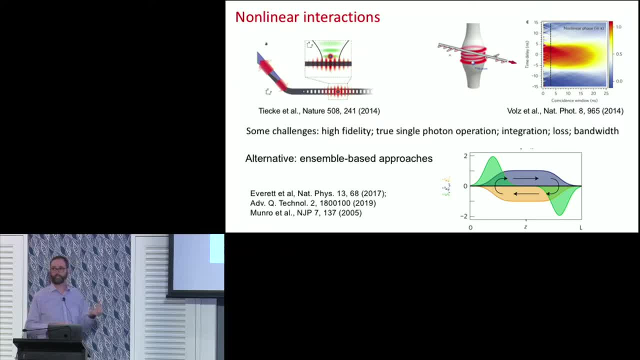 the stop light, the stationary light, based on that, to achieve a small nonlinear on that, to achieve a small nonlinear on that, to achieve a small nonlinear phase shift which can then be sort of phase shift, which can then be sort of phase shift, which can then be sort of amplified up, if you will, using theory. 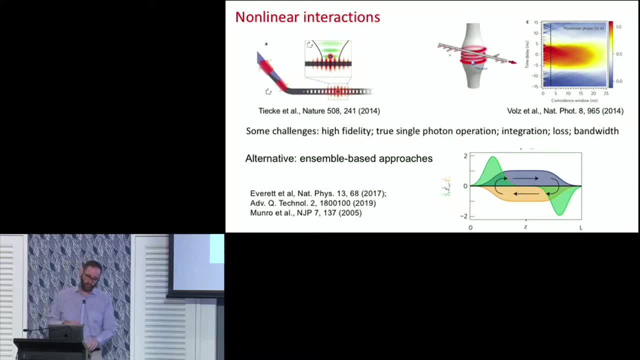 amplified up, if you will, using theory. amplified up, if you will, using theory, techniques that have been proposed. techniques that have been proposed, techniques that have been proposed previously. so nonlinear interactions are previously so. nonlinear interactions are previously so. nonlinear interactions are one way to try to achieve photonic. 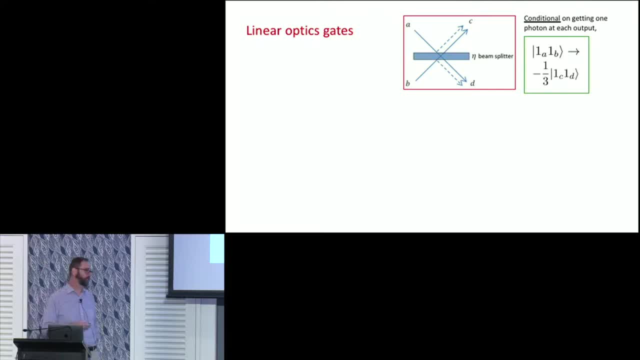 one way to try to achieve photonic, one way to try to achieve photonic: quantum computing, or indeed that also quantum computing, or indeed that also quantum computing, or indeed that also can apply to continuous variables, can apply to continuous variables, can apply to continuous variables approaches as well. but another way is to 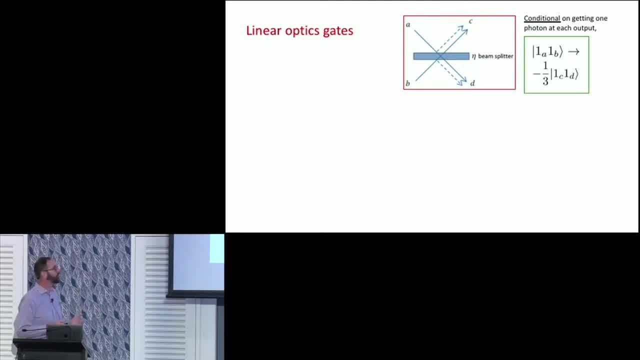 approaches as well. but another way is to approaches as well, but another way is to think about using linear optics gates. think about using linear optics gates. think about using linear optics gates. okay, and the idea here is is sort of okay, and the idea here is is sort of. 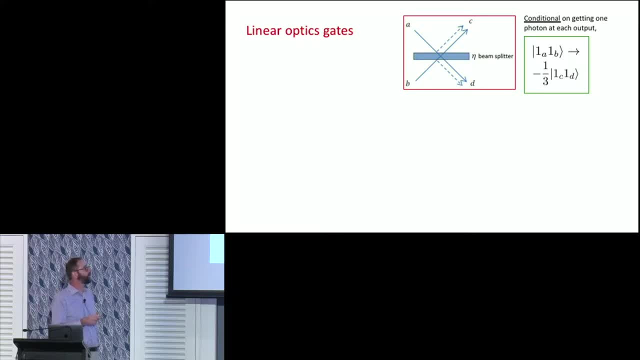 okay, and the idea here is is sort of something roughly like this: if you something roughly like this, if you something roughly like this, if you interfere two photons on a suitably interfere two photons on a suitably interfere two photons on a suitably chosen beam splitter, then 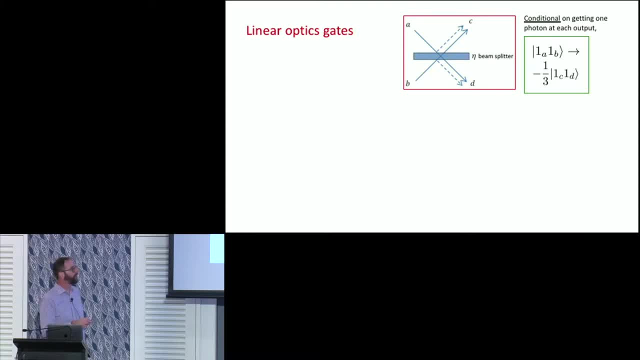 chosen beam splitter, then chosen beam splitter, then non-deterministically, but with some non-deterministically but with some non-deterministically but with some probability there can be a phase shift. probability there can be a phase shift. probability there can be a phase shift. that appears a pie phase shift, exactly. 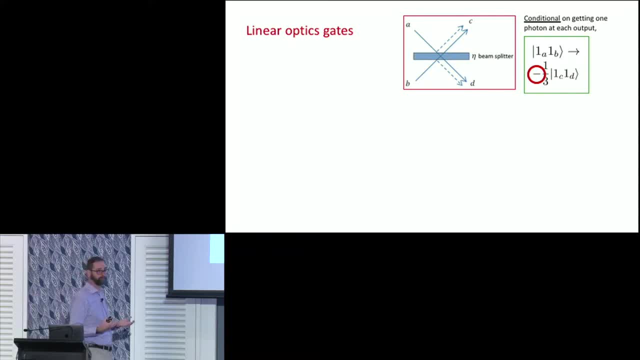 that appears a pie phase shift. exactly that appears a pie phase shift. exactly like you would have in a in one of. like you would have in a in one of these occur gates. okay, so that's what the these occur gates. okay, so that's what the these occur gates. okay, so that's what the minus sign depicts, but the one-third. 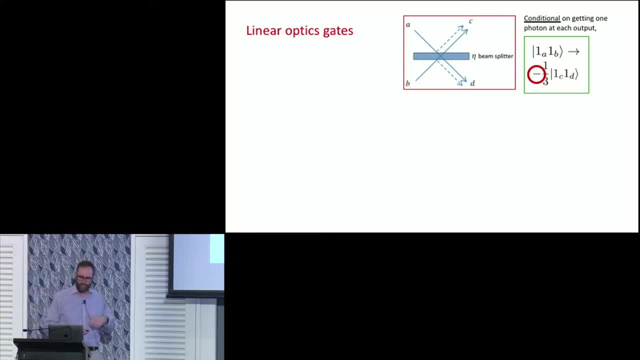 minus sign depicts. but the one-third minus sign depicts. but the one-third pre-factor here depicts that this is a pre-factor here. depicts that this is a pre-factor here. depicts that this is a non-deterministic process. that by itself non-deterministic process. that by itself. 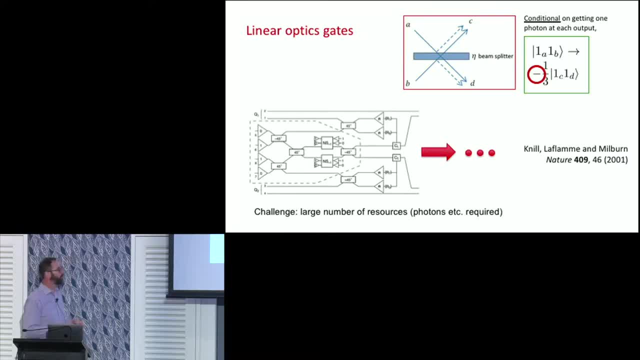 non-deterministic process. that by itself isn't a showstopper. canila flama isn't a showstopper. canila flama isn't a showstopper. canila flama- Milburn showed how to integrate these. Milburn showed how to integrate these. 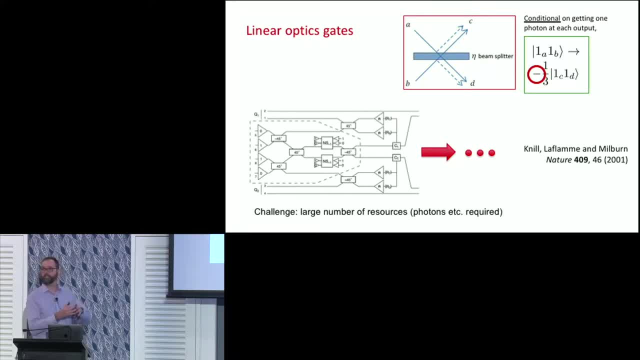 Milburn showed how to integrate these kinds of beam splitters into some of kinds of beam splitters, into some of kinds of beam splitters, into some of these devices here, which then get these devices here, which then get these devices here, which then get concatenated up into larger circuits and 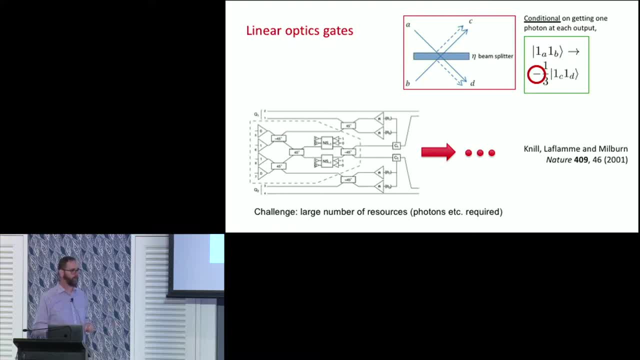 concatenated up into larger circuits and concatenated up into larger circuits. and you keep going and keep going and you keep going and keep going and you keep going and keep going, and eventually you have something that's eventually. you have something that's eventually. you have something that's very close to a deterministic gate. but 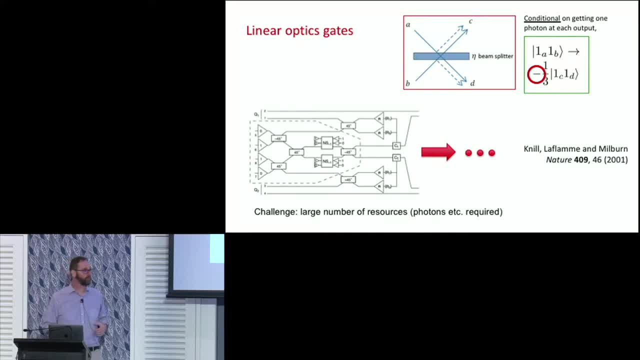 very close to a deterministic gate, but very close to a deterministic gate. but the challenge is that a large number of the challenge is that a large number of the challenge is that a large number of resources like photons and components, resources like photons and components, resources like photons and components, are required, even though it scales. 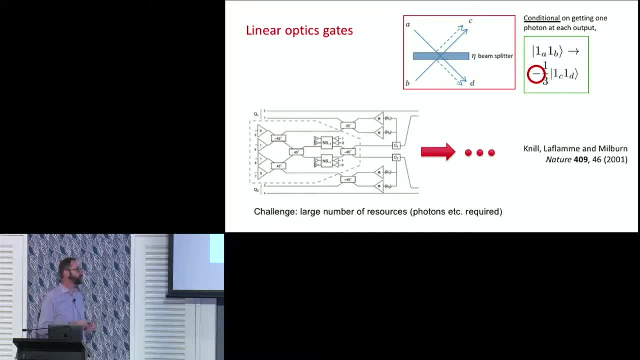 are required. even though it scales are required. even though it scales linearly with the number of qubits, it's linearly with the number of qubits. it's linearly with the number of qubits. it's it's still a significant overhead. it's still a significant overhead. 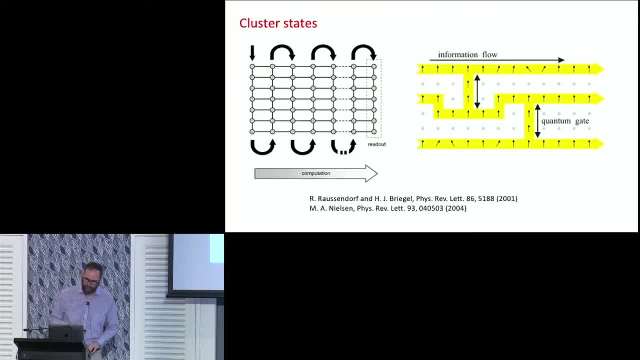 it's still a significant overhead, although theory has brought that down, although theory has brought that down, although theory has brought that down over the years. an alternative is to over the years. an alternative is to over the years. an alternative is to consider a cluster state model, now in a 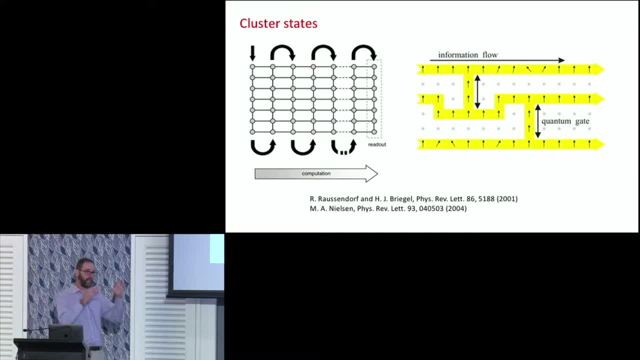 consider a cluster state model now in a. consider a cluster state model now in a cluster state. what we're thinking about cluster state, what we're thinking about cluster state. what we're thinking about is constructing a large entangled state. is constructing a large entangled state. 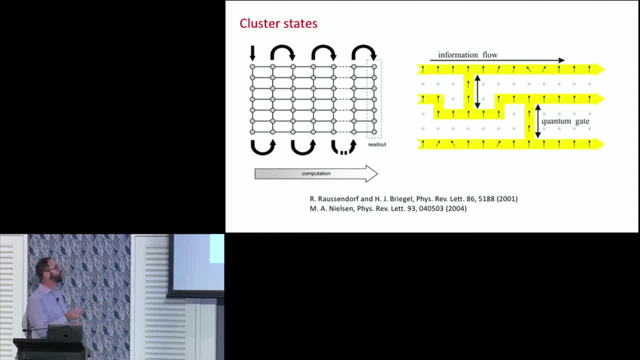 is constructing a large entangled state offline, if you will, or before the offline, if you will, or before the offline, if you will, or before the computation. so something like this: here's computation. so something like this, here's computation. so something like this: here's a two-dimensional version. so this grid, 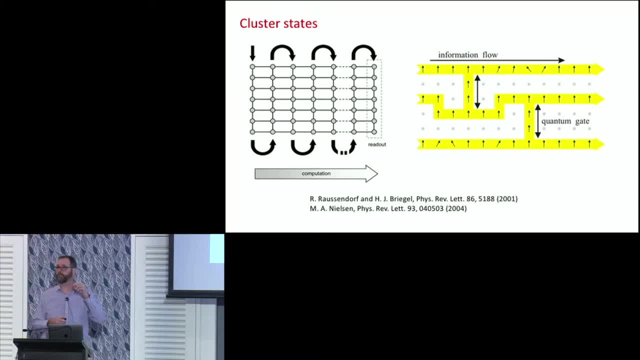 a two-dimensional version. so this grid, a two-dimensional version. so this grid: each of the nodes is a qubit and the each of the nodes is a qubit and the each of the nodes is a qubit and the lines between them indicate an lines between them indicate an. 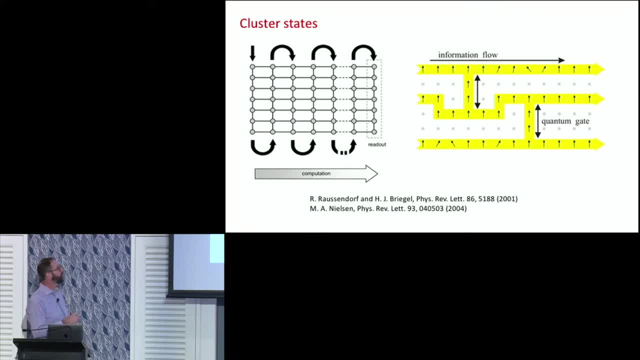 lines between them indicate an entangling operation. so these qubits are entangling operation. so these qubits are entangling operation. so these qubits are entangled to their neighbors. so one one entangled to their neighbors. so one one entangled to their neighbors. so one one creates such a 2d or 3d cluster and then 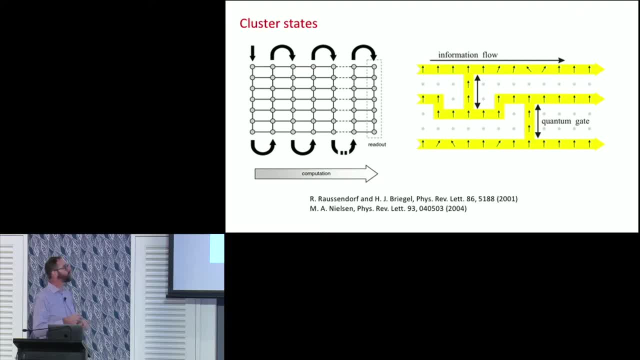 creates such a 2d or 3d cluster and then creates such a 2d or 3d cluster and then performs a sort of- I guess sequences of, performs a sort of I guess sequences of performs a sort of, I guess, sequences of operations on the planes of qubits. 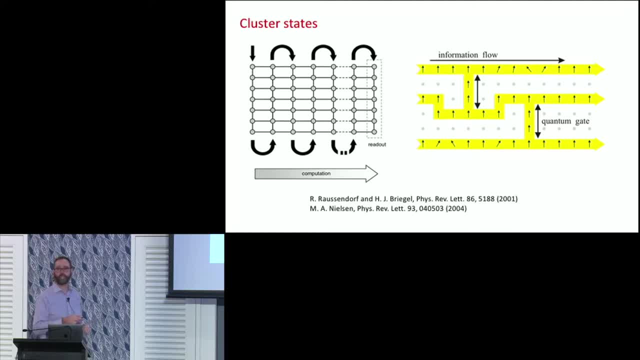 operations on the planes of qubits through this device and feeds forward through this device. and feeds forward through this device. and feeds forward the measurement result to the next step. the measurement result to the next step, the measurement result to the next step. and and by choosing the measurements, and and by choosing the measurements and and by choosing the measurements that are made, the basis in which they're that are made, the basis in which they're that are made, the basis in which they're made, and these feed forward operations made and these feed forward operations. 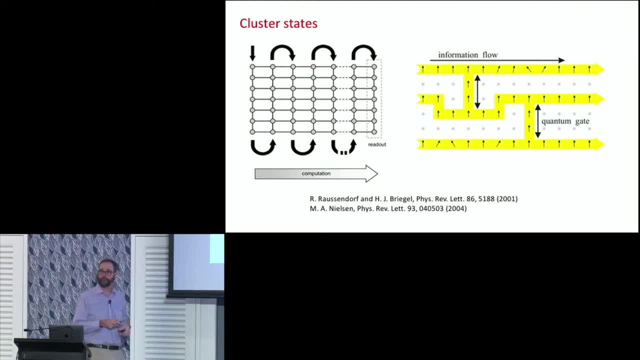 made and these feed forward operations. one can essentially carve out a path, for one can essentially carve out a path, for one can essentially carve out a path for the information through this kind of the information, through this kind of the information, through this kind of system, which is equivalent to performing. 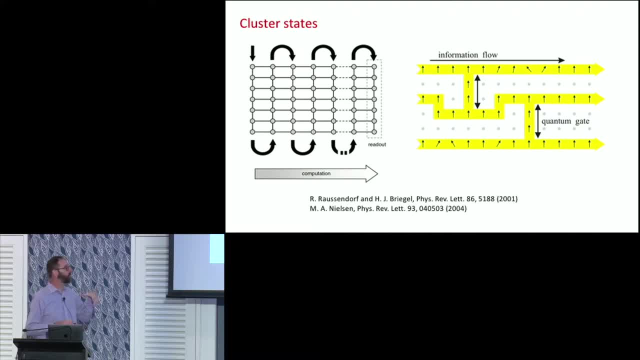 system which is equivalent to performing system which is equivalent to performing quantum computation in a circuit model, quantum computation in a circuit model. quantum computation in a circuit model. this is sometimes called a one-way. this is sometimes called a one-way. this is sometimes called a one-way quantum computer because the 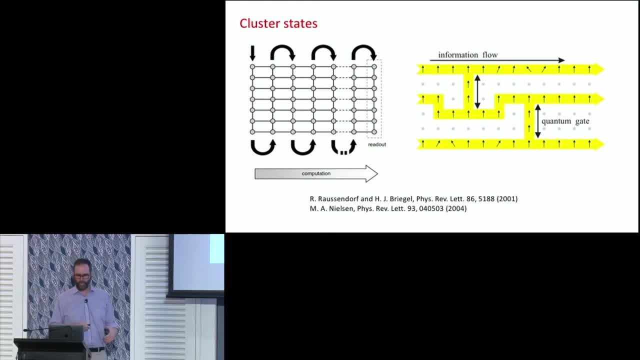 quantum computer, because the quantum computer, because the entanglement resource is consumed as you, entanglement resource is consumed as you, entanglement resource is consumed as you make the measurements. but the nice thing: make the measurements. but the nice thing, make the measurements. but the nice thing about it is that, although establishing 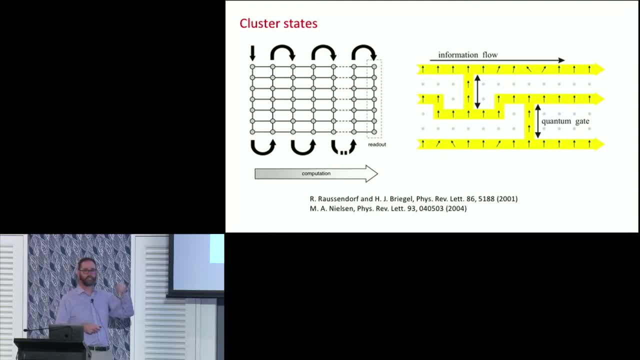 about it is that, although establishing about it is that, although establishing this cluster requires entangling, this cluster requires entangling, this cluster requires entangling operations of the same kind of a operations of the same kind of a operations of the same kind of a CNOT gate, this can be done, sort of 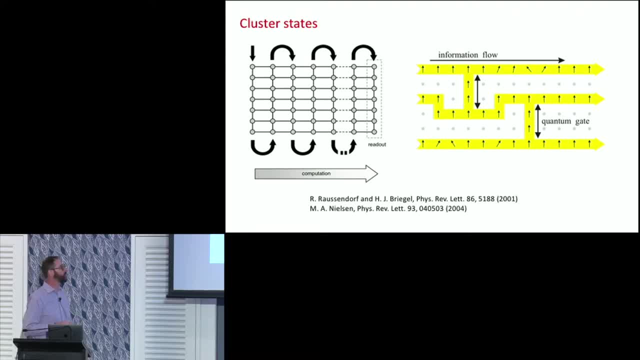 CNOT gate. this can be done sort of CNOT gate. this can be done sort of offline, if you will, and then that's a offline, if you will, and then that's a offline, if you will, and then that's a resource that can then be used and the 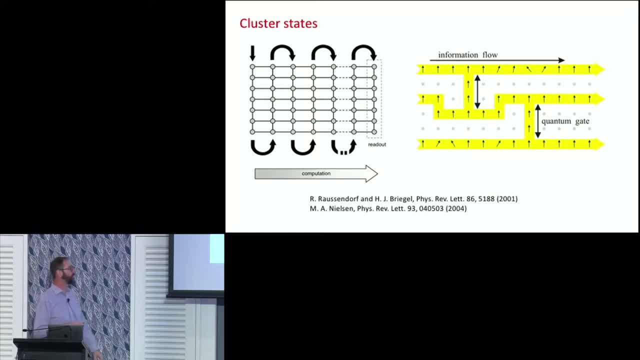 resource that can then be used and the resource that can then be used, and the single qubit operations and measurements, single qubit operations and measurements, single qubit operations and measurements, which, as we said, are incredibly high, which, as we said, are incredibly high, which, as we said, are incredibly high fidelity and high performance can be. 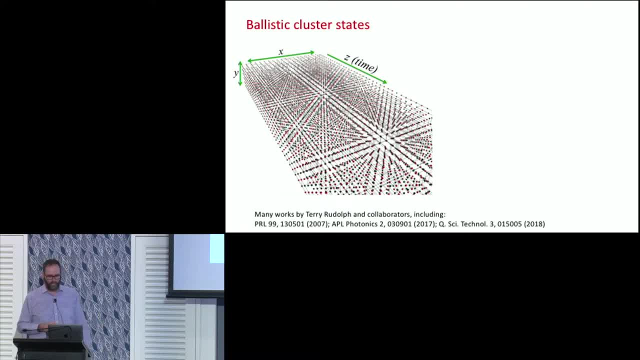 fidelity and high performance can be. fidelity and high performance can be used to process the information, so used to process the information, so used to process the information. so there's a bunch of work by Terry Rudolph. there's a bunch of work by Terry Rudolph. there's a bunch of work by Terry Rudolph and many collaborators over the years. 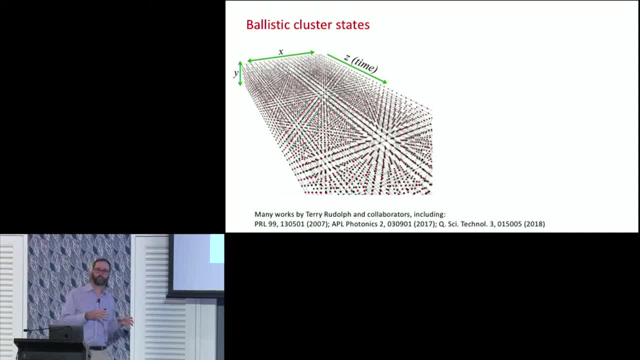 and many collaborators over the years, and many collaborators over the years, which is looking at how one can do, which is looking at how one can do, which is looking at how one can do ballistic quantum computing. so not even ballistic quantum computing. so not even ballistic quantum computing, so not even requiring memory in a scheme that uses 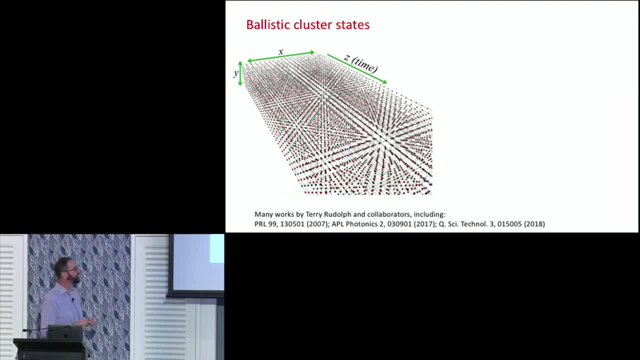 requiring memory in a scheme that uses requiring memory, in a scheme that uses these kinds of clusters. so here's an these kinds of clusters. so here's an these kinds of clusters. so here's an example of a 3d cluster that one might, example of a 3d cluster that one might. 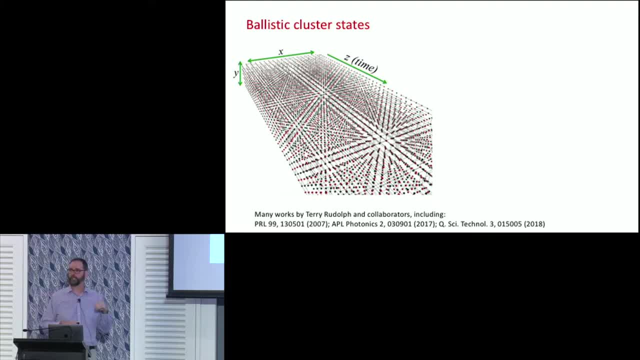 example of a 3d cluster that one might make this cluster may in fact even have make this cluster may in fact even have make this cluster may in fact even have some imperfections in it and there are some imperfections in it, and there are some imperfections in it and there are techniques for dealing with those. 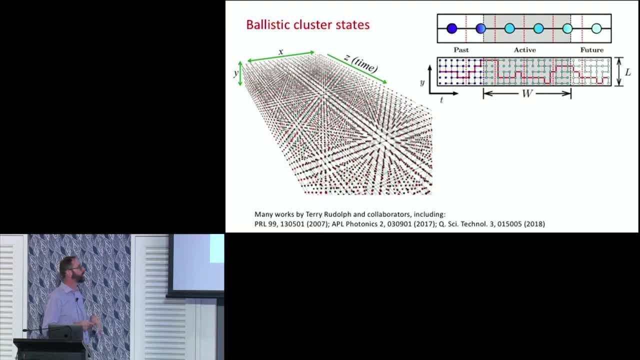 techniques for dealing with those techniques for dealing with those imperfections using percolation theory, imperfections using percolation theory, imperfections using percolation theory, and so on. but the idea if we think about and so on, but the idea if we think about, 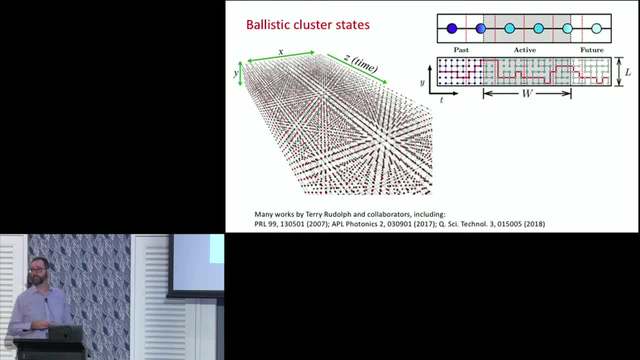 and so on, but the idea, if we think about a 2d cluster, the idea is sort of a 2d cluster, the idea is sort of a 2d cluster. the idea is sort of something like this: the cluster doesn't. something like this: the cluster doesn't. 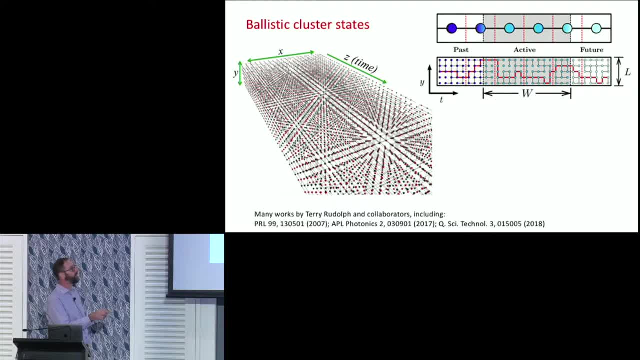 something like this: the cluster doesn't even have to all exist at the same time, even have to all exist at the same time, even have to all exist at the same time. there can be some parts of the cluster, there can be some parts of the cluster, there can be some parts of the cluster cluster. so here, here at the end, that 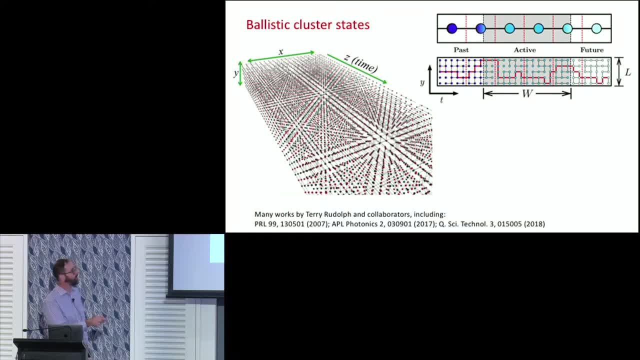 cluster, so here here at the end, that cluster, so here here at the end, that have been measured already and consumed, have been measured already and consumed, have been measured already and consumed. there's some cluster that exists at the. there's some cluster that exists at the. there's some cluster that exists at the moment and that you know measurements. 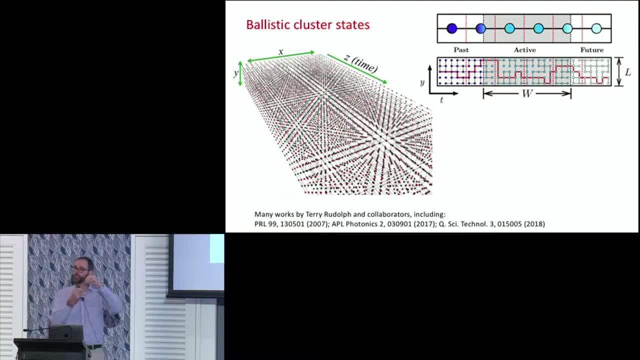 moment, and that you know measurements moment, and that you know measurements are about to be made on, and here's the are about to be made on and here's the are about to be made on. and here's the future cluster, so there are sources. future cluster, so there are sources. 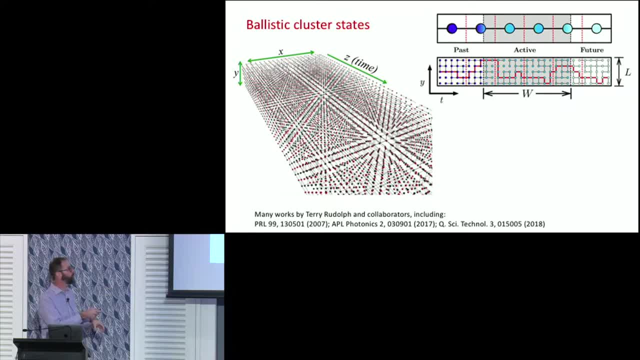 future cluster. so there are sources making entangled photons and building on making entangled photons and building on making entangled photons and building on to the back end of the cluster, even as to the back end of the cluster, even as to the back end of the cluster, even as the front end is being being measured, and 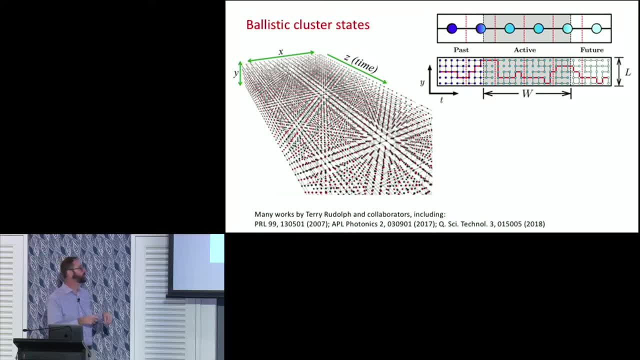 the front end is being being measured, and the front end is being being measured and consumed, and so there are open consumed, and so there are open consumed, and so there are open theoretical questions about what theoretical questions, about what theoretical questions, about what dimensions need to exist in this active. 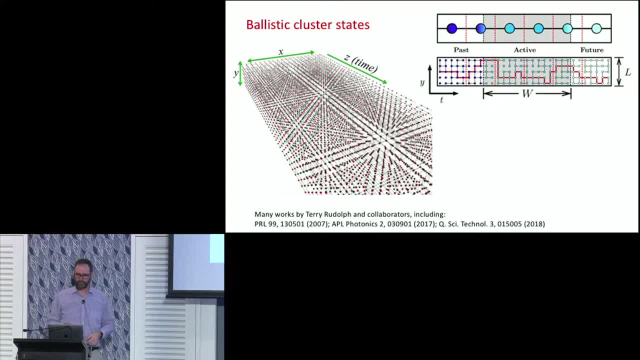 dimensions need to exist in this active dimensions need to exist in this active zone: the length, the breadth, the depth. if zone the length, the breadth, the depth, if zone the length, the breadth, the depth, if you will, but it seems like it's not, you will, but it seems like it's not. 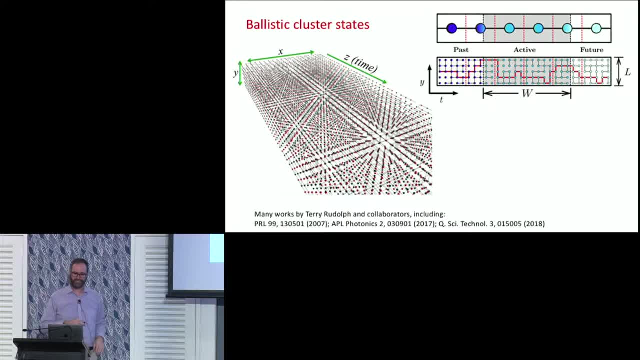 you will, but it seems like it's not outrageously huge. one of the things I outrageously huge, one of the things I outrageously huge, one of the things I should just mention is that, of course a should just mention. is that of course a should just mention? is that, of course, a lot of the theorists who've worked on 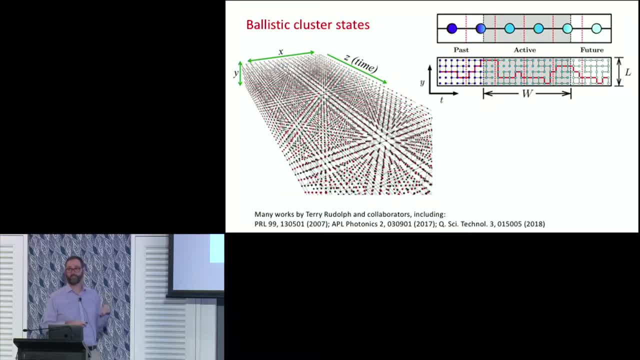 lot of the theorists who've worked on, lot of the theorists who've worked on this are now tied up with the Psi. this are now tied up with the Psi. this are now tied up with the Psi- quantum company, and so be interesting to quantum company and so be interesting to. 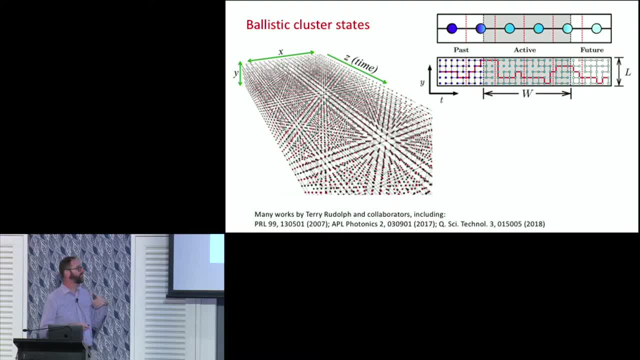 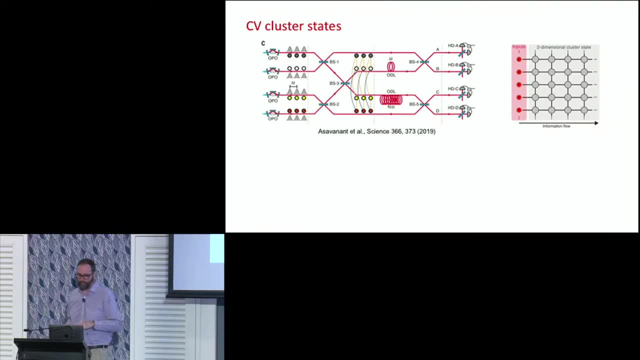 quantum company, and so be interesting to see going forwards. how much of that, see going forwards. how much of that, see going forwards, how much of that, those, those theoretically develop, those, those theoretically develop, those, those theoretically develop, theoretical developments are publicly theoretical developments are publicly theoretical developments are publicly released. okay, so in our Center, one of 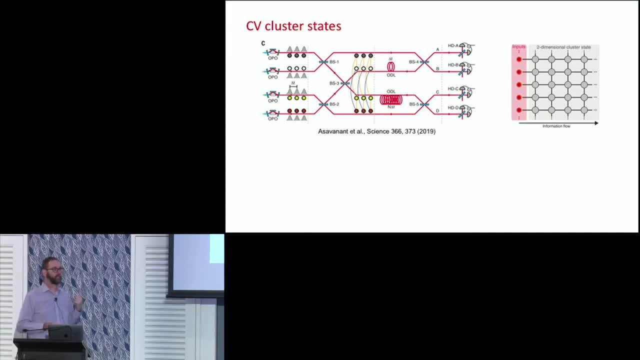 released. okay so in our Center, one of released. okay, so in our Center, one of the things that were particularly the things that were particularly the things that were particularly actively pursuing is the cluster state actively pursuing. is the cluster state actively pursuing is the cluster state scheme for continuous variables? okay, so, 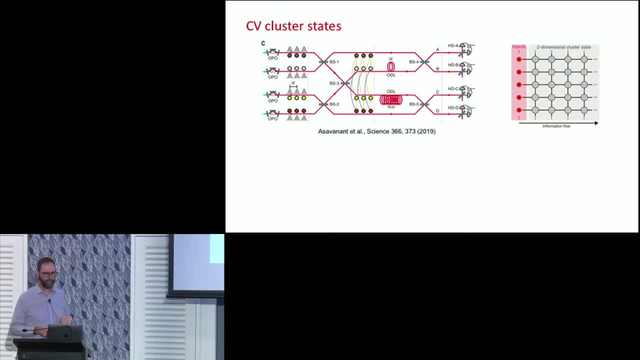 scheme for continuous variables: okay. so, scheme for continuous variables: okay. so there's a lot of theory work being done. there's a lot of theory work being done. there's a lot of theory work being done by Nick Manicucci and collaborators, and by Nick Manicucci and collaborators, and 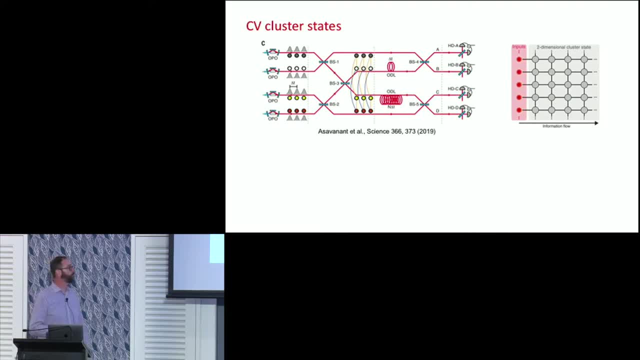 by Nick Manicucci and collaborators, and our partners, such as Akira Furusawa's. our partners such as Akira Furusawa's. our partners such as Akira Furusawa's group at Tokyo and Olivia Fister's group group at Tokyo and Olivia Fister's group. 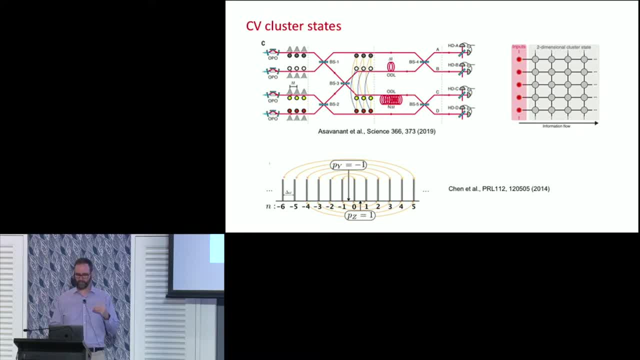 group at Tokyo and Olivia Fister's group at Virginia working on making these kinds at Virginia, working on making these kinds at Virginia, working on making these kinds of devices and have demonstrated 1d and of devices and have demonstrated 1d and of devices and have demonstrated 1d and 2d clusters in frequency encodings and. 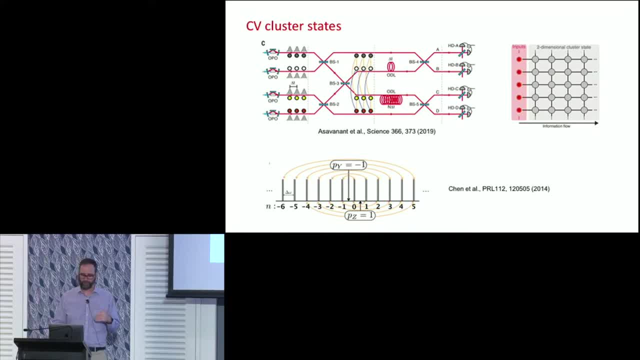 2d clusters in frequency encodings and 2d clusters in frequency encodings and in temporal encodings, with very large in temporal encodings, with very large in temporal encodings, with very large cluster sizes. okay, so, let me say just a cluster sizes. okay, so, let me say just a. 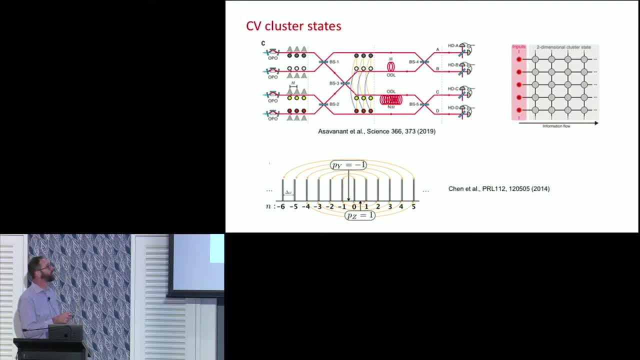 cluster sizes. okay, so let me say just a little bit about the temporal encoding. little bit about the temporal encoding, little bit about the temporal encoding. here we have some, some some different. here we have some some some different. here we have some some some different pulses of squeezed light coming from. 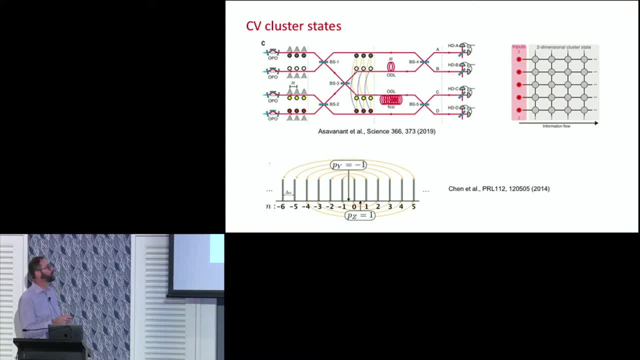 pulses of squeezed light coming from pulses of squeezed light coming from these parametric oscillators. they're these parametric oscillators. they're these parametric oscillators. they're mixed on a beam splitter which, as I said, mixed on a beam splitter which, as I said, 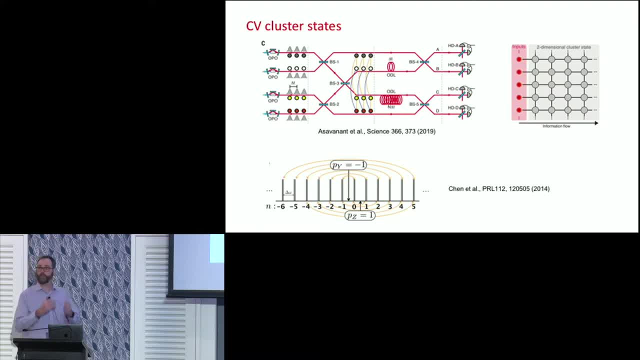 mixed on a beam splitter which, as I said, gives you some entanglement. there's gives you some entanglement. there's gives you some entanglement. there's some delay lines here which allow you to some delay lines here which allow you to some delay lines here which allow you to basically take these entangled modes. 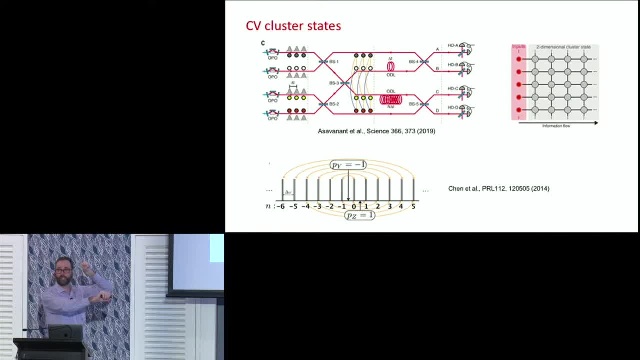 basically take these entangled modes. basically take these entangled modes, these entangled squeezed modes, and to these entangled squeezed modes and to these entangled squeezed modes and to to shift them temporally in time and then to shift them temporally in time and then. 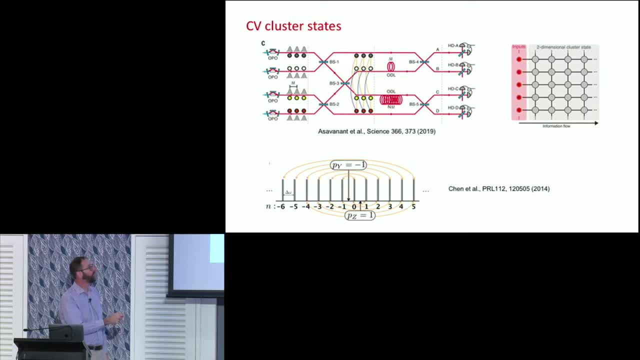 to shift them temporally in time, and then to interfere them again with the, to interfere them again with the, to interfere them again with the next one along, and then one builds up a next one along, and then one builds up a next one along, and then one builds up a kind of cluster state where the lines 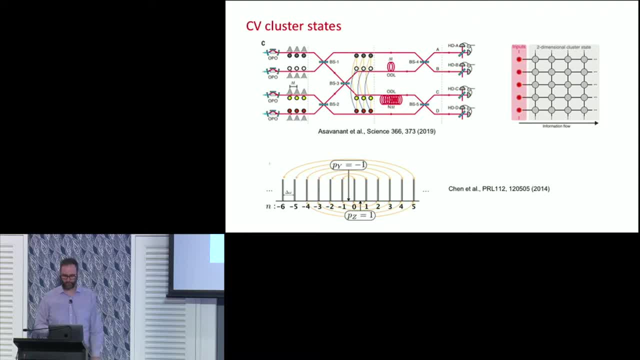 kind of cluster state where the lines kind of cluster state where the lines here show the linkages and it can be here show the linkages and it can be here show the linkages. and it can be mapped onto a, in this case a 2d cluster. 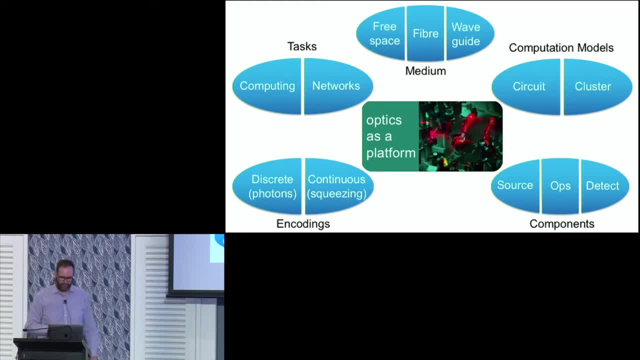 mapped onto a- in this case, a 2d cluster. mapped onto a- in this case, a 2d cluster. okay, so, this is all very nice, but how? okay, so, this is all very nice, but how are we going to realize all of this? are we going to realize all of this? 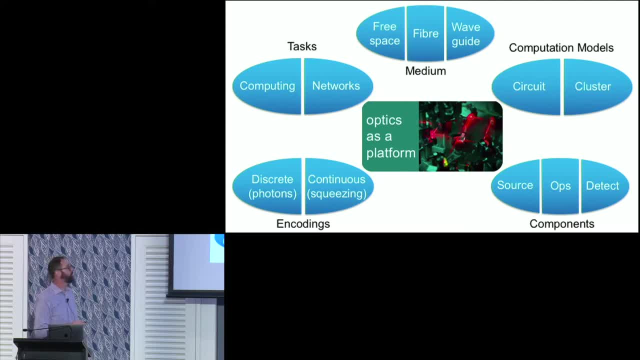 are we going to realize all of this? we've sort of shown different media, or we've sort of shown different media, or we've sort of shown different media or platforms for doing it, and so I want to platforms for doing it, and so I want to platforms for doing it, and so I want to say a little bit about the three. 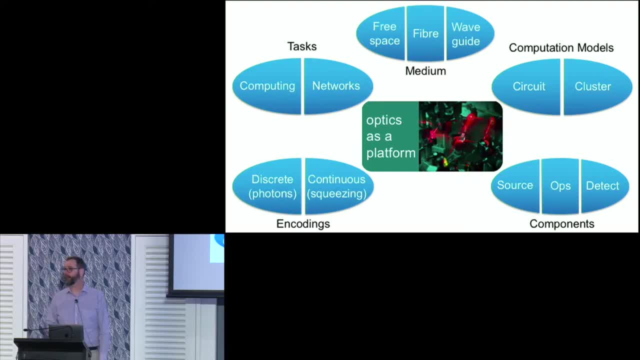 say a little bit about the three, say a little bit about the three techniques that one might use, free techniques. that one might use free techniques, that one might use free space, fiber and wave guide. I'm not space, fiber and wave guide. I'm not space, fiber and wave guide. I'm not really going to say much about fiber. 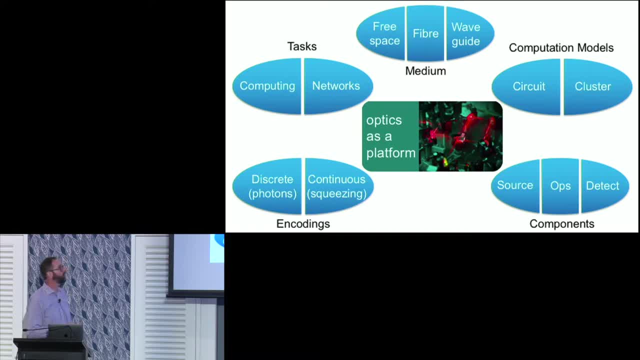 really going to say much about fiber, really going to say much about fiber because I'm not saying much about, because I'm not saying much about, because I'm not saying much about networking. but let's talk about the networking. but let's talk about the networking, but let's talk about the other two. okay, so this is an example of 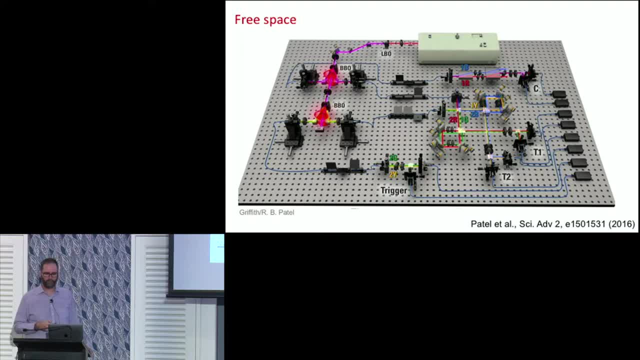 other two. okay, so this is an example of other two. okay, so this is an example of a typical: you know few qubit linear. a typical: you know few qubit linear. a typical: you know few qubit linear. optics, quantum computing experiment. okay, optics, quantum computing experiment. okay. 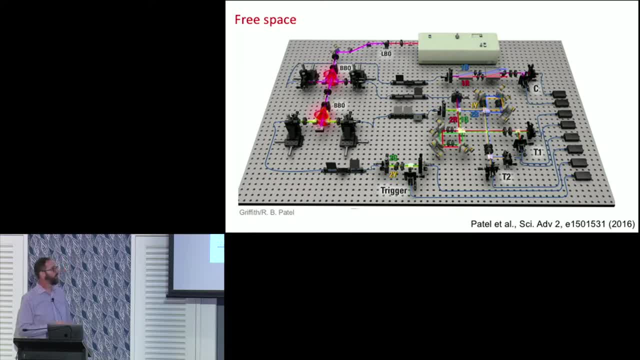 optics quantum computing experiment. okay, it sits on a breadboard in an optical. it sits on a breadboard in an optical. it sits on a breadboard in an optical lab and it's not sort of inherently lab and it's not sort of inherently lab and it's not sort of inherently technologically scalable. why do we do? 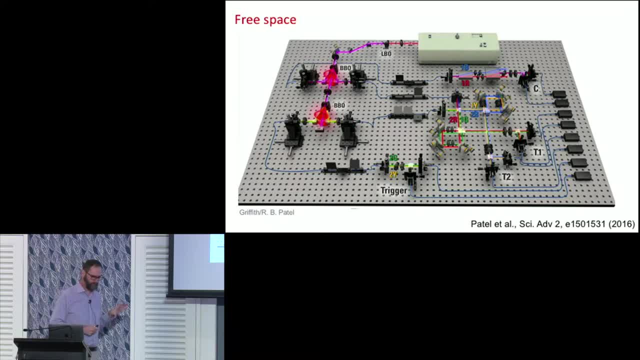 technologically scalable. why do we do technologically scalable? why do we do experiments like this? well, as one of the experiments like this, well, as one of the experiments like this. well, as one of the one of the squeezing community said I, one of the one of the squeezing community said I. 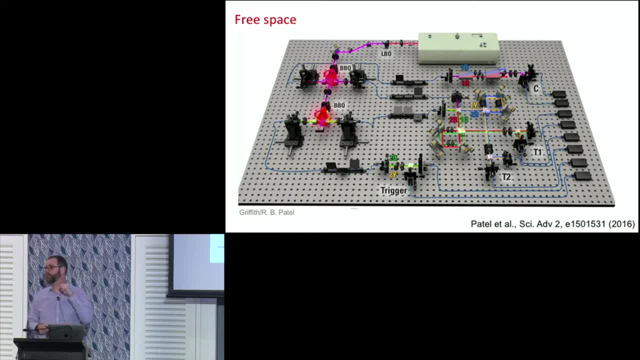 one of the one of the squeezing community said: I think it might have been Roman. think it might have been Roman. think it might have been Roman Schnabel. we do these kinds of experiments, Schnabel. we do these kinds of experiments, Schnabel. we do these kinds of experiments because they produce simply the best. 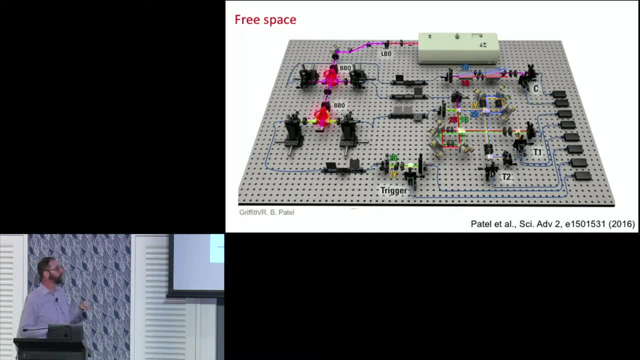 because they produce simply the best, because they produce simply the best fidelity. I mean we're very, very good at fidelity. I mean we're very, very good at fidelity. I mean we're very, very good at doing these and we can do complex doing these, and we can do complex. 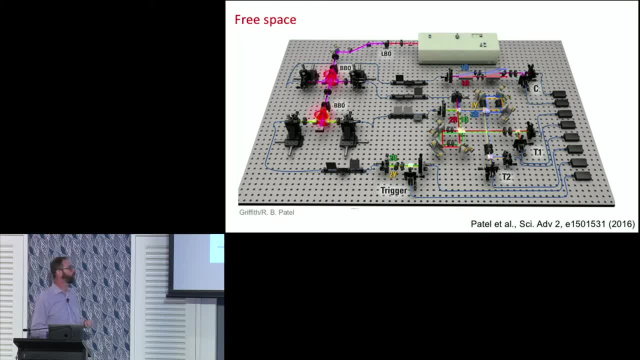 doing these and we can do complex operations. we can learn how to build operations. we can learn how to build operations. we can learn how to build better sources. we can learn how to do better sources. we can learn how to do better sources. we can learn how to do different conceptual techniques. okay, and 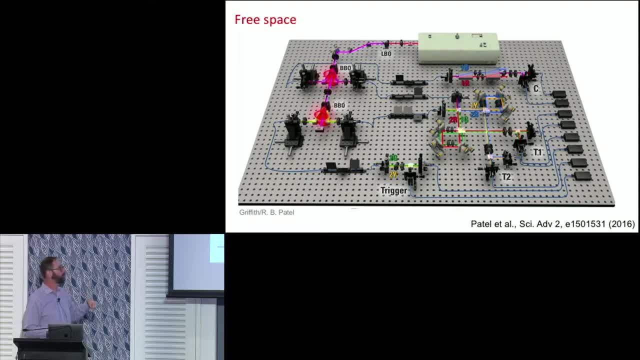 different conceptual techniques. okay, and different conceptual techniques okay. and when it comes to doing things that are, when it comes to doing things that are, when it comes to doing things that are not universal quantum computing, it may be not universal quantum computing. it may be not universal quantum computing. it may be that this kind of platform is a 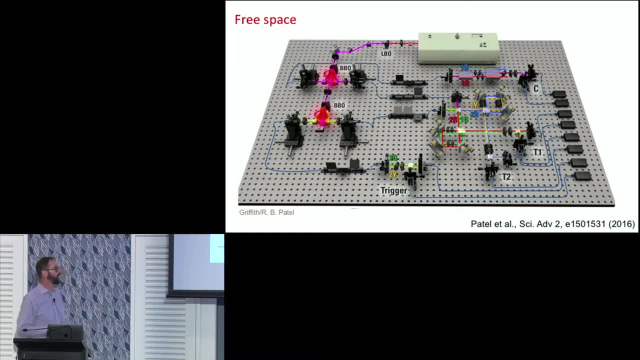 that this kind of platform is a, that this kind of platform is a perfectly good way for doing networking, perfectly good way for doing networking, perfectly good way for doing networking tasks and other things, particularly tasks and other things, particularly tasks and other things, particularly since it can still be considerably. 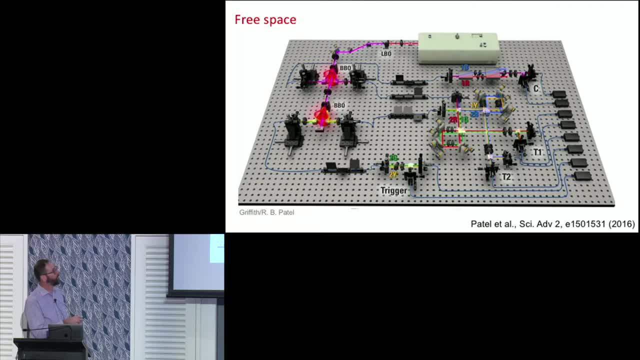 since it can still be considerably, since it can still be considerably miniaturized compared to to what this miniaturized, compared to to what this miniaturized, compared to to what this looks like here, just by way of reference. looks like here, just by way of reference. 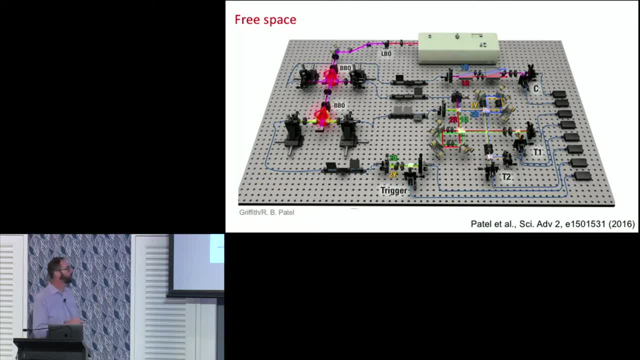 looks like here, just by way of reference. this laser here is. you know, probably I. this laser here is, you know, probably I. this laser here is, you know, probably I don't know what three-quarters of a, don't know what three-quarters of a, don't know what three-quarters of a meter long, or half a meter long, okay, but 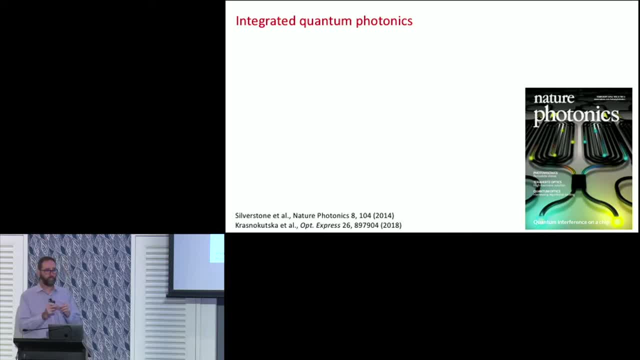 meter long or half a meter long, okay, but meter long or half a meter long, okay, but ultimately one wants to think about, ultimately one wants to think about, ultimately one wants to think about scaling to a miniaturized platform. where scaling to a miniaturized platform, where 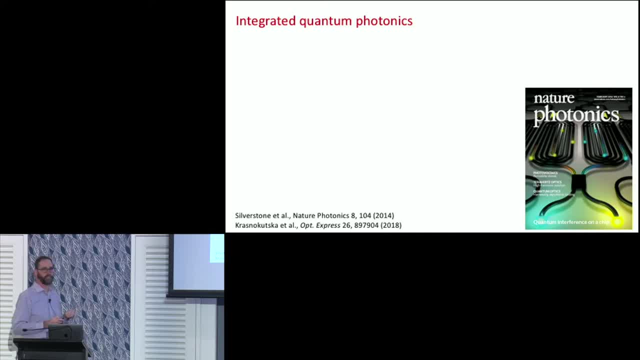 scaling to a miniaturized platform where you can have multiple devices in a very. you can have multiple devices in a very. you can have multiple devices in a very small space, something equivalent to the small space, something equivalent to the small space, something equivalent to the electronics industry. and so this is the 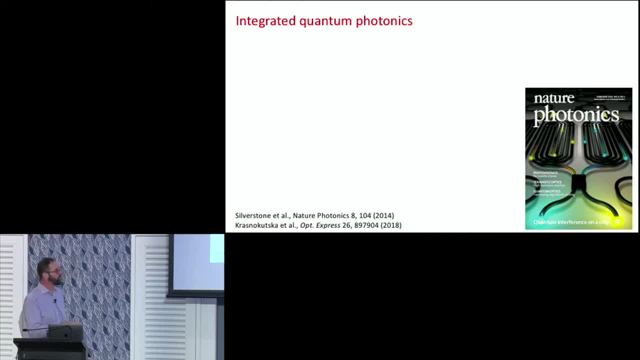 electronics industry, and so this is the electronics industry, and so this is the idea of integrated quantum photonics, idea of integrated quantum photonics, idea of integrated quantum photonics. okay, so devices that something like this- okay, so, devices that something like this: okay, so devices that something like this, not electronic circuits, but optical. 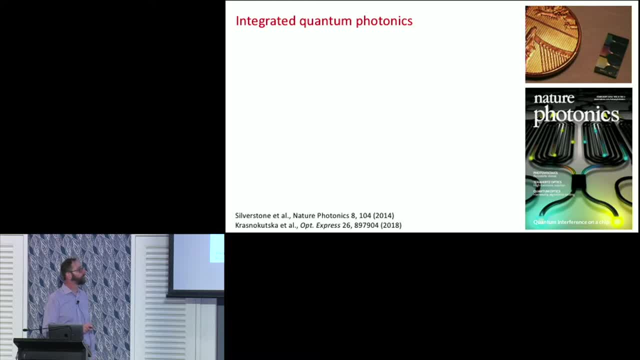 not electronic circuits, but optical. not electronic circuits, but optical circuits on some kind of chip platform, circuits on some kind of chip platform. circuits on some kind of chip platform. okay, so here's an example of a device. okay, so here's an example of a device. okay, so here's an example of a device that Alberto Peruzzo has worked on in the. 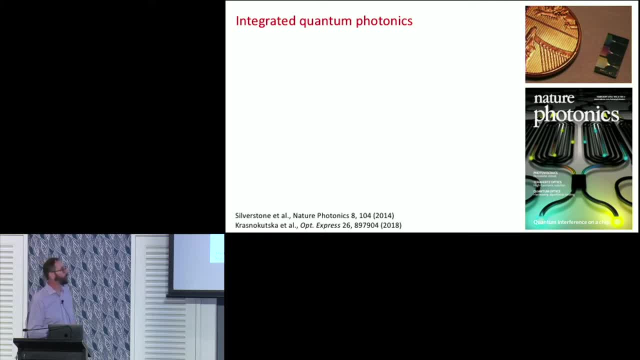 that Alberto Peruzzo has worked on in the, that Alberto Peruzzo has worked on in the past. you can see it compared to the past. you can see it compared to the past. you can see it compared to the size of a small European coin. okay, so, 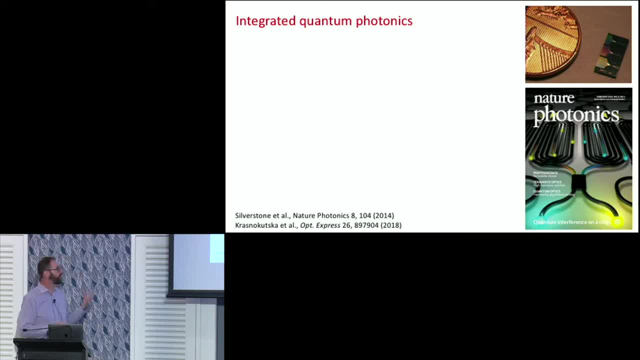 size of a small European coin. okay, so, size of a small European coin. okay, so many, many modes squished into here and many, many modes squished into here and many, many modes squished into here and, in fact, can be even made smaller. now, if in fact can be even made smaller now, if 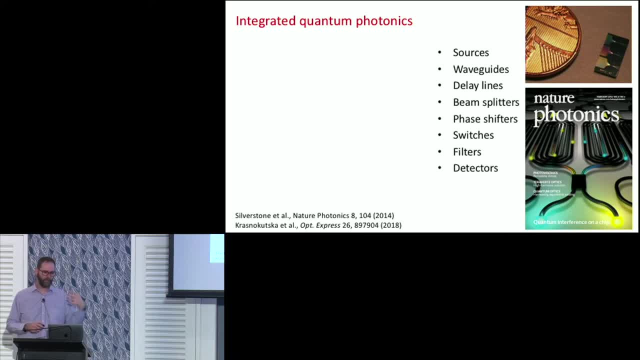 in fact, can be even made smaller. now, if we're going to go to this kind of, we're going to go to this kind of. we're going to go to this kind of platform. what one needs is to have platform. what one needs is to have platform. what one needs is to have sources, waveguides, delay lines, beam. 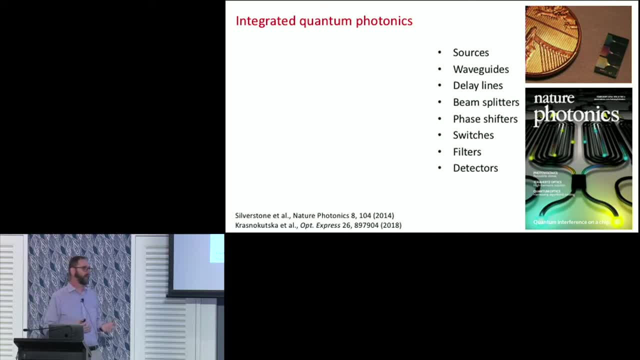 sources: waveguides- delay lines- beam sources- waveguides, delay lines- beam splitters, phase shifters- all the usual splitters, phase shifters- all the usual splitters, phase shifters, all the usual tools detectors- in in this integrated tools detectors. in in this integrated tools detectors in in this integrated platform. okay, so one's looking for a. 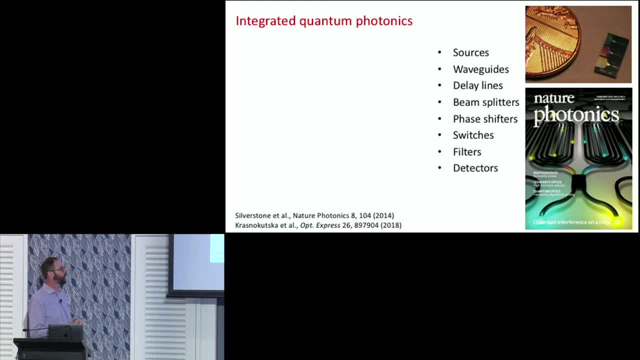 platform. okay, so one's looking for a platform. okay, so one's looking for a material system and a technology system, material system and a technology system, material system and a technology system where all of these things can be put, where all of these things can be put, where all of these things can be put together and realized, you know, in a 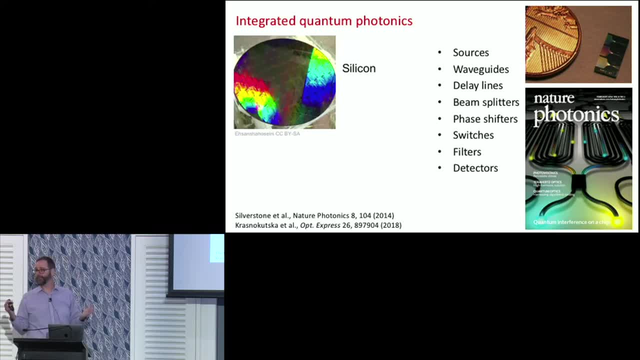 together and realized, you know, in a together and realized, you know, in a practical kind of way. there are many practical kind of way. there are many practical kind of way. there are many different materials that one might different materials that one might different materials that one might choose. but an account of time I'll. 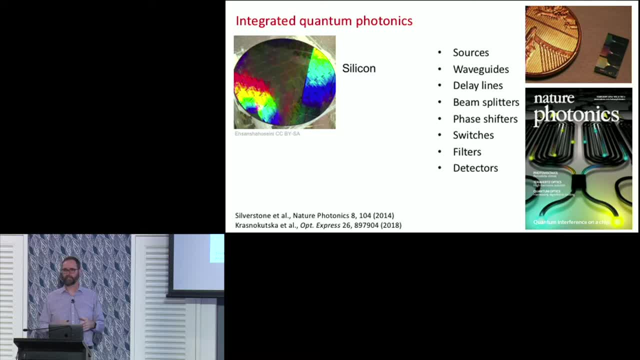 choose, but an account of time, I'll choose. but an account of time, I'll mention. I'll mention two. one is of mention, I'll mention two. one is of mention, I'll mention two. one is, of course, silicon. okay, we've heard from course silicon. okay, we've heard from. 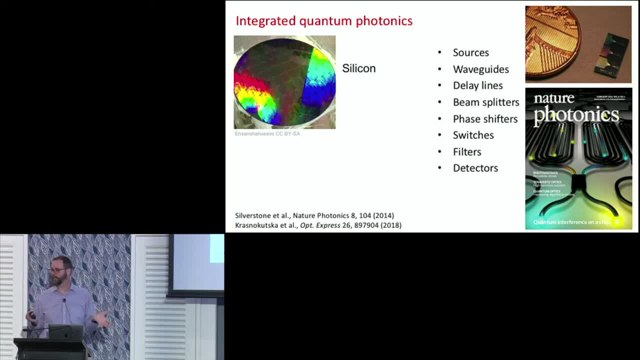 course silicon. okay, we've heard from Andrea that silicon is a technologically Andrea, that silicon is a technologically Andrea, that silicon is a technologically ready platform. it's something that ready platform. it's something that ready platform. it's something that people do processing in already. 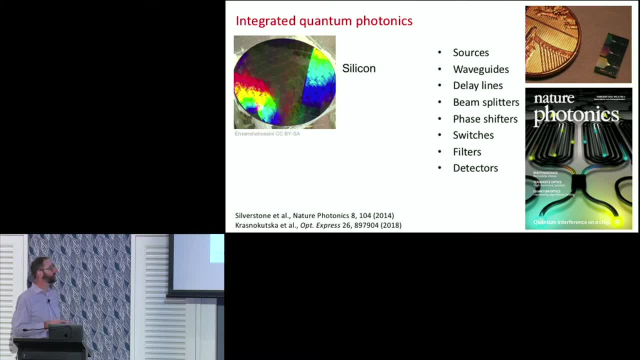 people do processing in already. people do processing in already, including in classical silicon photonics, including in classical silicon photonics, including in classical silicon photonics. and so here's an example of a bunch of, and so here's an example of a bunch of and so here's an example of a bunch of optical circuits on a classical for. 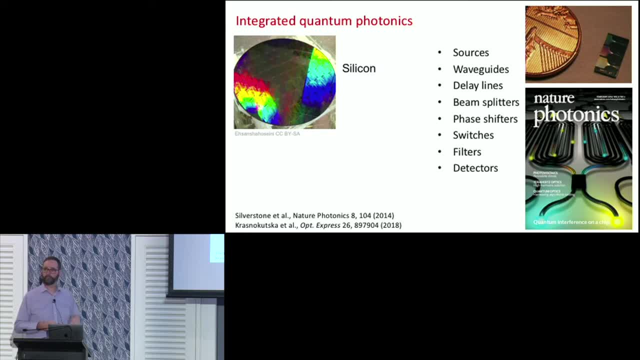 optical circuits on a classical for optical circuits on a classical for classical applications- okay, and one can classical applications okay, and one can classical applications okay, and one can get very high index contrast ratio. get very high index contrast ratio, get very high index contrast ratio between the wave guides and and the 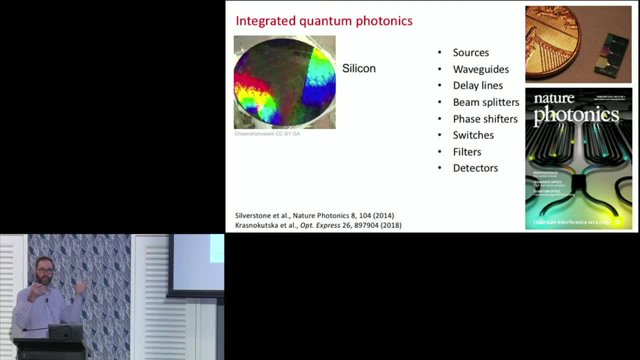 between the wave guides and and the between the wave guides and and the surrounds in silicon, which means that surrounds in silicon, which means that surrounds in silicon, which means that you can pack components in in very, very. you can pack components in in very, very. you can pack components in in very, very high density. but there's another, very high density, but there's another very high density, but there's another very interesting platform and it's the one interesting platform and it's the one interesting platform and it's the one that we're looking at mostly in the, that we're looking at mostly in the. 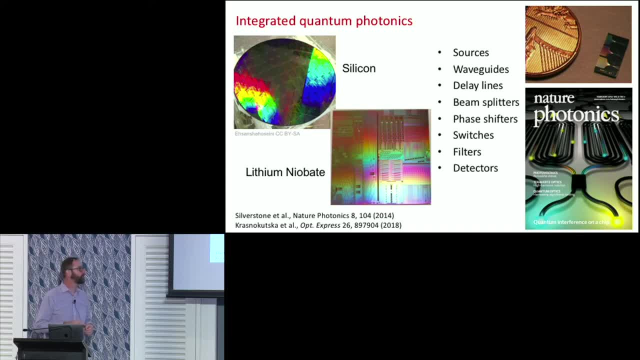 that we're looking at mostly in the center which is lithium niobate: okay. so center which is lithium niobate: okay. so center which is lithium niobate: okay. so lithium niobate is also a really great. lithium niobate is also a really great. 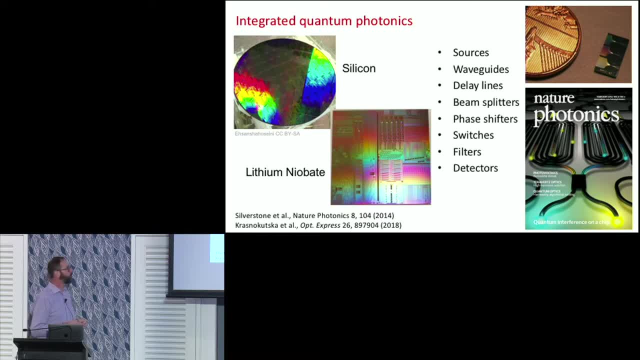 lithium niobate is also a really great technology, and I'll say a little bit technology and I'll say a little bit technology and I'll say a little bit more about that as we go along, okay. so more about that as we go along, okay, so. 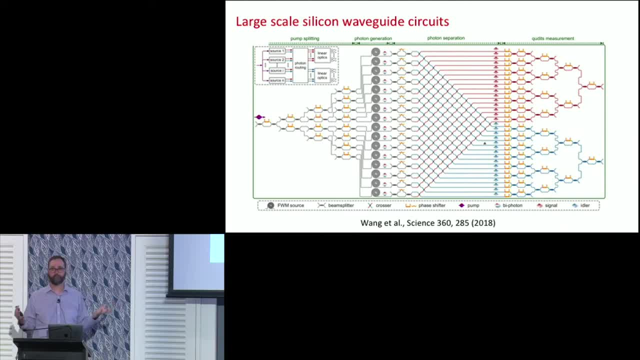 more about that as we go along okay. so there have been some sophisticated. there have been some sophisticated. there have been some sophisticated demonstrations of putting a great many demonstrations of putting a great many demonstrations of putting a great many components onto a silicon chip. this is components onto a silicon chip. this is. 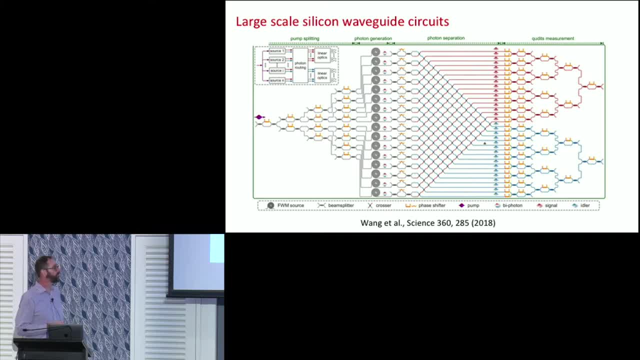 components onto a silicon chip. this is by Bristol, they're a partner of our by Bristol, they're a partner of our by Bristol, they're a partner of our Center and they have sort of many Center and they have sort of many Center and they have sort of many sources, you know, photon generation steps. 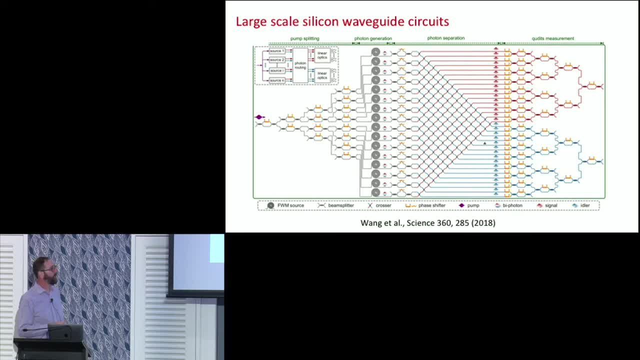 sources: you know photon generation steps. sources: you know photon generation steps, if you will. you know moving the photons, if you will. you know moving the photons, if you will. you know moving the photons around, interfering the photons in around, interfering the photons in around, interfering the photons in different ways, and so on. so chips with 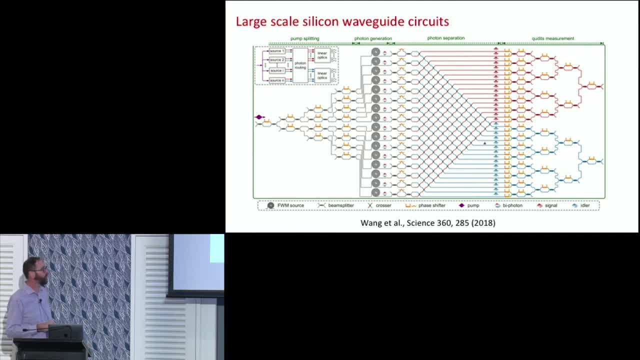 different ways and so on. so chips with different ways and so on. so chips with sort of you know getting to hundreds of sort of you know getting to hundreds of sort of you know getting to hundreds of hundreds of elements on them in a very, hundreds of elements on them in a very. 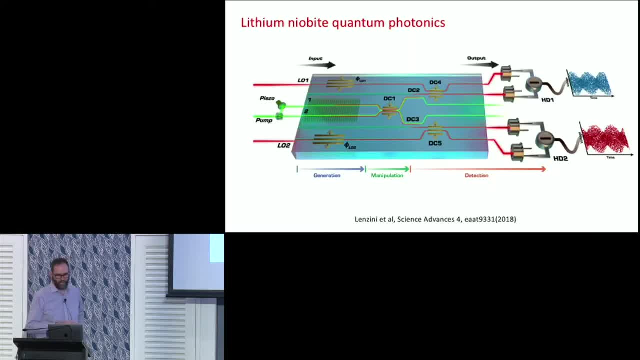 hundreds of elements on them in a very compact kind of way. okay, but we're compact kind of way. okay, but we're compact kind of way. okay, but we're interested in using lithium niobate and interested in using lithium niobate and interested in using lithium niobate and one of the reasons that lithium niobate 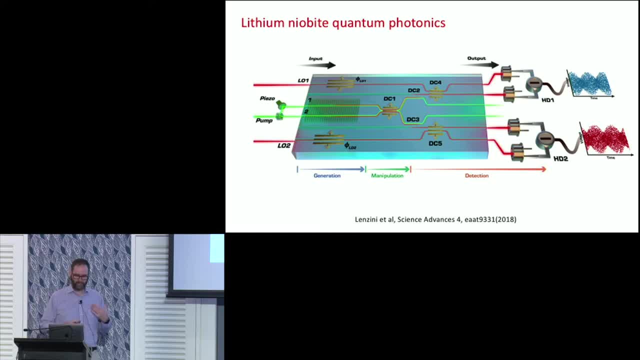 one of the reasons that lithium niobate, one of the reasons that lithium niobate is really really nice- yep, yep is that it is really really nice. yep, yep is that it is really really nice. yep, yep is that it is it enables really beautiful. 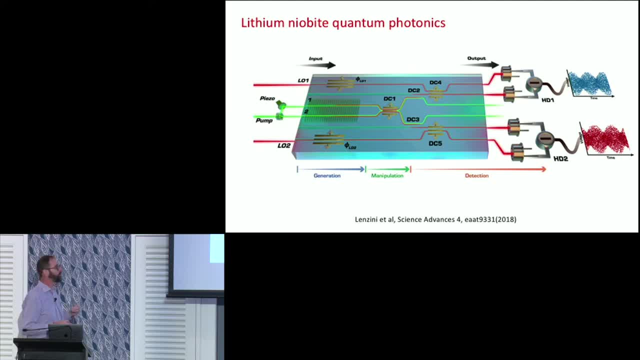 is it enables really beautiful, is it enables really beautiful switching, fast switching, nonlinear switching, nonlinear switching, nonlinear processes in the material and can be made processes in the material and can be made processes in the material and can be made very low loss. okay, here's an example. very low loss. okay, here's an example. 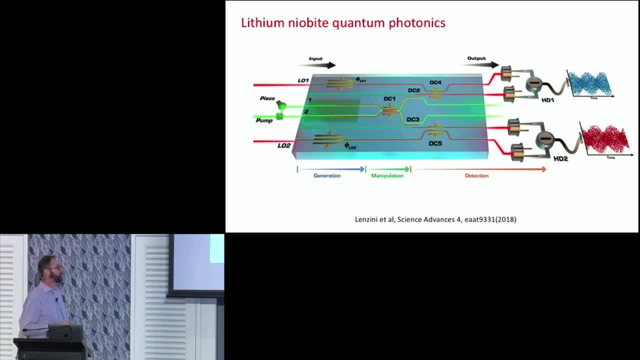 very low loss. okay, here's an example of some work which is a collaboration of some work, which is a collaboration of some work, which is a collaboration between Mirko and the groups at ANU, and between Mirko and the groups at ANU, and between Mirko and the groups at ANU and ADFA. okay, to do generate squeezing on. 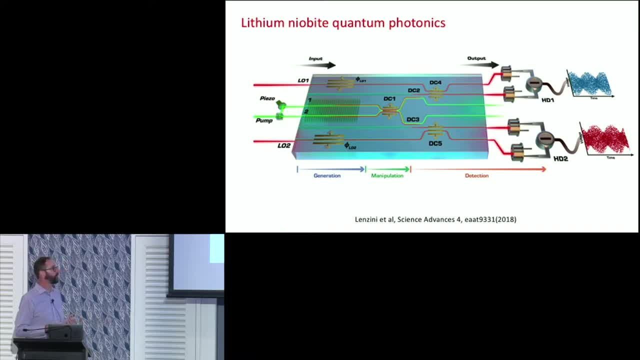 ADFA. okay to do generate squeezing on ADFA. okay to do. generate squeezing on chip and to basically do the homodyne chip and to basically do the homodyne chip and to basically do the homodyne interference part of the experiment here. interference- part of the experiment here. 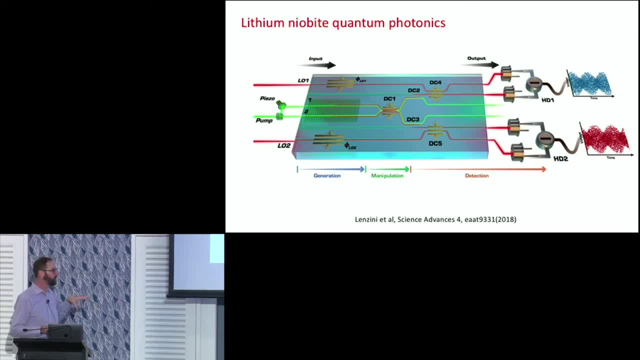 interference part of the experiment here, and to see squeezing on chip which can and to see squeezing on chip which can, and to see squeezing on chip which can then be built in in a pathway towards CV, then be built in in a pathway towards CV, then be built in in a pathway towards CV cluster states. this is done with dopant. 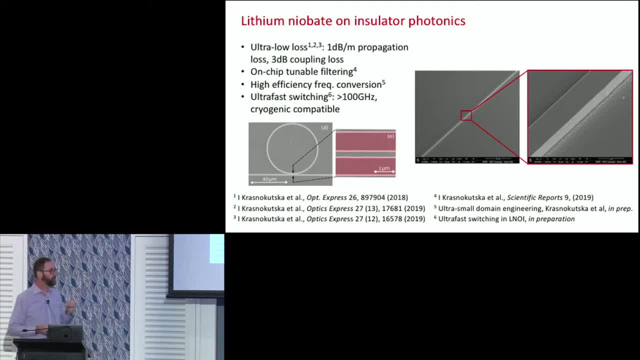 cluster states. this is done with dopant cluster states. this is done with dopant waveguide in silicon but a very low loss waveguide in silicon, but a very low loss waveguide in silicon, but a very low loss. technology is the technology being. technology is the technology being. 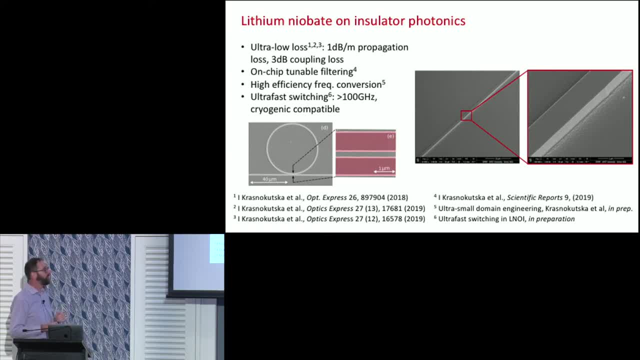 technology is the technology being pursued by Alberto Peruzzo at RMIT with pursued by Alberto Peruzzo at RMIT with pursued by Alberto Peruzzo at RMIT with making ridge waveguides. so this lithium making ridge waveguides. so this lithium. 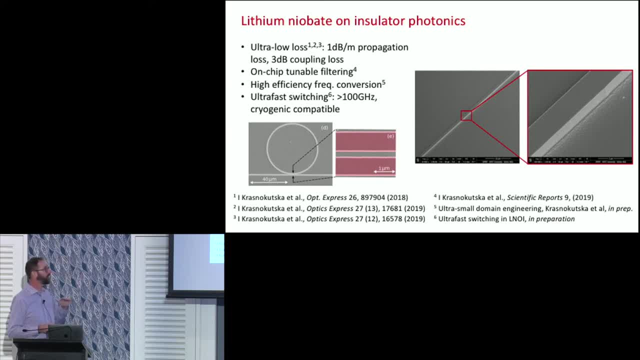 making ridge waveguides. so this lithium niobate is is sort of deposited on top niobate. is is sort of deposited on top niobate. is is sort of deposited on top of a silica layer on top of silicon, so it of a silica layer on top of silicon, so it. 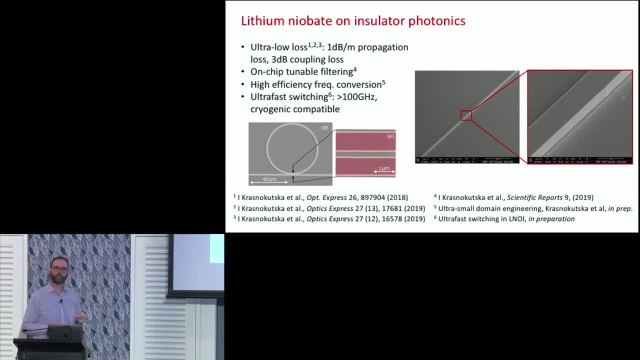 of a silica layer on top of silicon so it can be integrated with silicon, can be integrated with silicon, can be integrated with silicon technologies. but it can be made technologies. but it can be made technologies. but it can be made. incredibly low loss with incredibly fast. incredibly low loss with incredibly fast. 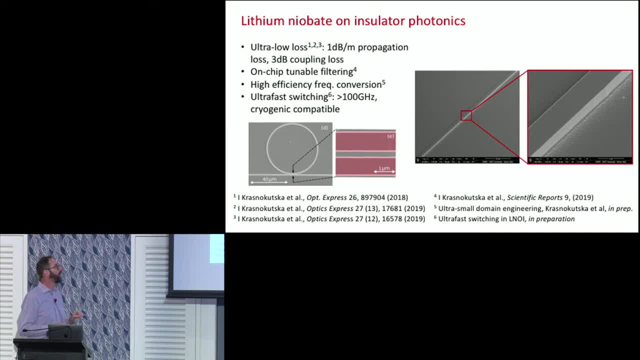 incredibly low loss with incredibly fast switching. it can be cryogenically switching. it can be cryogenically switching. it can be cryogenically compatible, and one can make as as compatible, and one can make as as compatible, and one can make as, as Alberto is doing, making ring resonators. 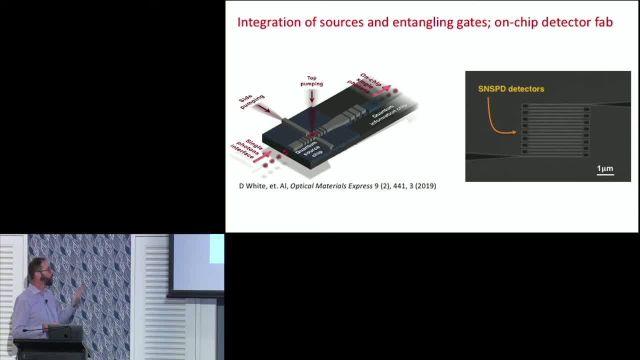 Alberto is doing making ring resonators. Alberto is doing making ring resonators. really beautiful sidewall etching. come, really beautiful sidewall etching. come really beautiful sidewall etching. come along, can do things like design along. can do things like design along. can do things like design structures for integrating quantum dots. 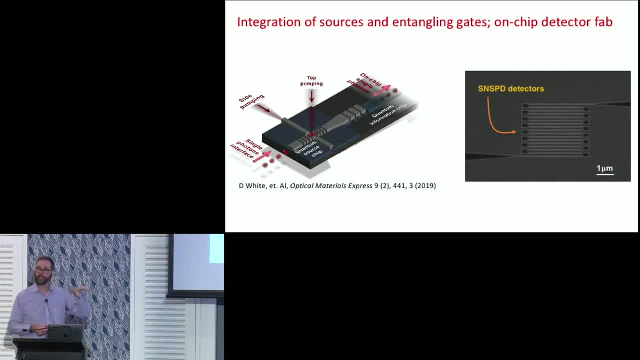 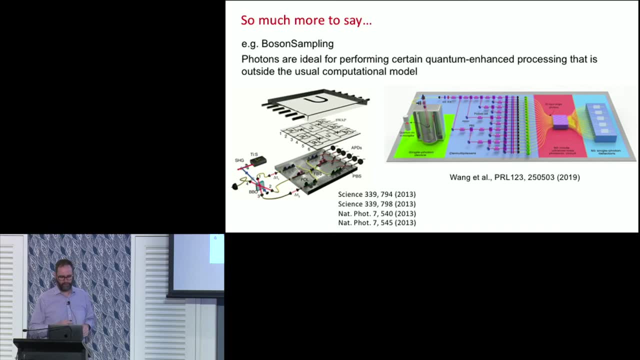 structures for integrating quantum dots. structures for integrating quantum dots onto chips for writing detectors, on to onto chips for writing detectors, on to onto chips for writing detectors. on to onto the chips as well. okay, so there's onto the chips as well. okay, so there's onto the chips as well. okay, so there's so much more to say about the optic. 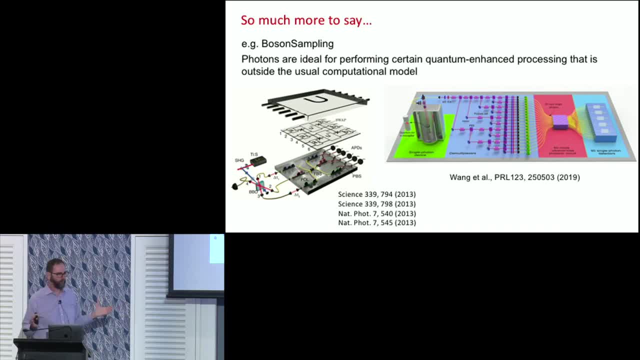 so much more to say about the optic, so much more to say about the optic space. I haven't even talked about space. I haven't even talked about space. I haven't even talked about sampling problems. photons are ideal for sampling problems. photons are ideal for sampling problems. photons are ideal for some non-universal kinds of tasks. 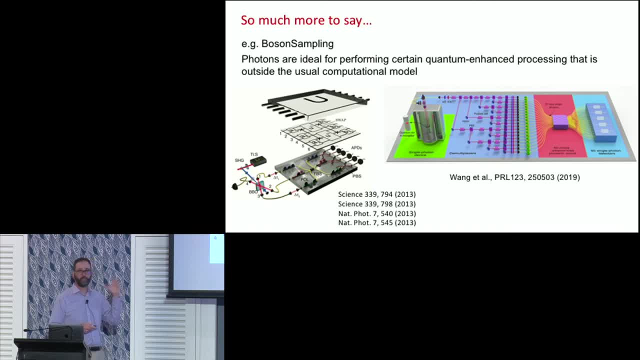 some non-universal kinds of tasks, some non-universal kinds of tasks because of their bosonic nature and because of their bosonic nature and because of their bosonic nature, and there are efforts within and outside the. there are efforts within and outside the, there are efforts within and outside the center to that. but let me conclude by center to that. but let me conclude by center to that. but let me conclude by just reminding you that one of the just reminding you that, one of the just reminding you that one of the reasons that we're interested in optics, reasons that we're interested in optics, 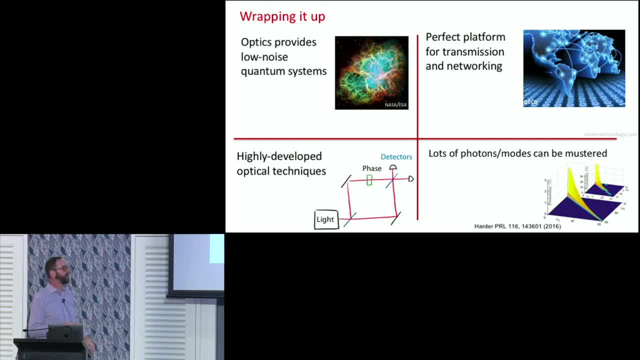 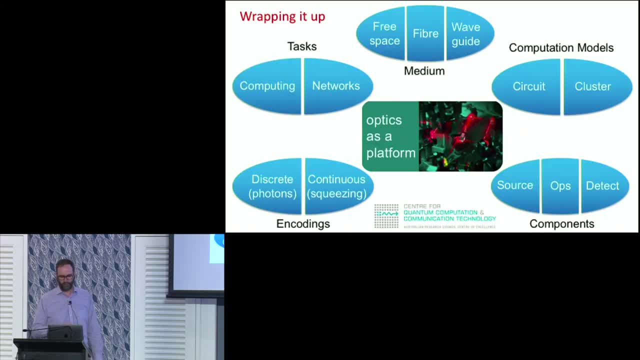 reasons that we're interested in optics is because of these. different is because of these. different is because of these different advantages: interacting networks with advantages. interacting networks with advantages. interacting networks with computing devices: low noise. the ability- computing devices, low noise. the ability- computing devices: low noise. the ability to muster many, many photons. and we've 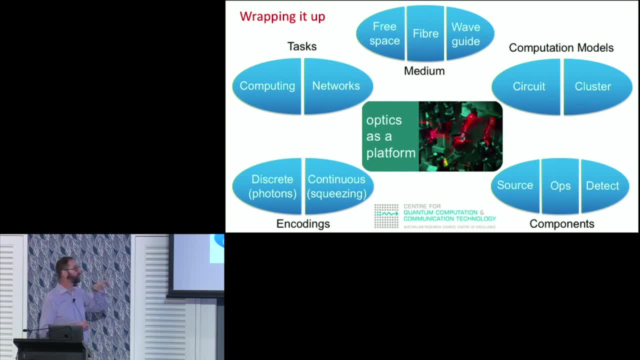 to muster many, many photons, and we've to muster many, many photons, and we've talked about how that optics plays out, talked about how that optics plays out, talked about how that optics plays out with all of these different tasks, and so, with all of these different tasks, and so 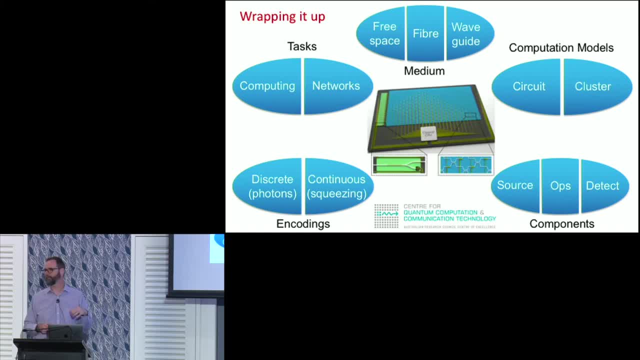 with all of these different tasks, and so it gives us the idea of optics as a. it gives us the idea of optics as a. it gives us the idea of optics as a platform, perhaps an integrated platform platform. perhaps an integrated platform platform, perhaps an integrated platform in which we can have sources, operations. 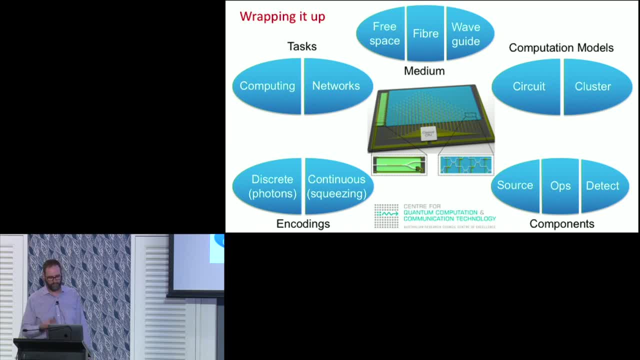 in which we can have sources, operations, in which we can have sources, operations and detectors for large-scale quantum and detectors for large-scale quantum and detectors for large-scale quantum computing and other quantum tasks. thank, computing and other quantum tasks. thank computing and other quantum tasks. thank you.